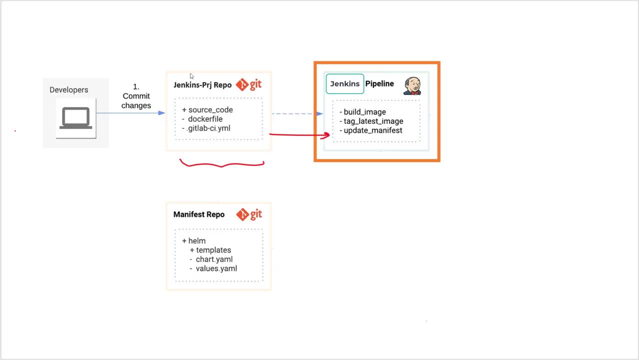 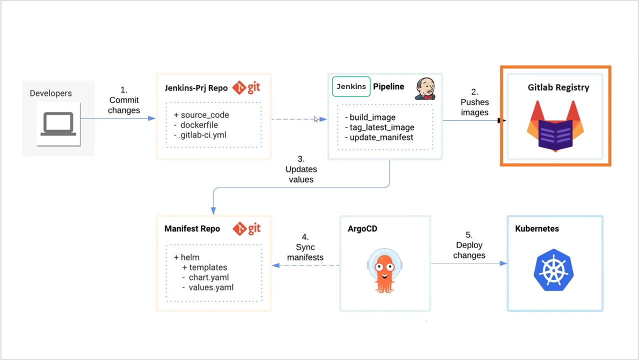 to GitLab server and we'll use webhook on GitLab repository to trigger build jobs on Jenkins server And after we will see the build image will be pushed on GitLab registry and the same time will update manifest or helm charts on manifest repo and automatically will be deployed by Argo CD. 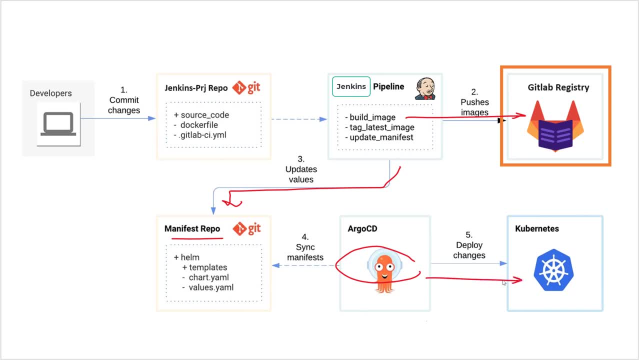 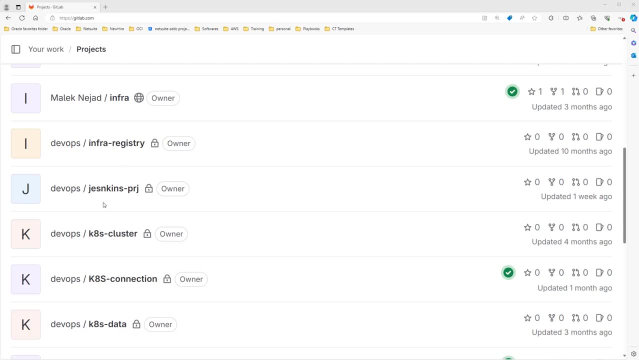 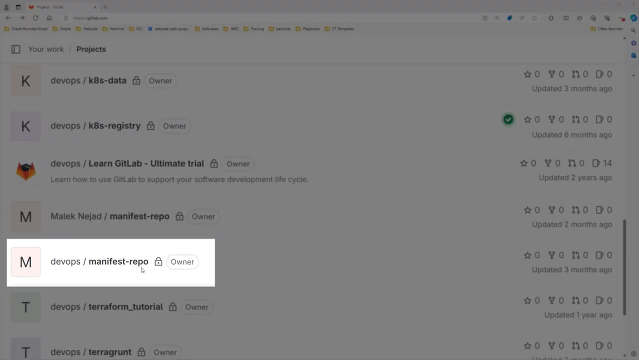 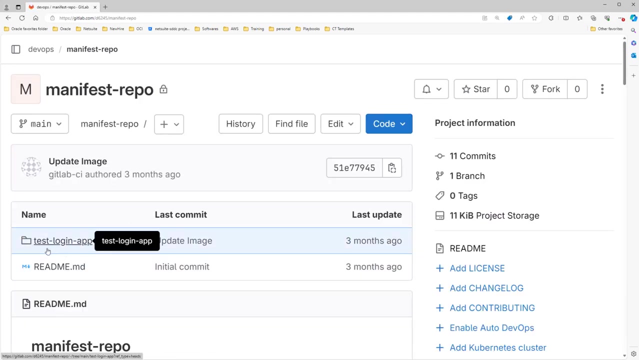 on Kubernetes cluster. Let's start. Here are my repositories on GitLab. Look here: this is Jenkins dash PRJ and the other one Manifest repo. Also, I added my files here. You see, this is my helm chart, If you want to know. 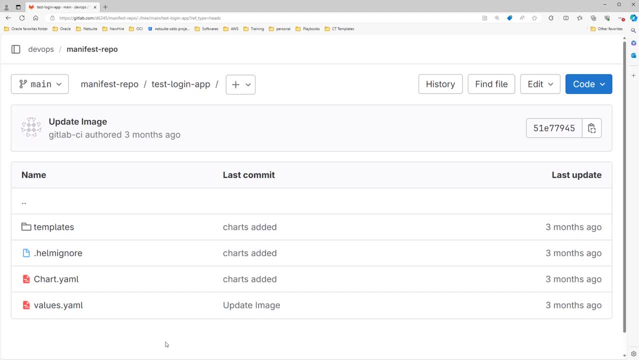 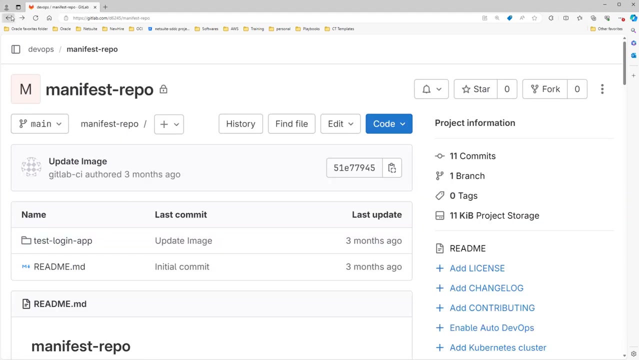 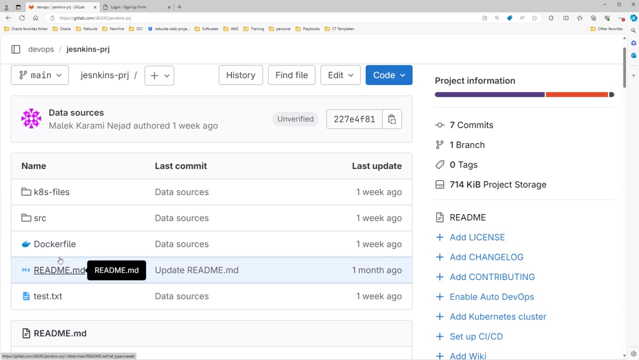 how can create chart for this project? you can check my other video about helm that I have pinned the link of that above of this video. Let's see the other video about this project. Let's see the other repository, Jenkins project. Here you will see all the file related to my project, If I go. 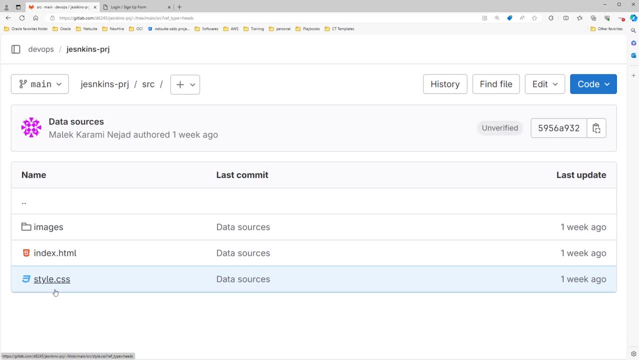 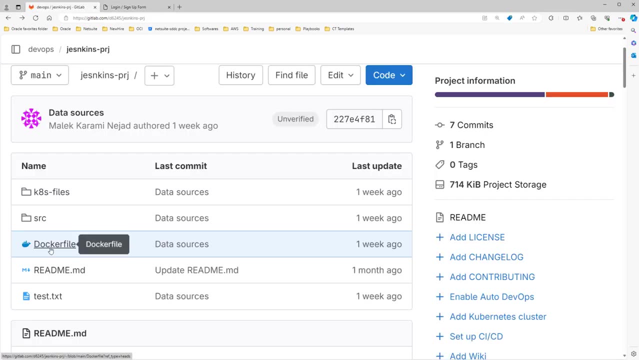 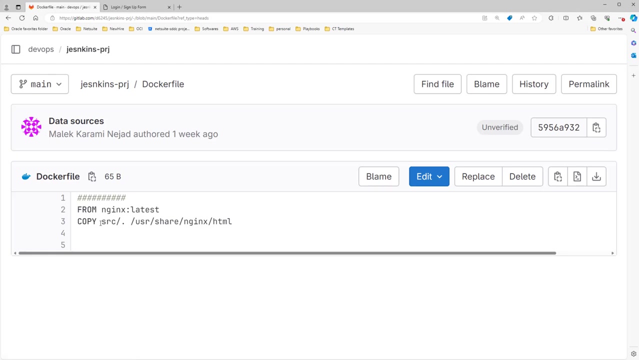 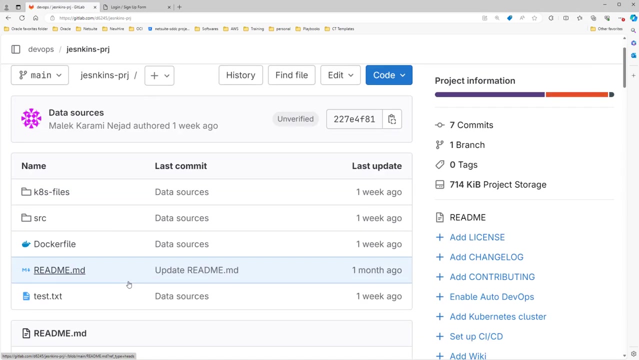 here you will see HTML file with CSS code. It will be a login page and a sign up one. Here is the Docker file. By this Docker file we can create an image from this Source file. This one just temporary here. No, need it, Only the file that we needed here. 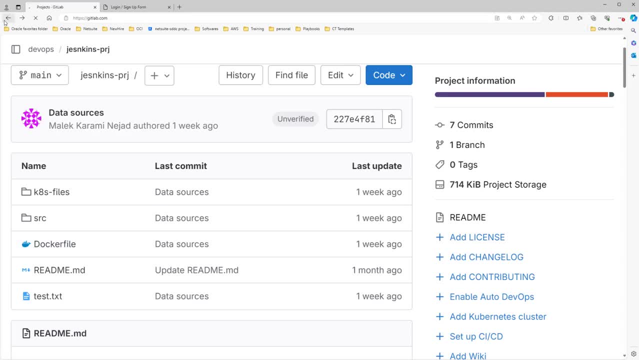 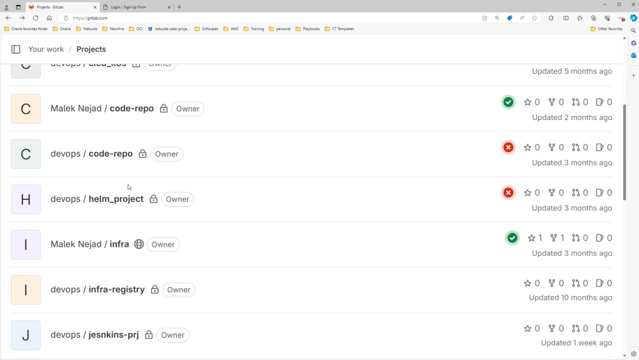 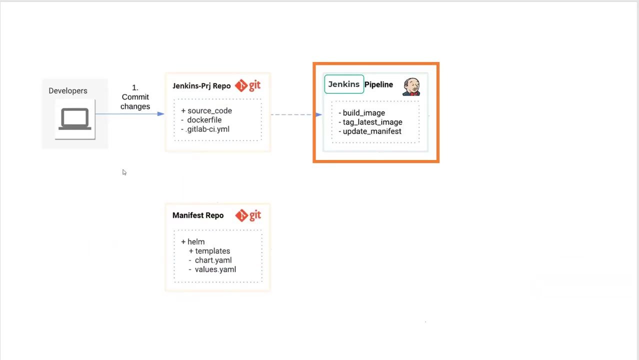 the source and the Docker file. So we have all repositories And in the first step, how this Jenkins dash PRJ repository that has my project data can communicate with Jenkins server. We want to know in the first step when we push an update on Jenkins dash PRJ repo, it should 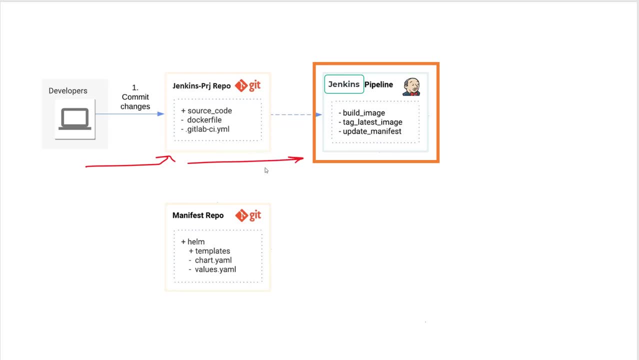 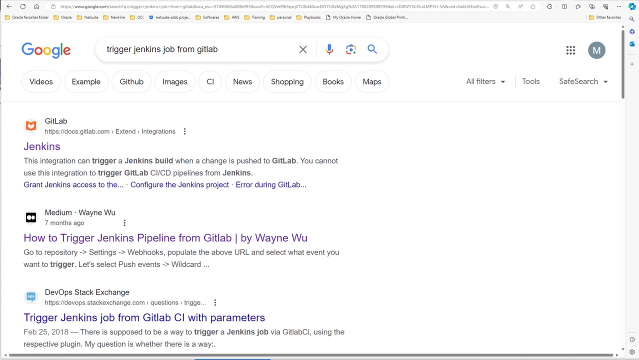 trigger Jenkins server and make a build image from source data and then push it on GitLab registry. How this repository can trigger Jenkins to build an image, Let's talk about it. For. trigger Jenkins job from GitLab. just type this title in Google from the result: 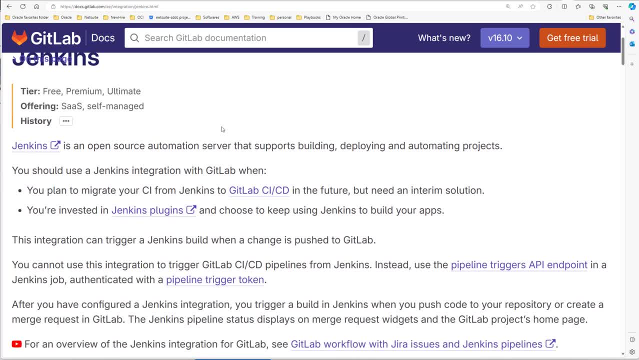 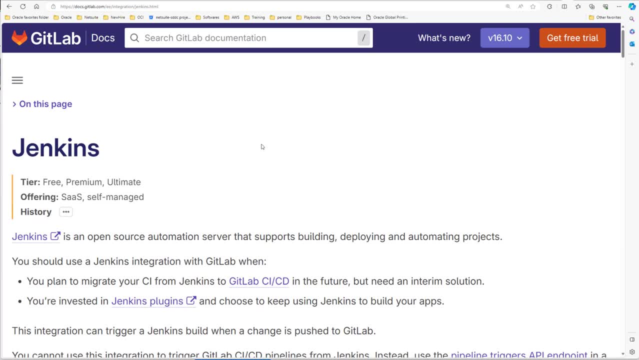 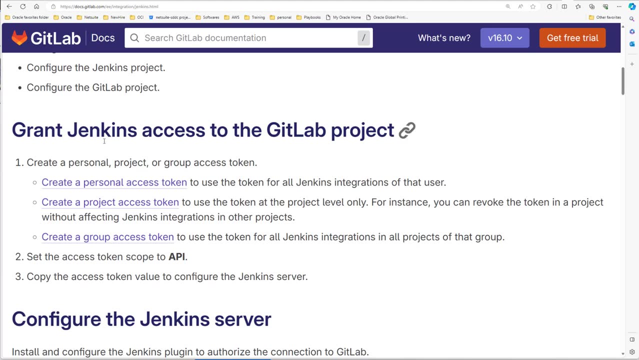 click on this one And here is the official website of GitLab. You can also see it is a complete document from GitLab. So going down it is written here: Grant Jenkins, access to the GitLab project. So for this one. 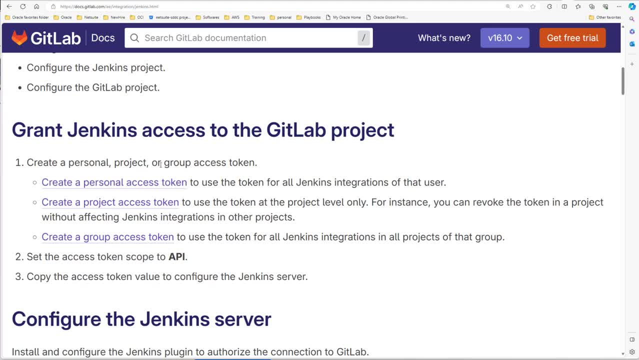 you have to create a personal, project or group access token. Just you need a token to let Jenkins have access to your project on GitLab. So when you go down in the build image right here, then it will be DRIVE04, this is the website where you'll see photo image on the gitlab iscamp and this e 서�必返. So when you click siitä and use the traditionally written function copy, I'm going to washed together each one here If I take the 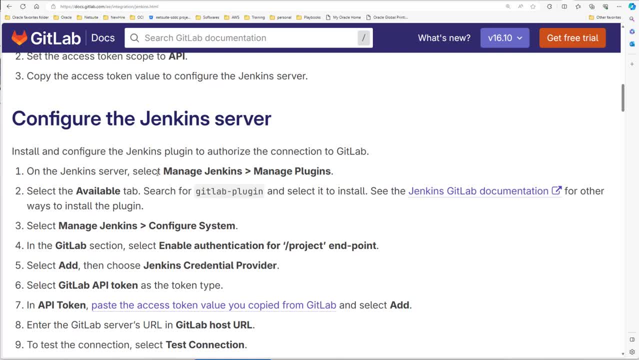 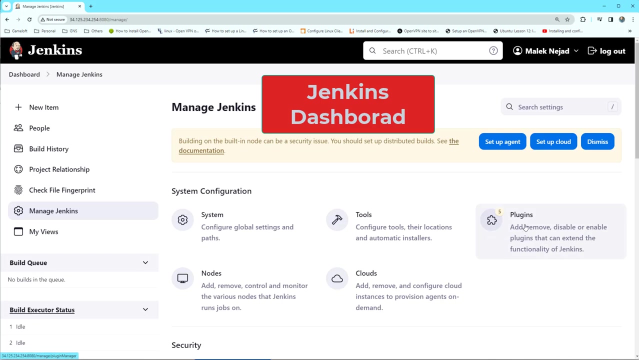 down here all the steps you need to configure. so configure the jenkins server. install and configure the jenkins plugin to authorize the connection to gitlab. in jenkins server: select manage jenkins manage plugin and in available tab search for this one. let's copy this one going to git lab: in gitlab dashboard, manage jenkins, click on plugins. then going to: 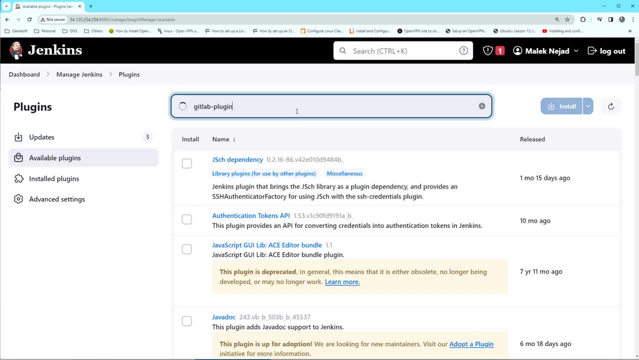 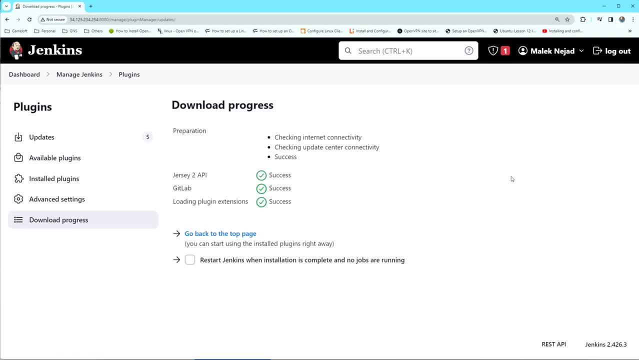 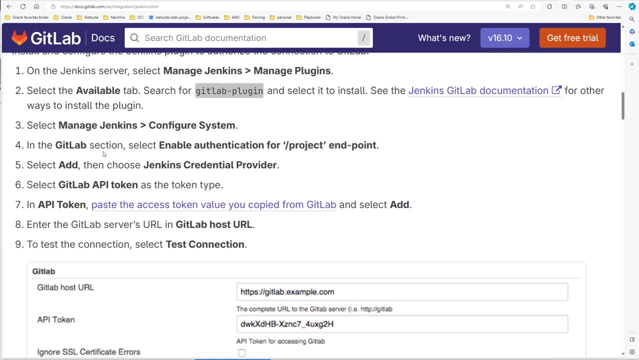 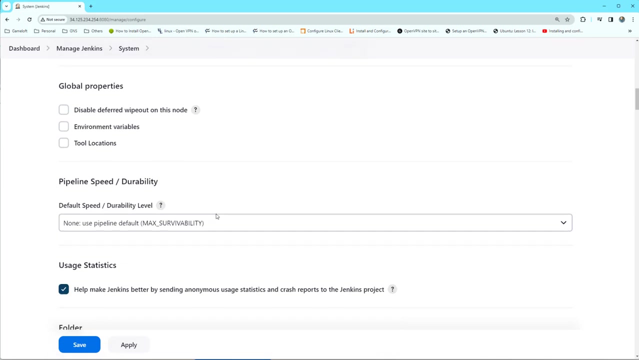 available plugins and search for this one, select it and init all. okay, it's done. let's back to gitlab documentation again. in manage jenkins configure system, in gitlab section, select enable authentication for a slash project endpoint. let's back to jenkins dashboard, manage jenkins system, going down and find gitlab. okay, by default. 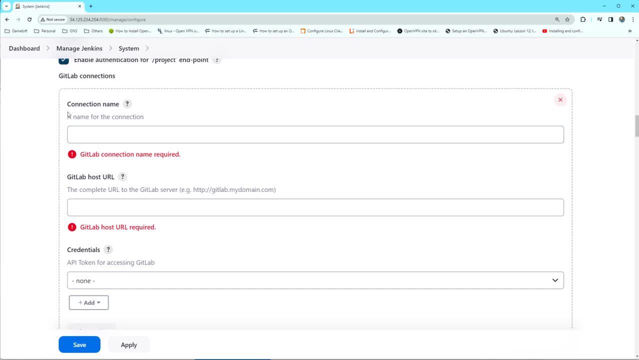 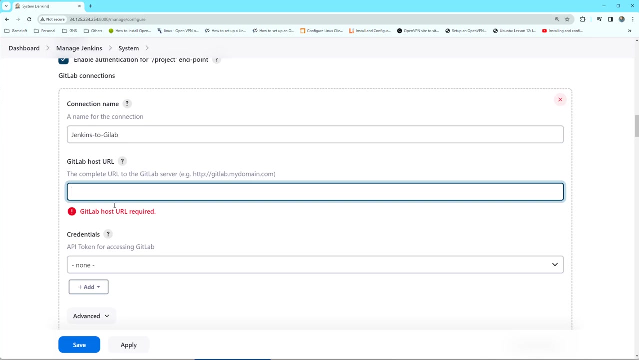 it is enabled. so we need to define a connection name. just type like this, for example, jenkins to gitlab, and here we need to copy gitlab host url. if you are using your local gitlab server, you have to paste the correct ip address or the url of that one here. or if you are using the public gitlab, 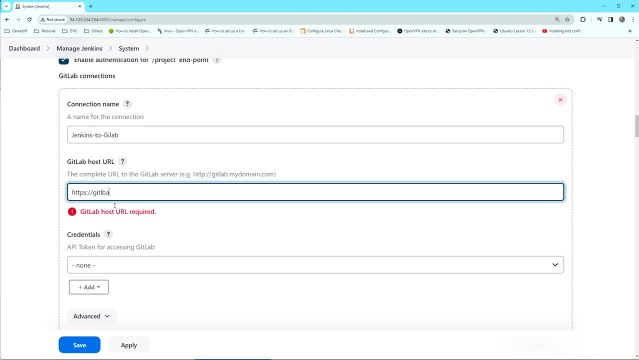 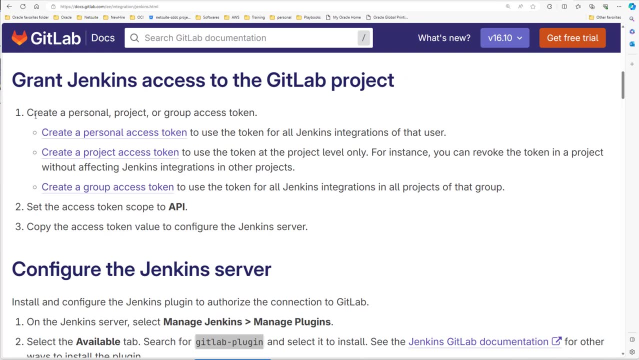 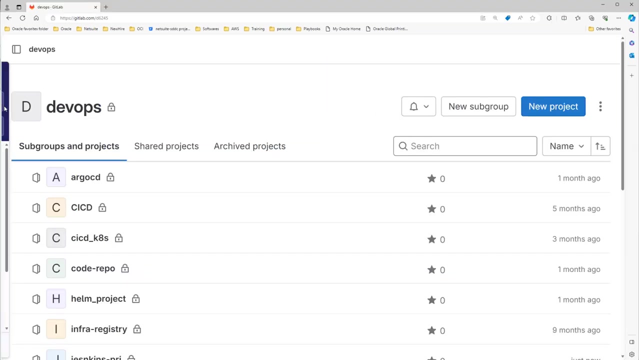 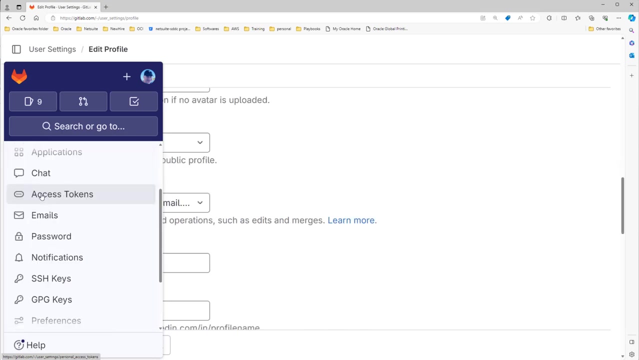 just type https- gitlabcom. now arrive to credential section. as it is written here, you need to create access token on gitlab project in gitlab. from the left side, click on icon and edit profile. now, from the left side, click on access token and here let's to create a personal. 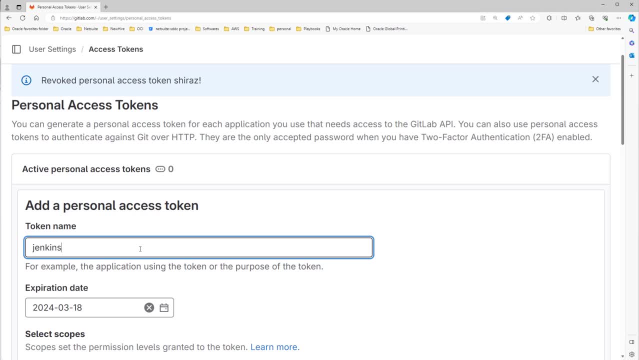 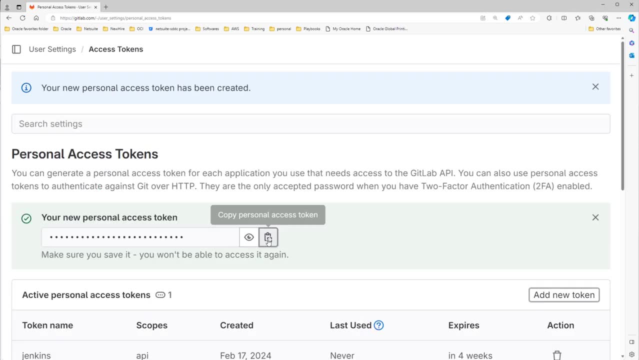 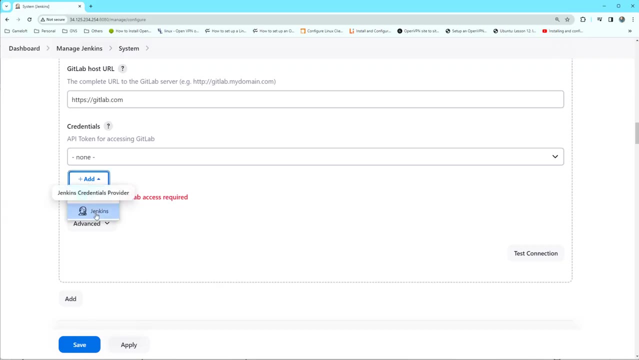 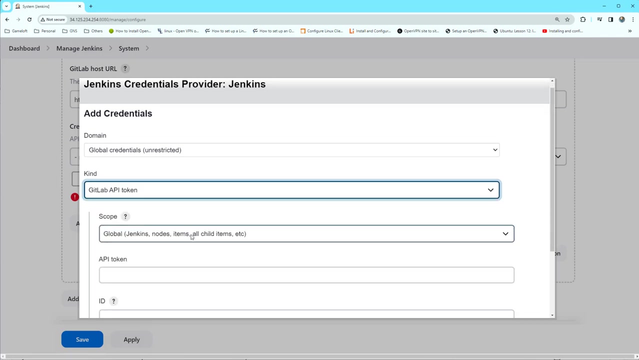 token token name jenkins and click on api and create personal access token. let's copy the token in a safe place at first. back to jenkins dashboard and let's add a credential: jenkins. from kind section, let's select gitlab api token, going down and paste the token here. give it an id in id, just i. 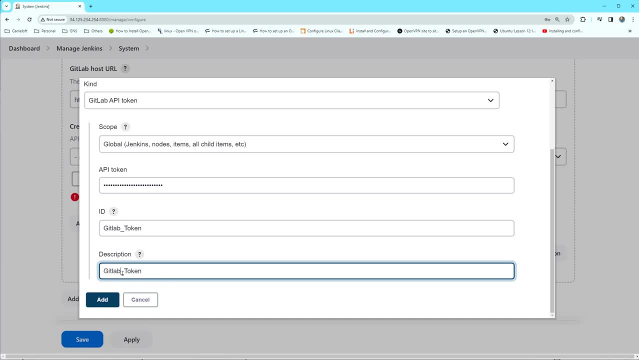 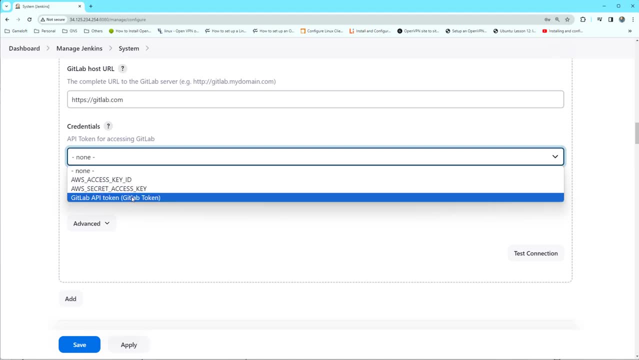 type like this one and the same in description and add so from this box, open it and select gitlab api token and let's click on test connection. you see success and it means your jenkins server at the moment connected to your gitlab server. let's save. let's back to gitlab documentation. so 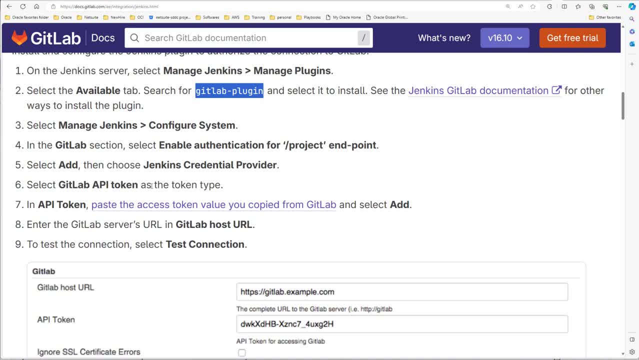 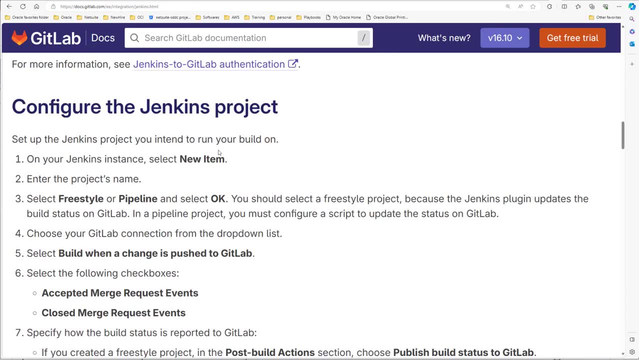 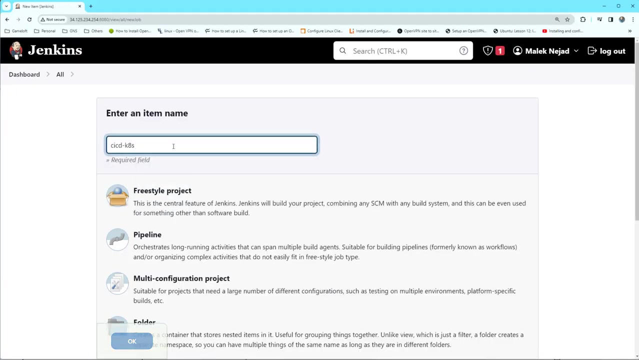 as you see, create and select that api token and also, with the test connection going down. and here in next section you see, configure the jenkins project. so let's go into the jenkins and create a project and configure that based on this document. new item: give it a name, for example: 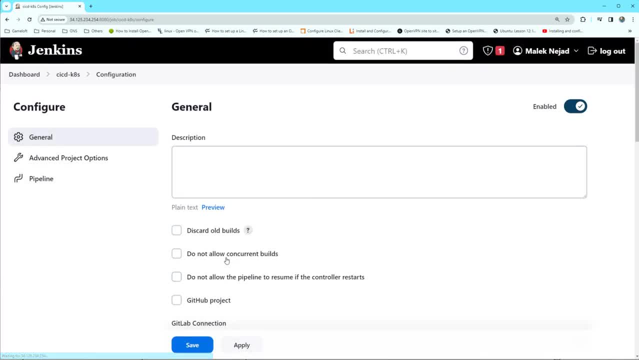 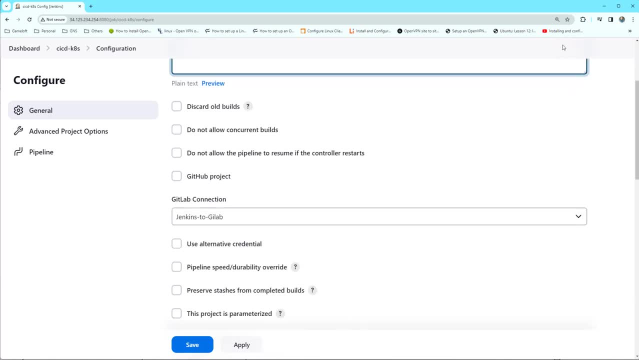 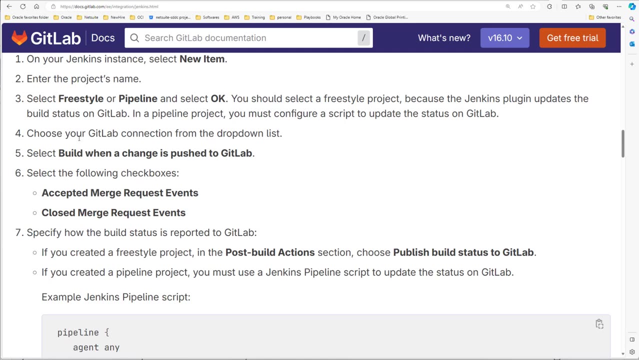 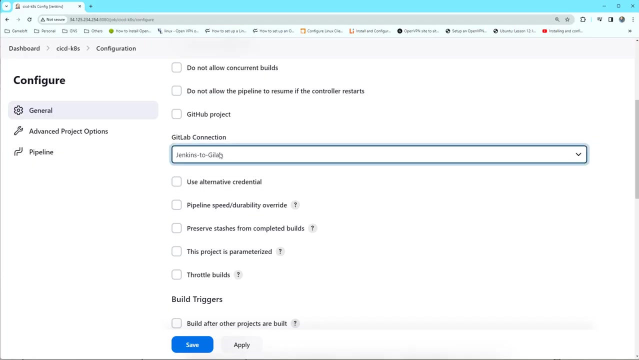 this one. select pipeline: okay, and you will go here. so let's give it and description. so let's back to documentation again. select freestyle or pipeline that we selected at the moment. pipeline: so choose your gitlab connection from drop down list back to jenkins here, gitlab connection, you see. 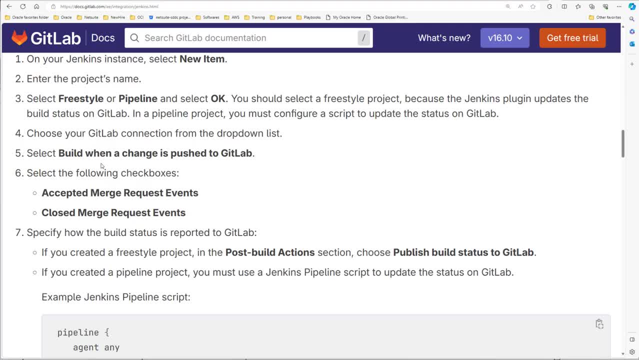 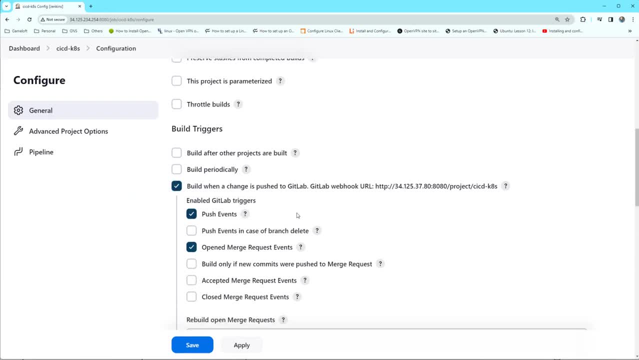 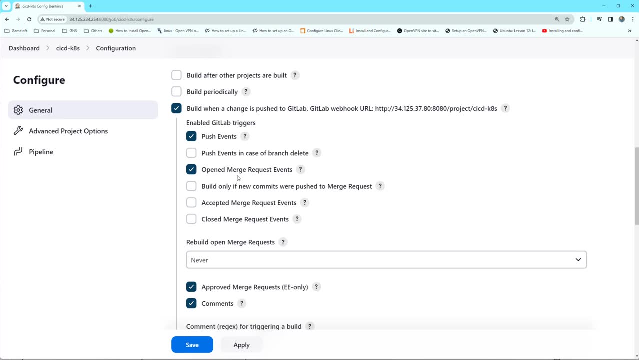 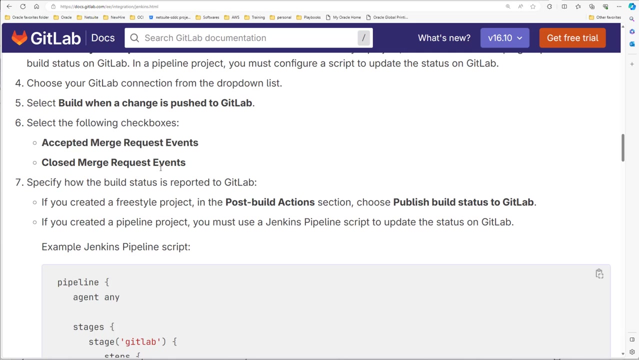 okay, we selected that and in continue select: build when a change is pushed to gitlab. build when changes push to gitlab. okay, so when a push is happened or when a pr is requested or a pr open, accept, accept merge request and close merge request. okay, and also accept merge request event. 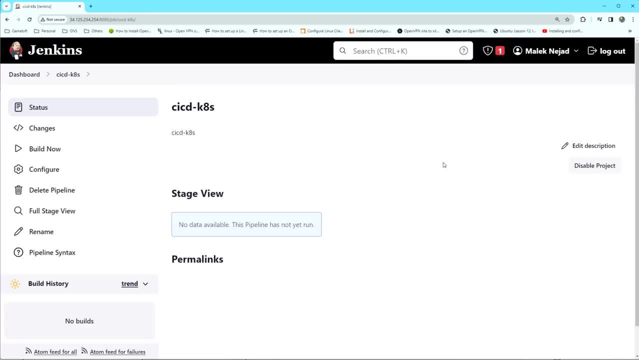 and this one. okay, so let's save it. this section is also done. let's going down. we don't need this one at the moment. let's save it. so let's save it. let's save it. we don't need this one at the moment. let's. 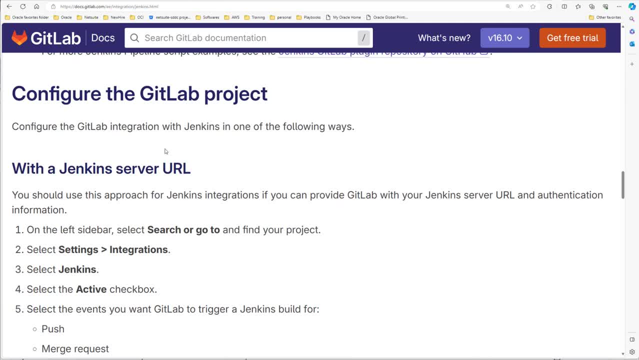 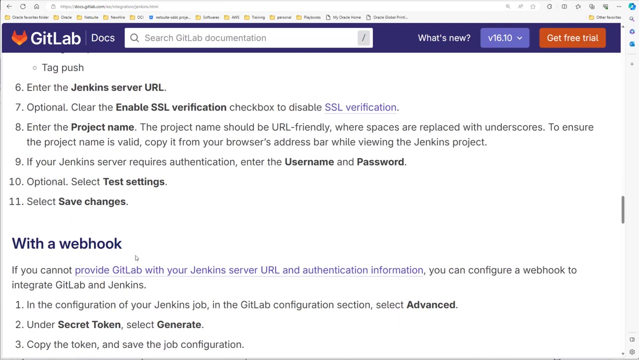 going down. now we want to see how we can trigger the jobs on jenkins server, as you see here, configure the gitlab integration with jenkins in one of the following ways. there are two ways, using the first one with the jenkins server url and the second one with a web hook. here i prefer 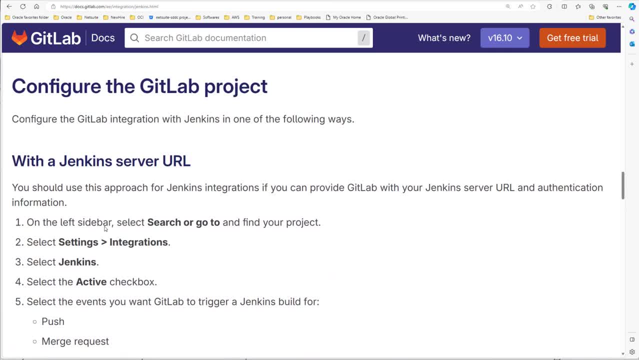 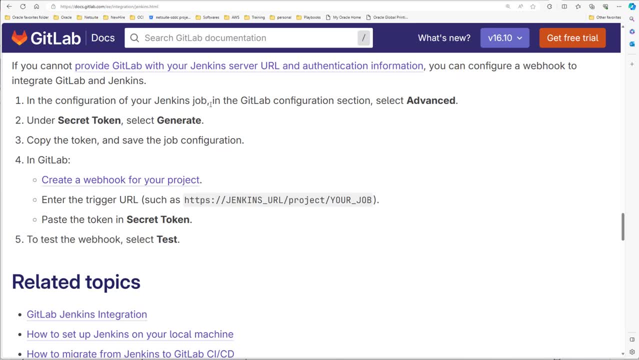 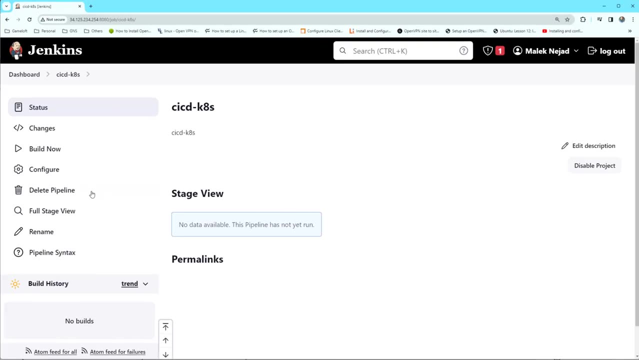 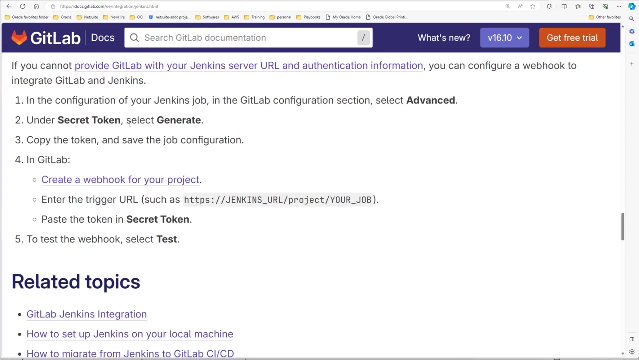 to use the second one also. you can test with the first one. so using with the webhook. so in configuration of your jenkins jobs, in gitlab configuration, select advance. okay, let's back to dashboard configure. let's going down, click on advance under secret token, select generate. 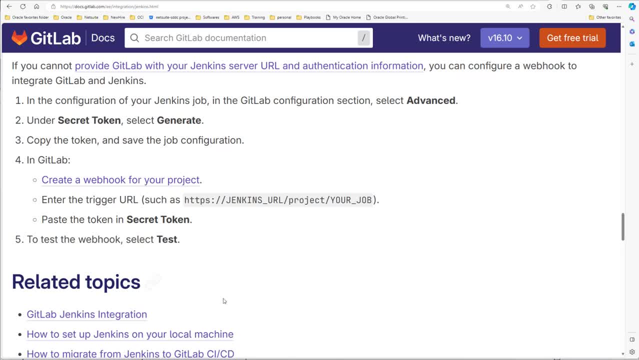 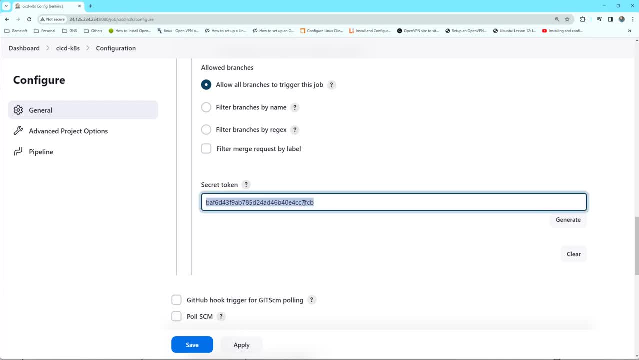 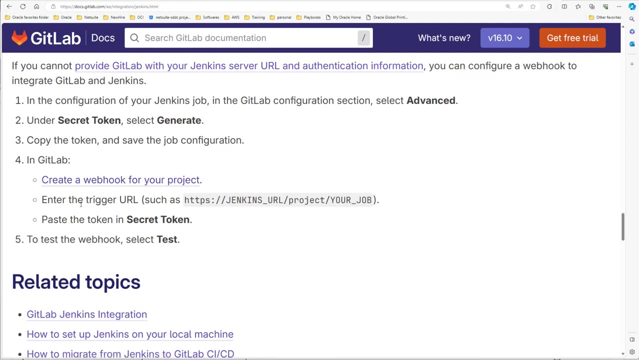 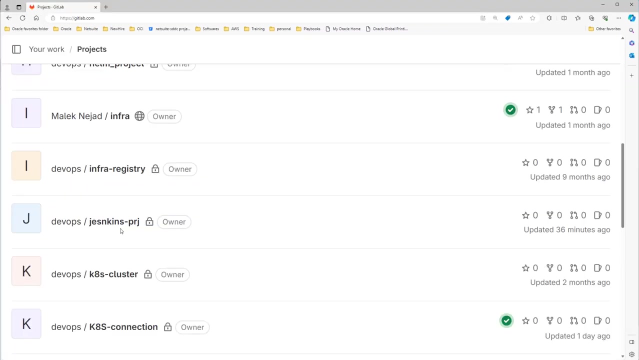 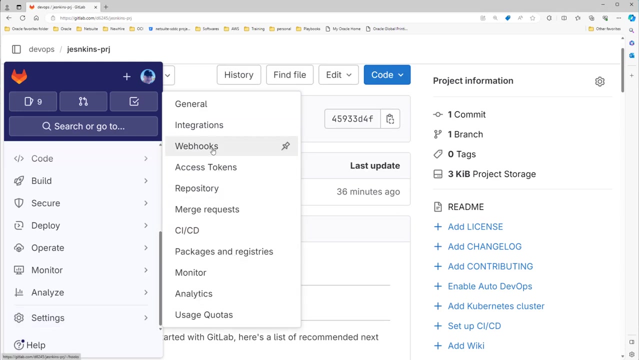 copy the token and save the job configuration. okay, let's here going down, generate a token, copy this one and save it in gitlab. create a web hook for your project, enter the trigger url and paste the token. okay, so let's go into gitlab, select the repo: okay, from the left side, going to setting, and click on web hook. 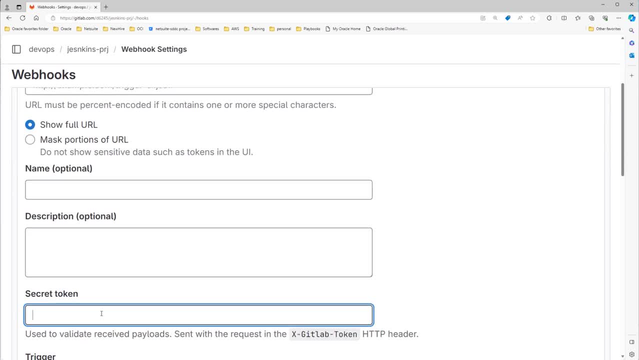 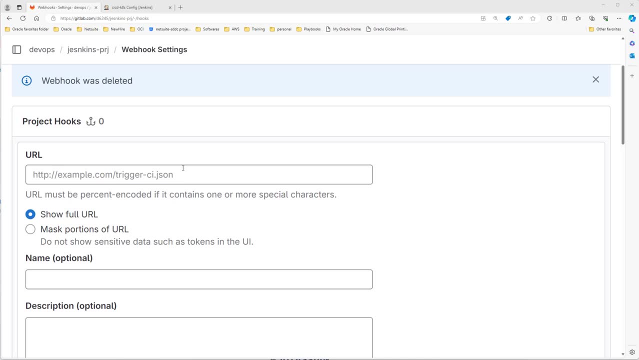 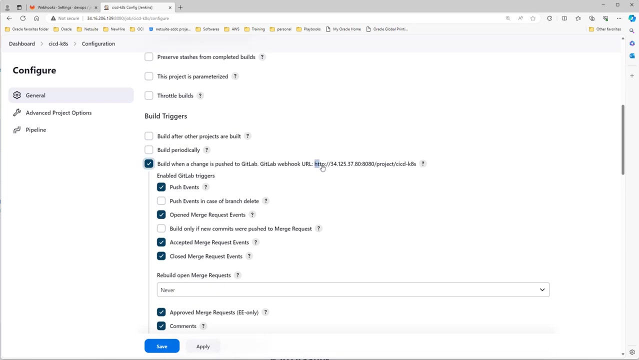 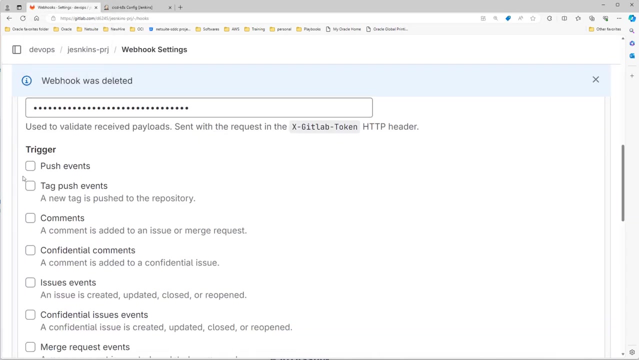 add new web hook here in secret token. let's paste the token and here it's the url for the url. let's back to jenkins and from here, as you see, it is written url, just we have to copy this one back to gitlab and paste it here. just click on trigger and that's enough, and add webhook. 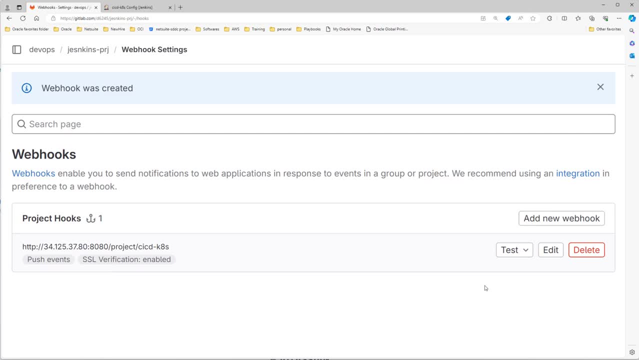 webhook added here. let do it a test. if i click here and click on push event, let's see what will happen here. you see we got an issue: hook execution failed. failed to open tcp connection to this address. what we can do to solve this issue in the recent version of gitlab. 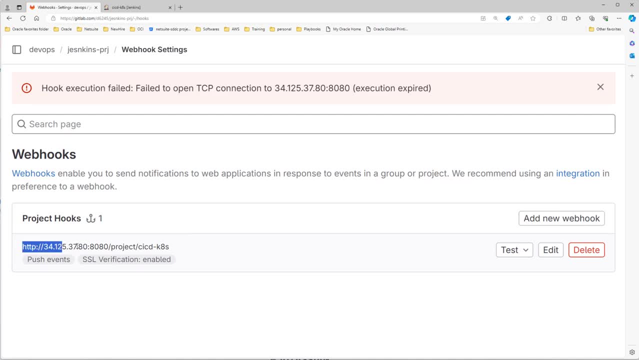 you are not permitted to using the ip address. you have to use https with ssl certification. so how we can solve it? there are some providers that give you free domain address so you can go and find one of them and use for this lab. for this one, you can go to this: 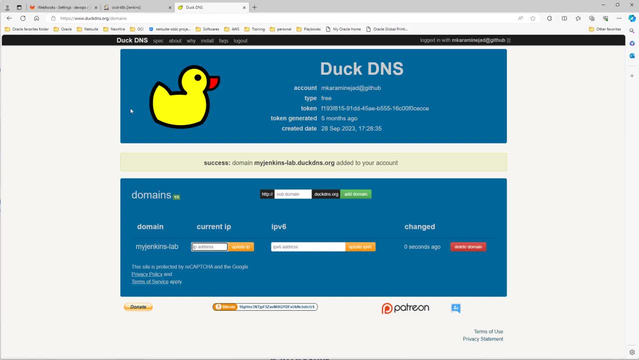 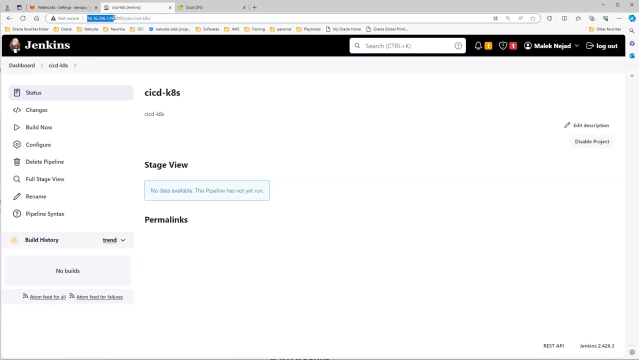 website doc. DNS and connect it by your github account and get a free domain. for example, I got this domain, my Jenkins dash lab dot doc. DNS, dot o-r-g. just I need to add my IP address here. let's go into Jenkins. copy the IP address back. 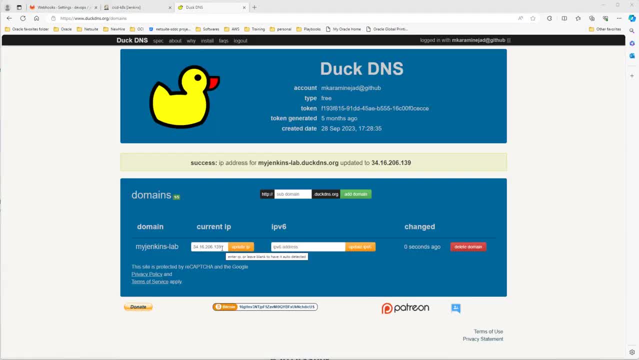 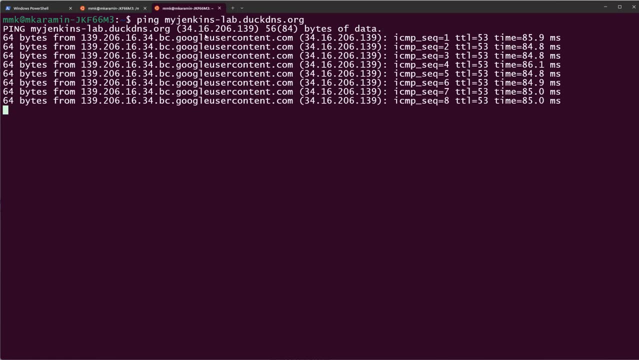 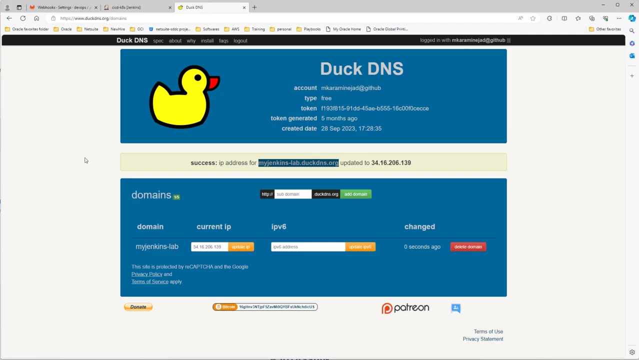 here: just add the IP address and update the IP. look here if I copy this address and back to terminal, ping that address. look here it's working. so we can use this address in a state of IP address. one another step is remaining. we have to enable SSP. 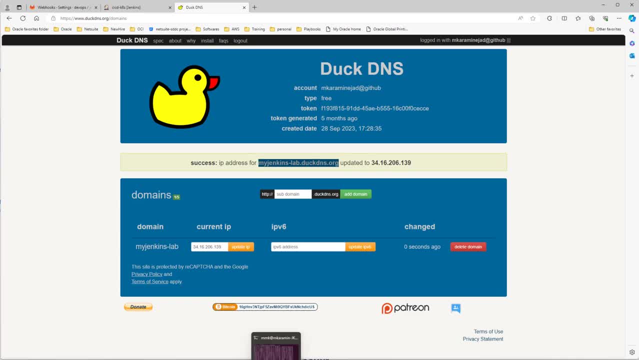 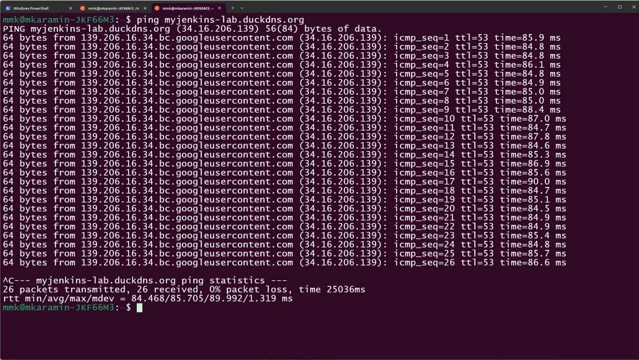 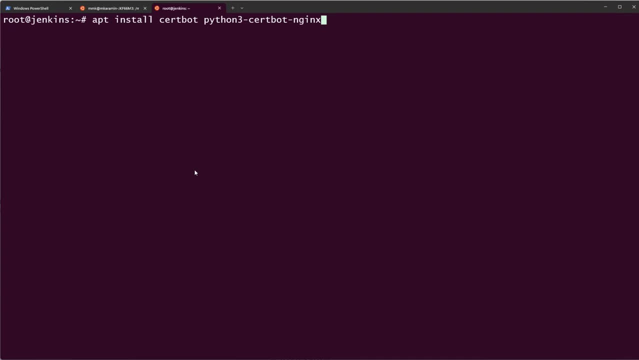 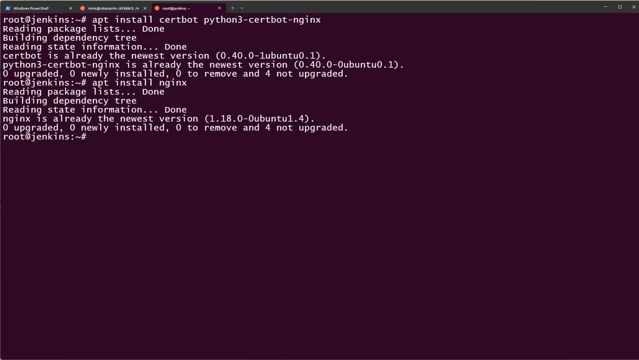 on Jenkins: just connect to Jenkins through terminal and let's see how we can enable SSL quickly after you connected to Jenkins machine. at first we need to install certbot package, plus Python certbot for nginx. let's install it. as you see, they are already installed- installed. and also we need to install nginx. as you see, nginx is already. 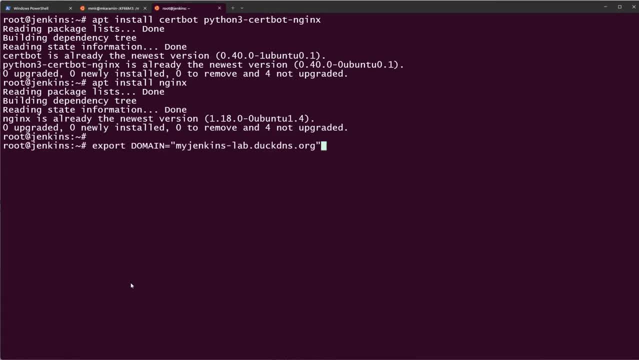 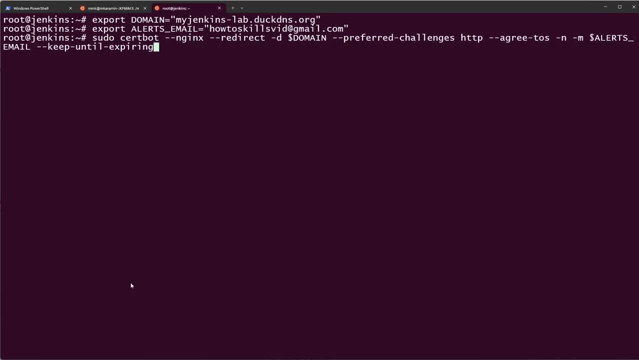 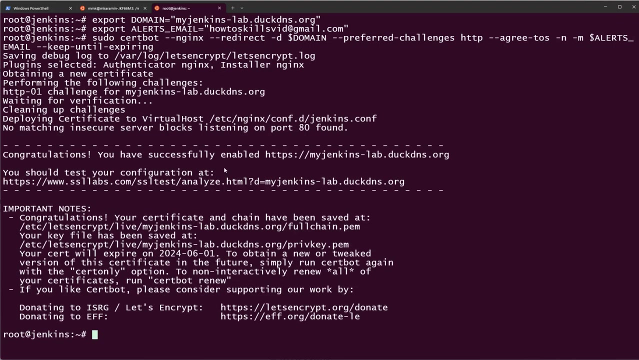 installed. just, I did define this environment variable also I did define this, this one. so with this command it will go and install SSL certification on this machine. let's run it. run it as you see. congratulation, you have successfully enabled HTTPS. my Jenkins dash lab dot doc. DNS dot. o-r-g. here you see the location of the. 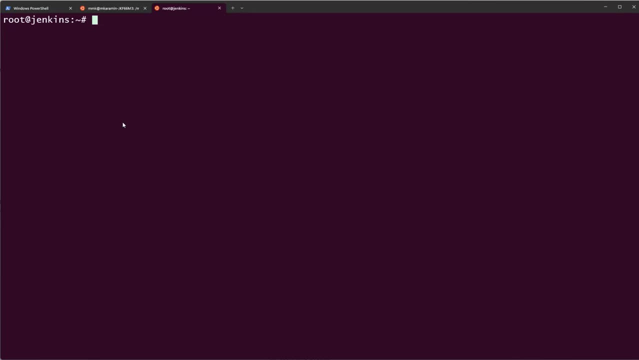 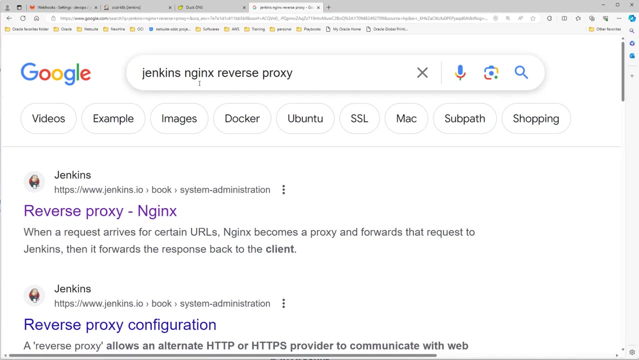 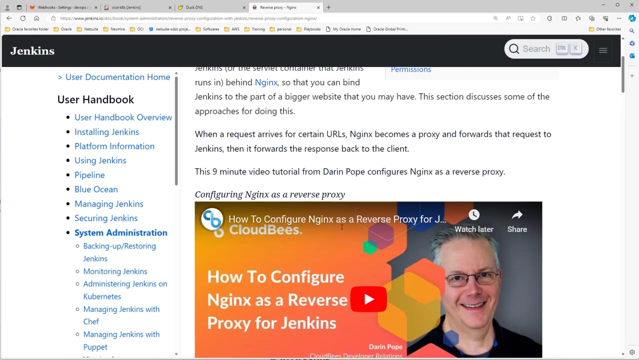 certificate on this machine. let's see how we can configure nginx to use as a reverse proxy and enable SSL for Jenkins. just if we go to Google and search for Jenkins, nginx, reverse proxy and from the result click on the first one, you see there is a video for that and also all the configuration. 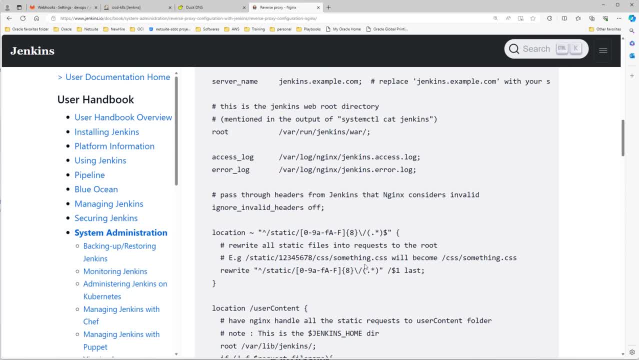 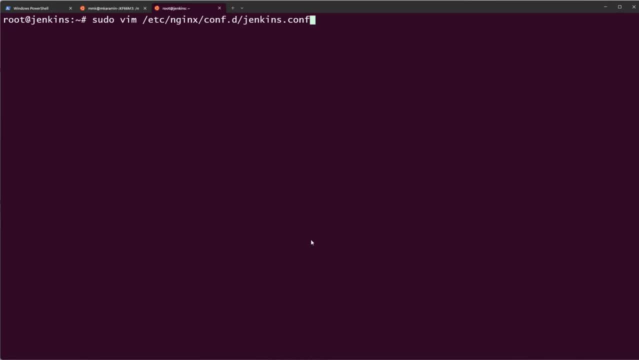 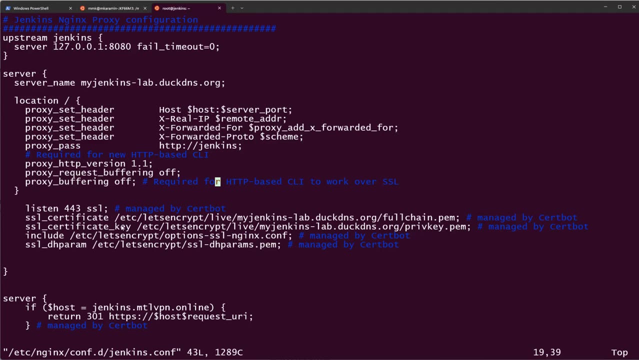 is here. we can just copy this configuration and back to terminal and going to this address and open it and paste it here. you see, here in this section the address is automatically configured here my Jenkins dash lab dot doc. DNS. just you have to update your address here. I did it this. 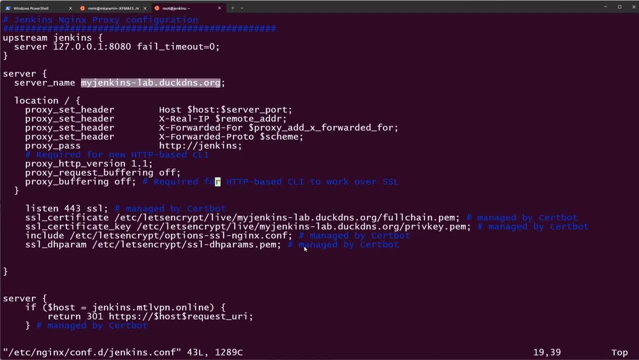 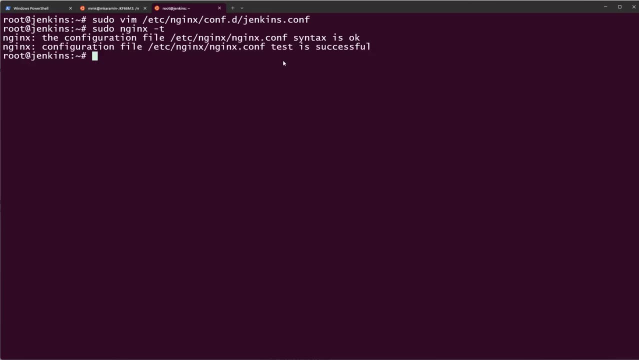 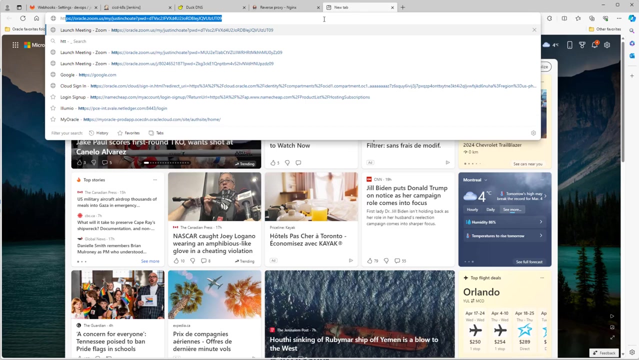 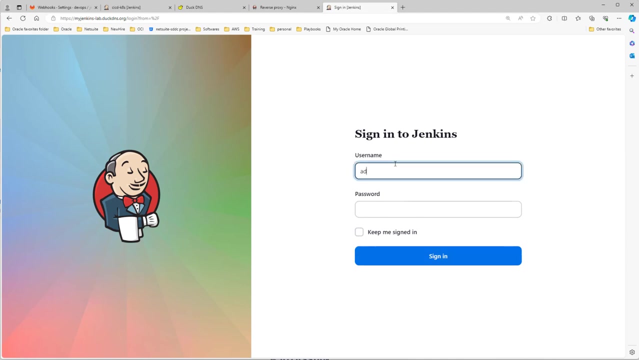 one manually, the the others managed by certbot, as you see here. just you have to change this one manually, so let's save it and type: sodo, nginx, dash T. look here: test is successful. let's copy this address in browser: HTTPS and enter: look here: SSL is enabled, so just type username, password and. 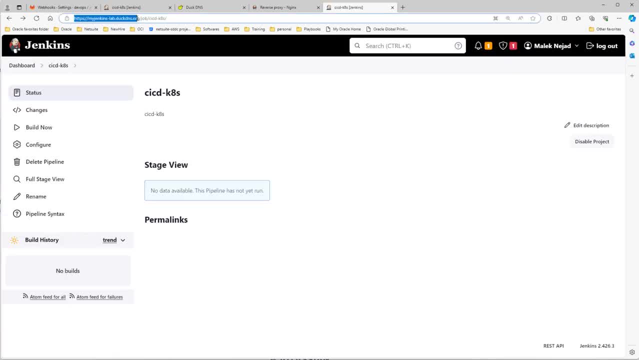 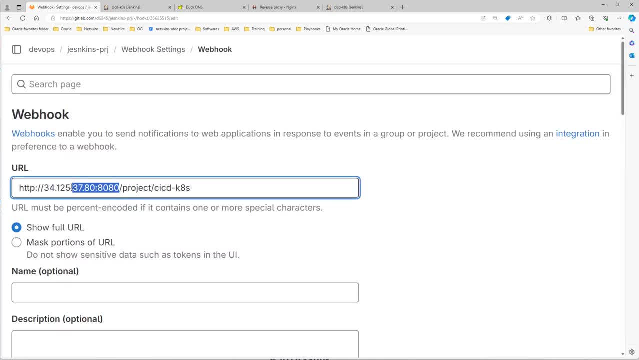 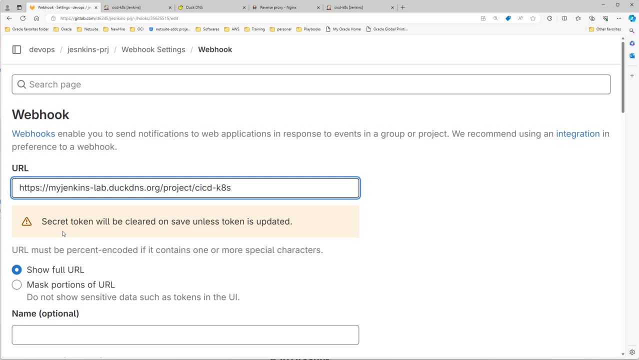 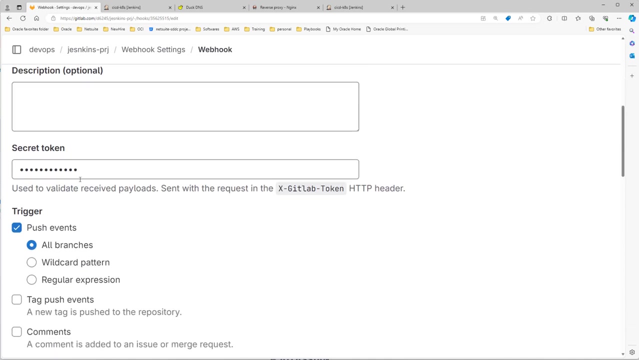 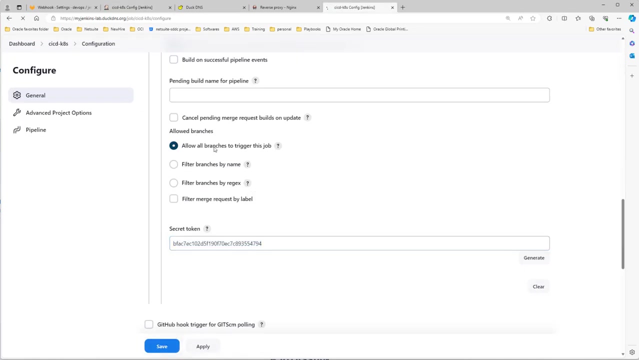 connect by it. so let's copy only the address and back to webhook on gitlab edit and in this section we change it to this address and, as you see the message here, secret token will be cleared on save unless token is updated. so let's back to Jenkins in configuration, copy it, save it back to. 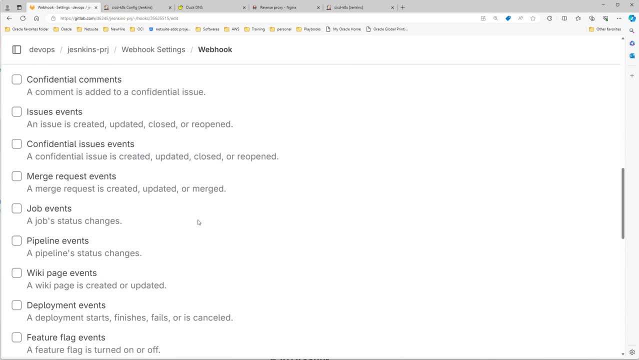 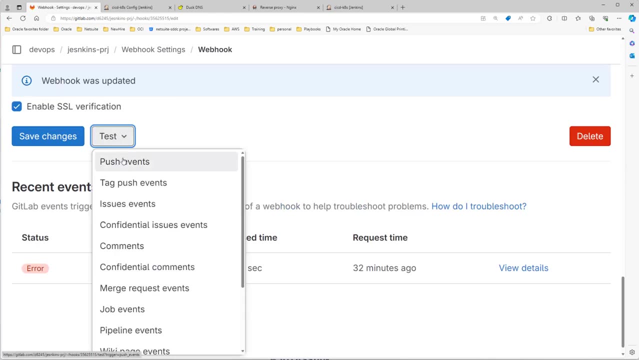 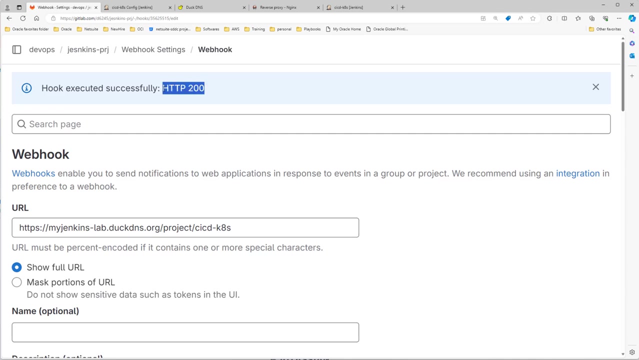 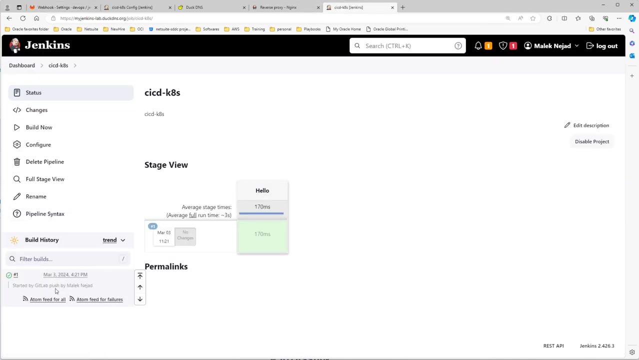 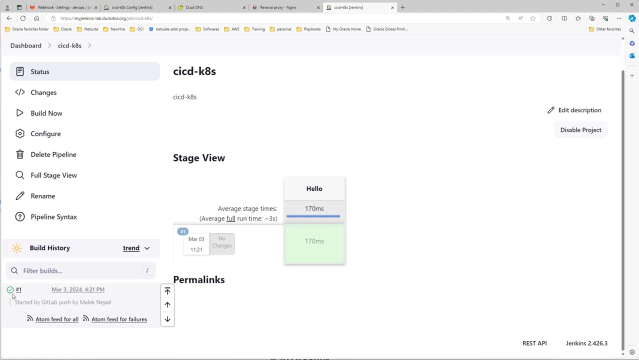 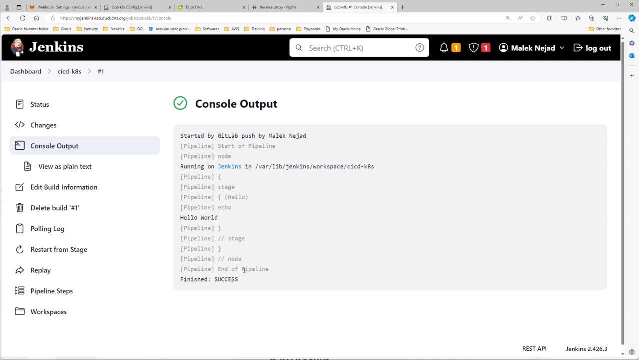 webhook and paste it here and save it in this time. if I do a test, let's see what will happen. hook executed successfully with this code: http 200. let's back to Jenkins. look here: webhook trigger Jenkins successfully and the project ran successfully. look here: this is the output. so until now we could connect. 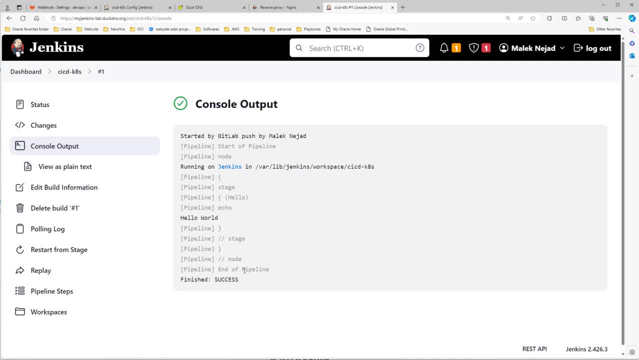 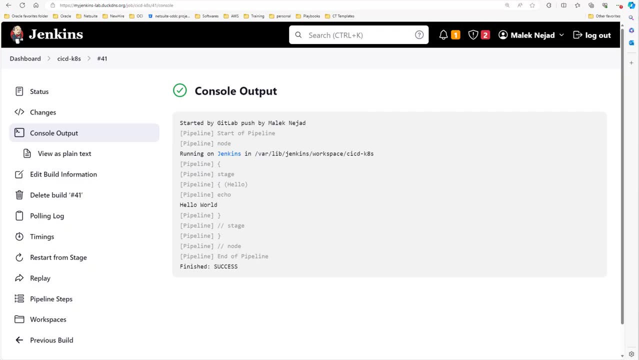 Jenkins to the gitlab and also enabled webhook to trigger Jenkins job. so let's go into the next step and configure our job on Jenkins. before configure the build job, let's see which steps we need to do to build an image. for building an image, at first we need to 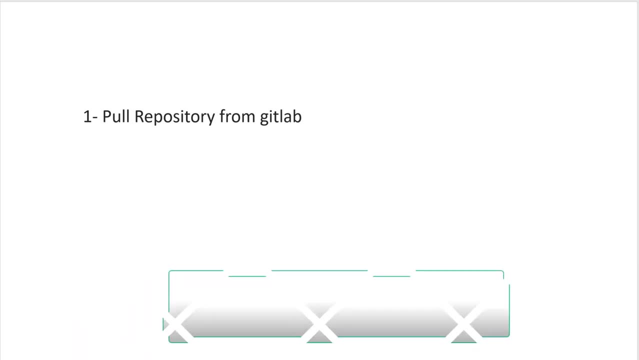 pull repository from gitlab, because our source data is located in Jenkins dash prj repository on gitlab and and here on Jenkins. at first we have to pull this repository and then build an image. so in first step, let's pull repository from gitlab. how to do that? let's 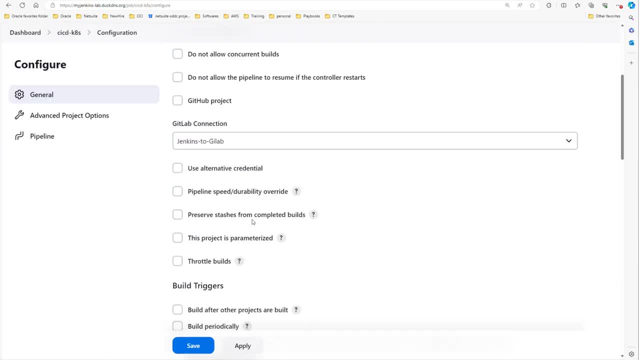 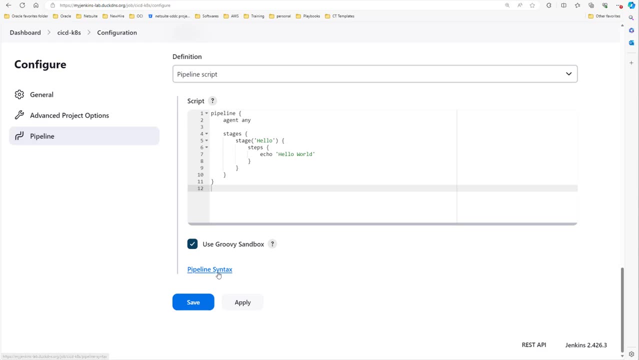 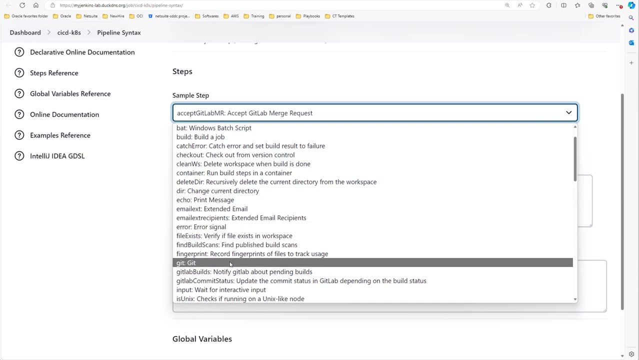 go into Jenkins back to job configure. going down here at the end you see pipeline syntax. let's techno. let's configure my github applications to r x and have a look on what this. going down here you see pipeline syntax. let's click on it from the sample steps. let's going down and select git here. ask you, where is the link of? 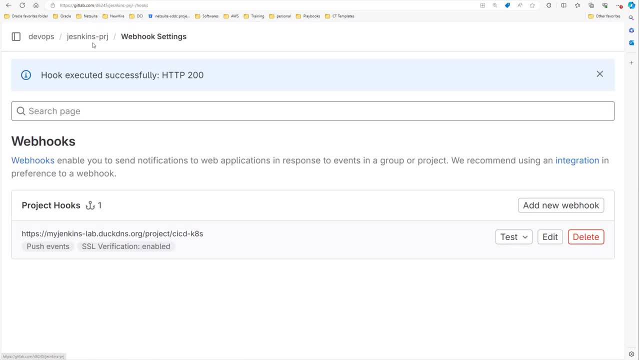 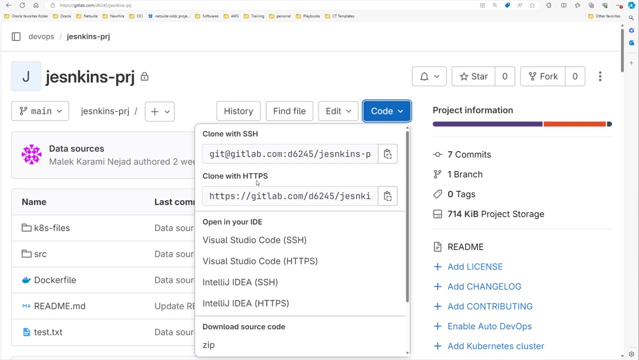 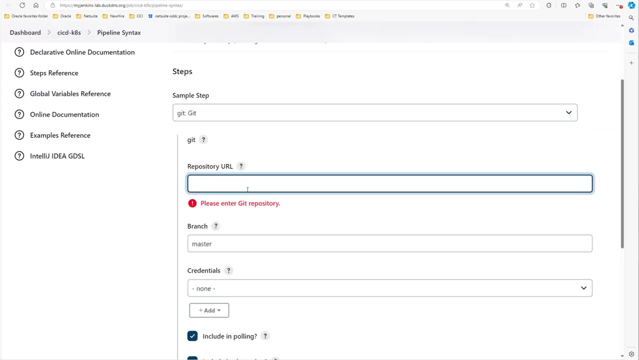 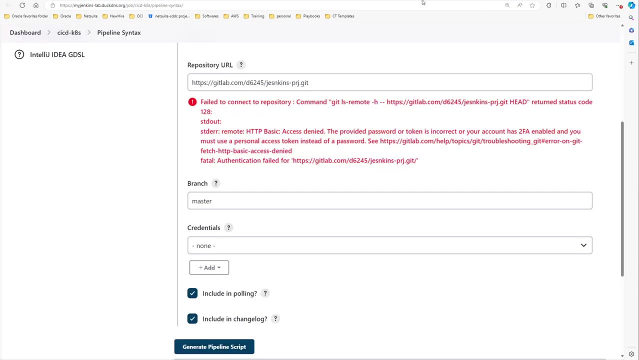 your repository, from the gitlab back to Jenkins dash prj from the code and clone with https, copy the link back to Jenkins generator and paste the URL here. what is the branch name? the branch name is main, so here just type main. you see here a failed to connect to repository because at the 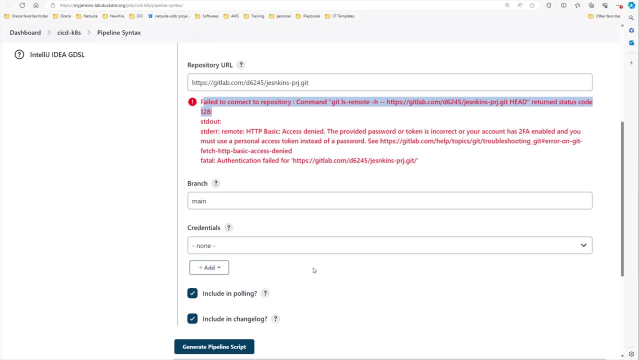 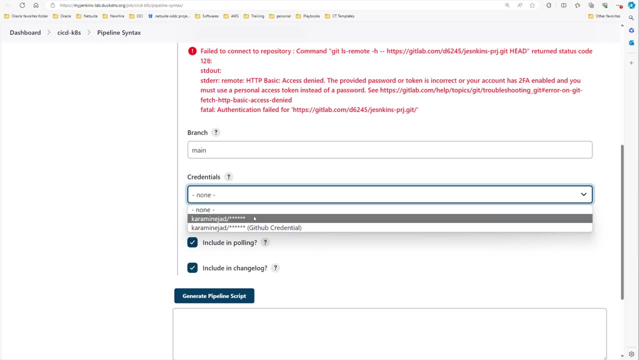 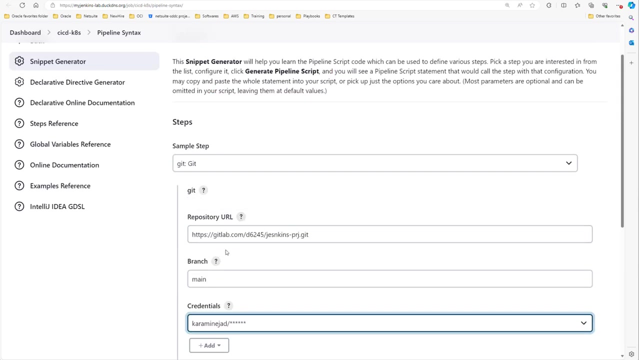 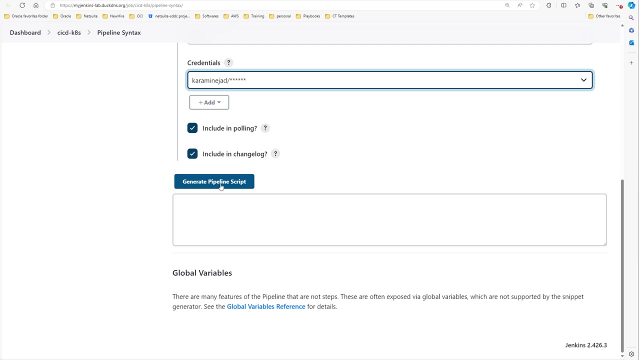 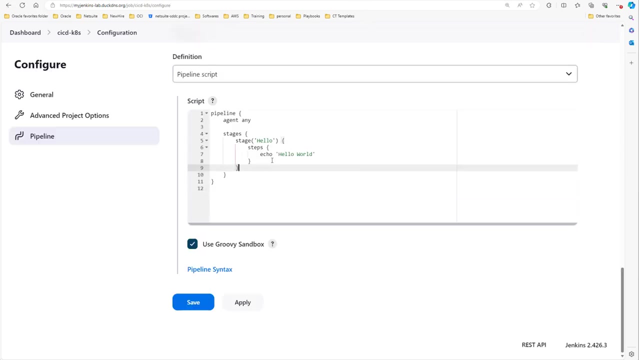 moment. still, we didn't mention the credential in the credential section. open it, select the credential related to gitlab. as you see that error gone, let's going down and click on generate pipeline. script done, just copy this one back to config and here in the stage, let's. 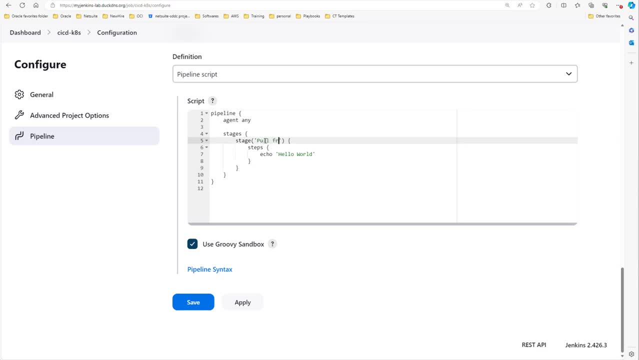 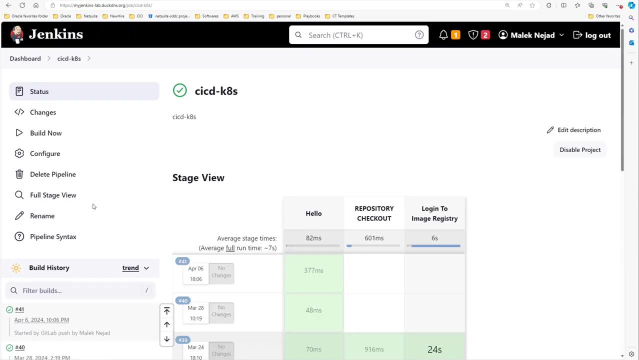 change this stage to pull from. just type this one and in the step let's, let's grab this one and paste the new command here, let's save it. let's manually run it and see if it works. build now. look here. now it's going to connect to gitlab and pull repository here. look, it's successfully done. 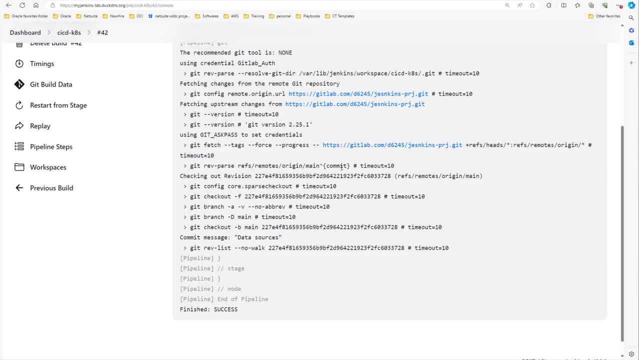 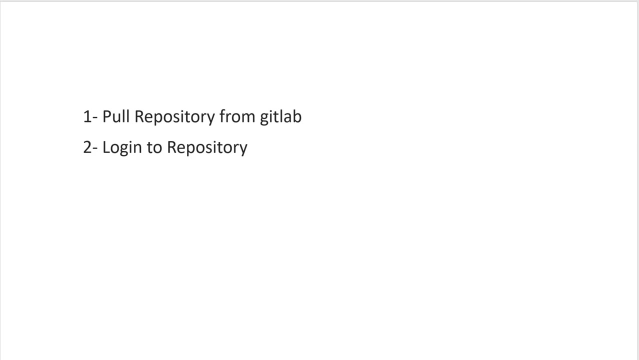 if I click here you will see it went and download the repository here on Jenkins server. what we need to do in the next step. in the next step we need to log in to repository. before building an image we need to log into repository. then we can build image and push that. 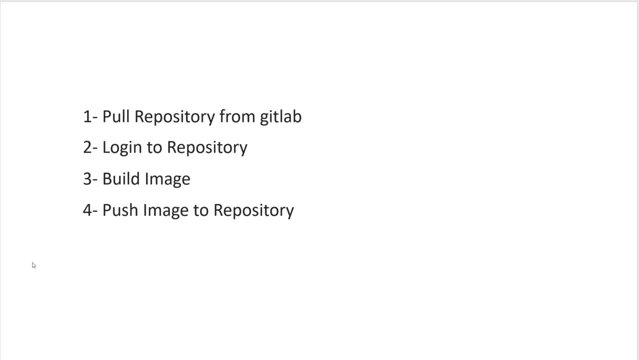 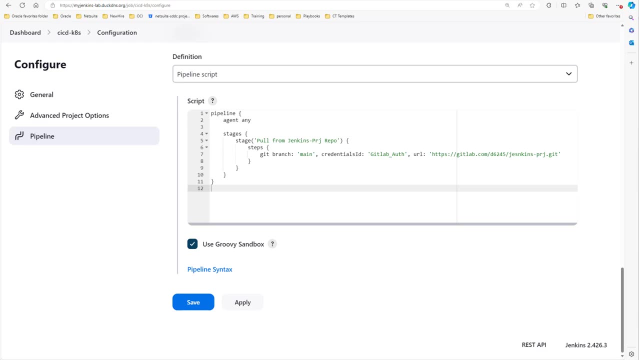 image to repository. let's back to Jenkins, back to job going to configure. let's going down here. let's to add another stage. let's copy this one and add it here. let's change the title: to login and build image. how to log in to image registry. here we are going to use. 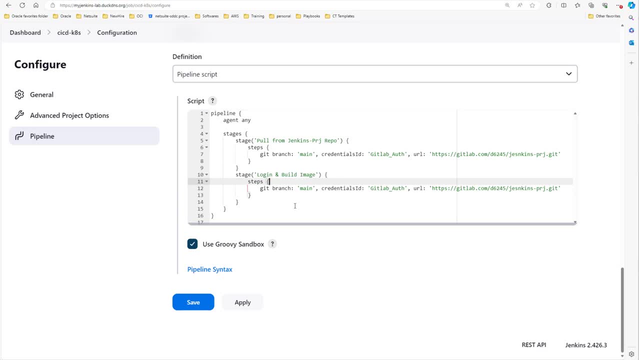 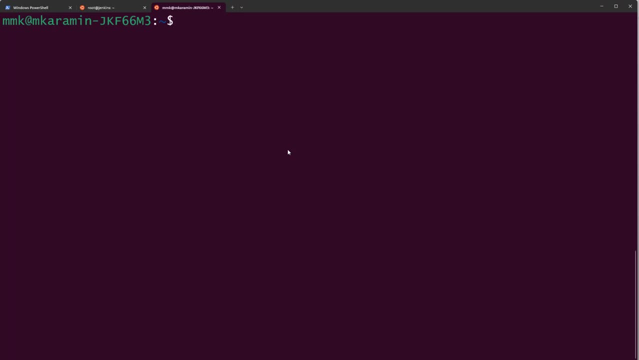 gitlab image registry. let's go into terminal. in terminal, when we wanted to log in to docker registry or gitlab registry, just type docker login. if we only use this one, it will go and connect to docker hub. but we don't want to connect to docker hub. we want to connect to. 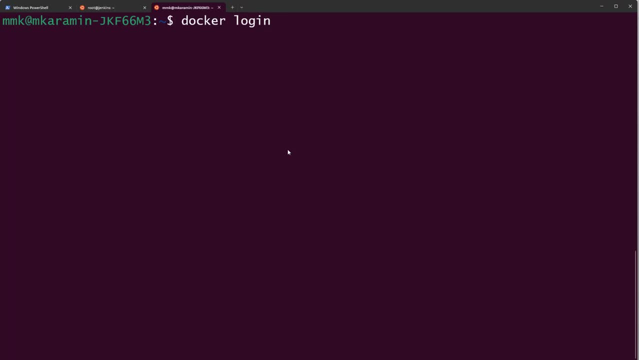 image registry. so here we have to define the address of that registry for the gitlab. just type registrygitlabcom, enter it will ask username and after we type the username it will ask the password. also here we can use the register. and then there we go. we are satisfied. as you can see, the registry is connected to and the grate i can read the data is landing on Anko. we are now able to tap an image and the registry is beenzh the endpoint. 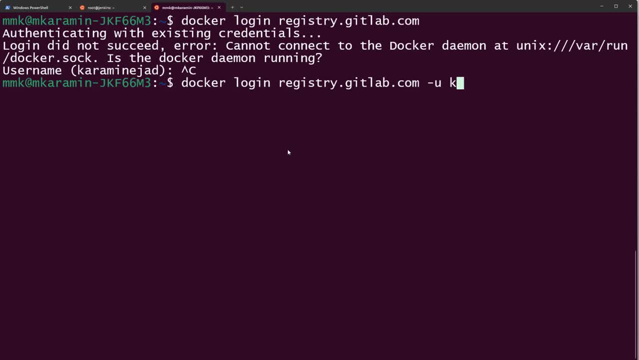 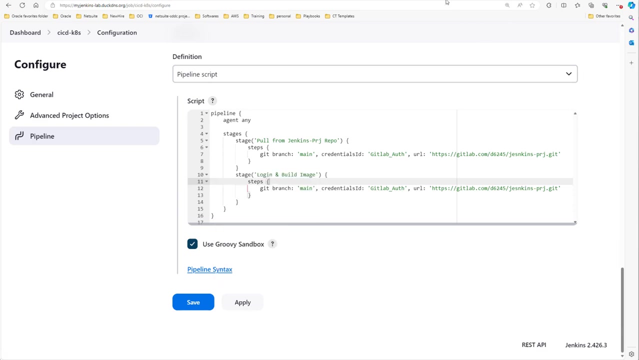 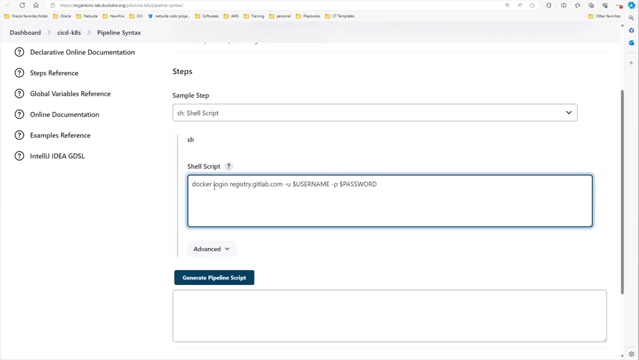 here we can use dash u, my username, dash p, the password, or let's enter here we'll ask the password. so we have to use this command on jenkins. let's back to jenkins. click on pipeline syntax. open in new page. from here, just going to shell script, do like this: docker login: registrygitlabcom. 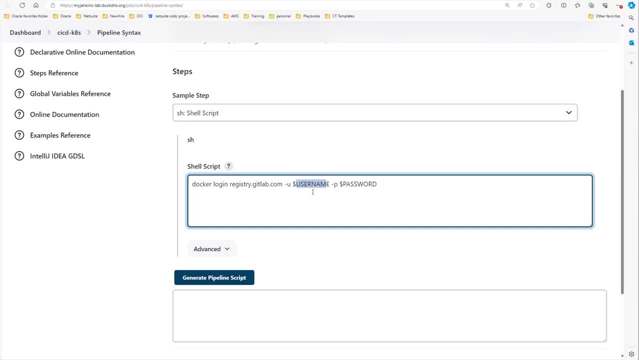 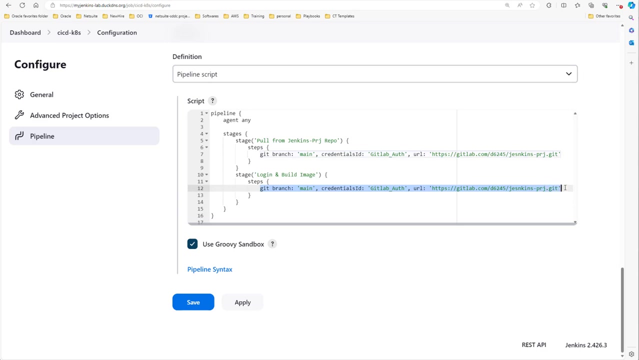 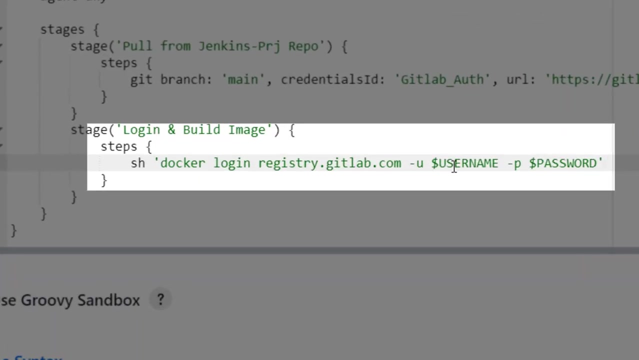 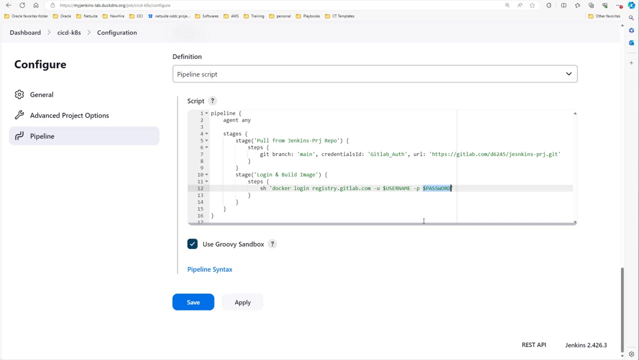 dash u using this variable username and this variable for password. let's generate this script, copy this one back to jenkins and let's grab this one and replace it here. at the moment these questions comes to your mind- where we have defined this username and password. if you remember, we defined before gitlab authentication. on credential. here we have to use this one to generate username and password. let's back again to pipeline syntax. syntax generator from the sample step: click here. going down here you will see with credential, bind credential to variables. let's click on this one in the bindings, let's click on add username and 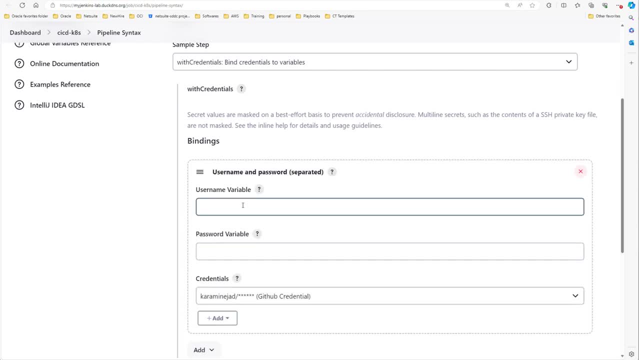 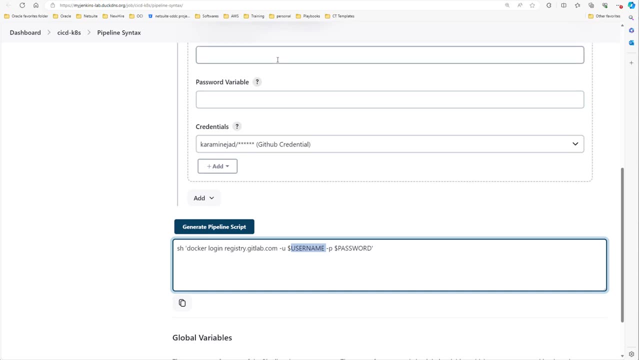 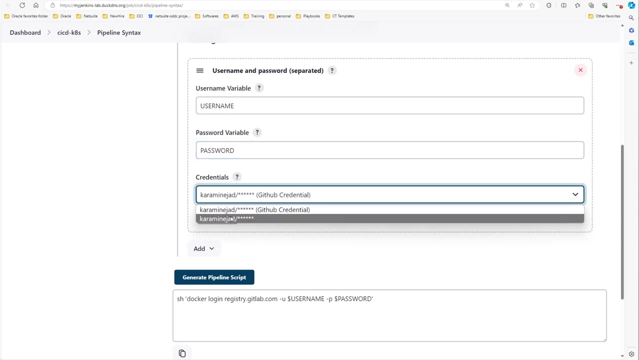 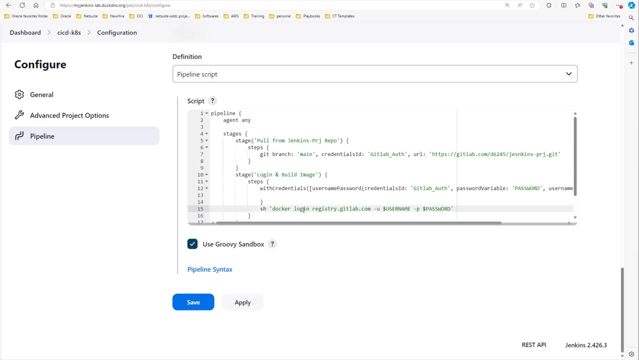 password separated. which username variable you want to use as we add in this command username, let's copy this one. copy it here. and for the password, copy it here. from which credential? the credential that we used for gitlab? let's generate and copy this one. ctrl c back to here and b for login: add it here, so let's. 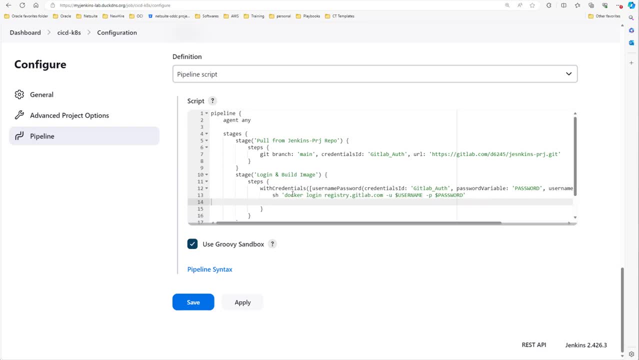 remove this one from here and put it here, so it will go and grab gitlab authentication and let's OHL. that's it. we're working. now we're ready to do a, and from here I am going to add this one, see, and from this one it will extract username and password that we defined in credential before. 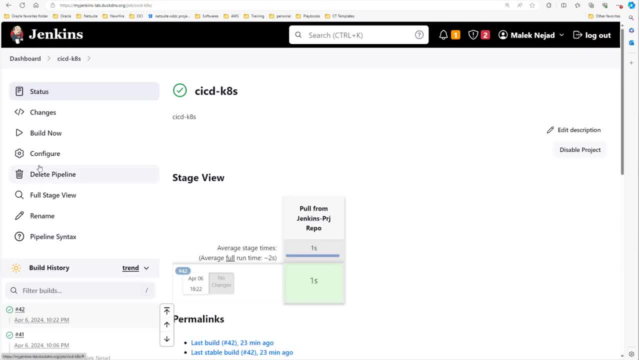 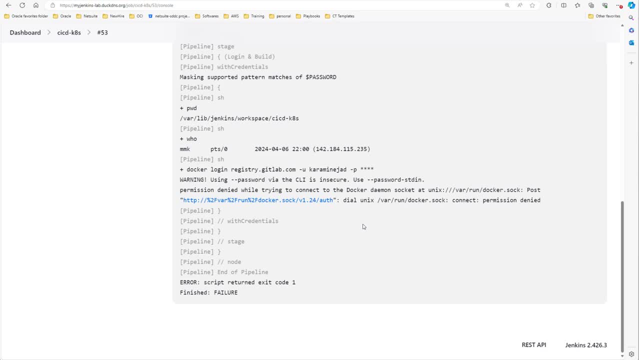 let's save it and let's do a test. let's see what's the issue going down, as you see here: permission denied, it seems. the user that wanna run the docker has no permission for solving this issue. you can copy this error and search on google and finally you will find like this: 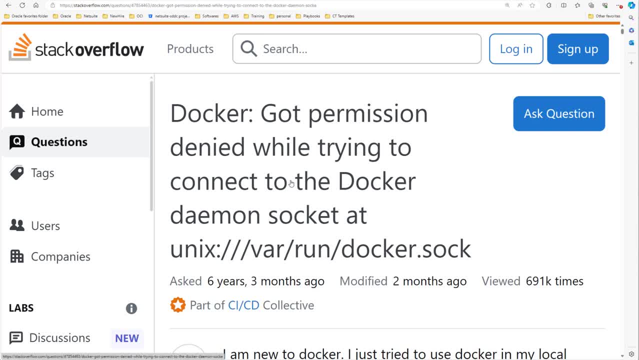 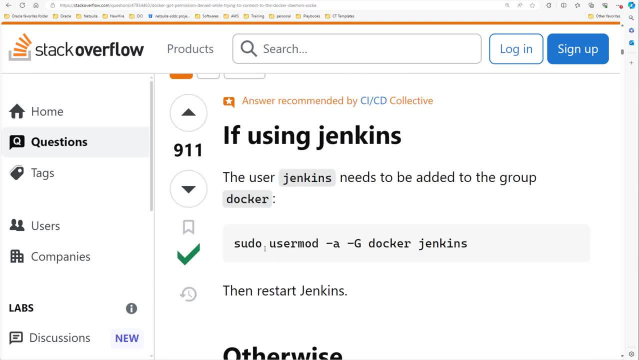 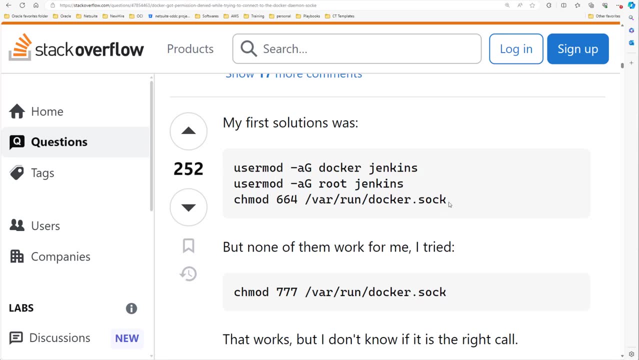 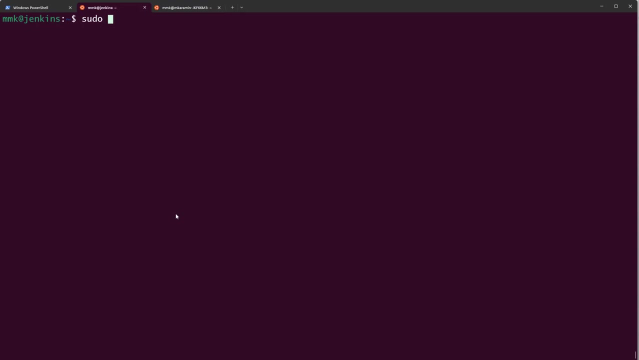 got permission denied while trying to connect to docker diamond socket. let's go down and see how we can solve it. you can use like this, or going down, grab this command and run on the jenkins terminal. if i grab them, copy here is jenkins, just sodo dash i and run them as root. okay, let's back to jenkins. 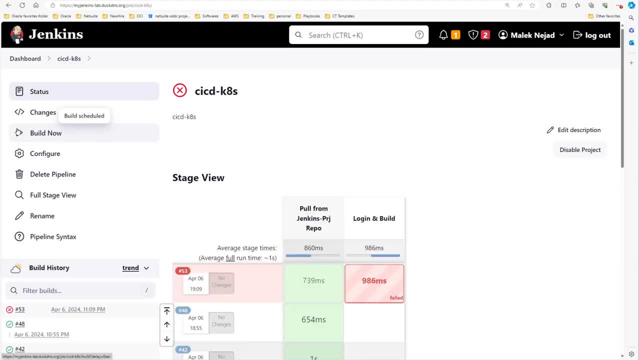 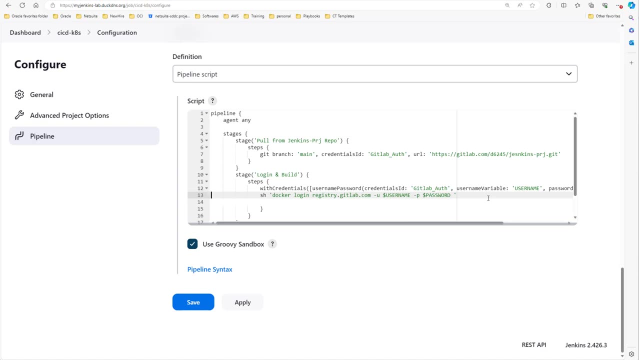 dashboard. going to the job and build it again. here you see, it worked successfully. okay, let's back to the jenkins dashboard and run on the docker diamond socket. let's go down and see back to job. going to configure and it could successfully log into gitlab image registry. 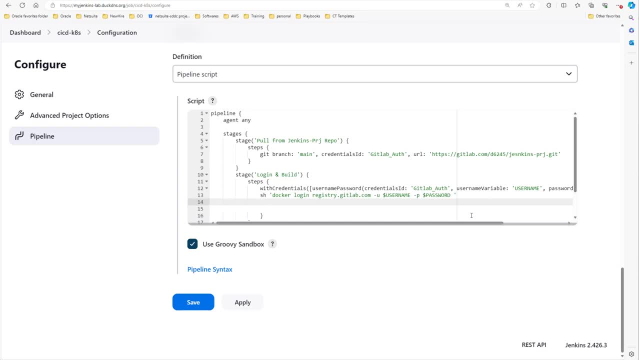 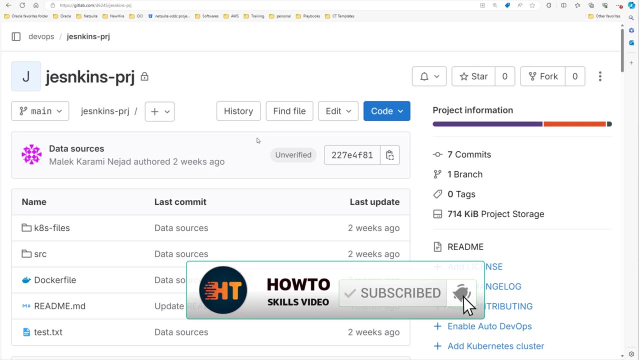 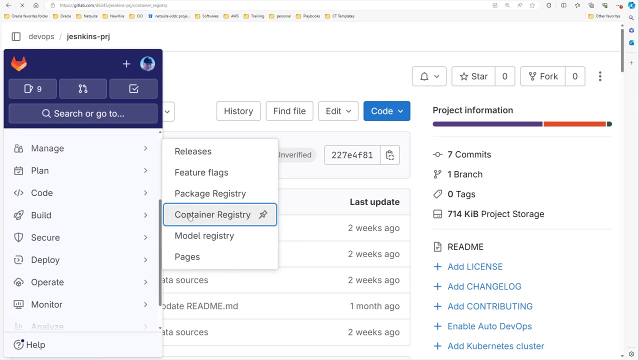 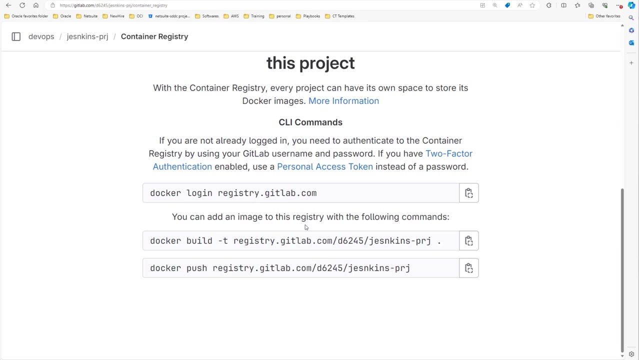 okay, so let's add another command to build image. let's back to gitlab. also, i want to use this repository as image registry. so from the left side going down, deploy container- registry at the moment is empty. going down, you can add an image to this registry. 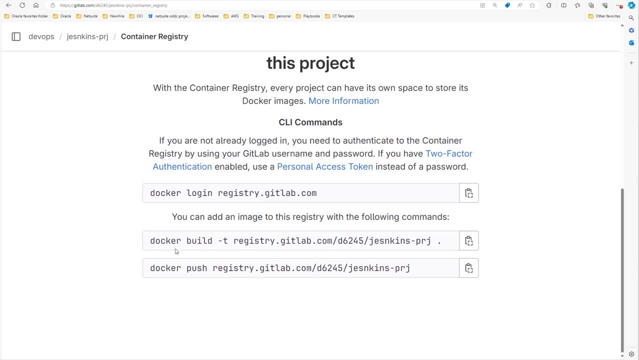 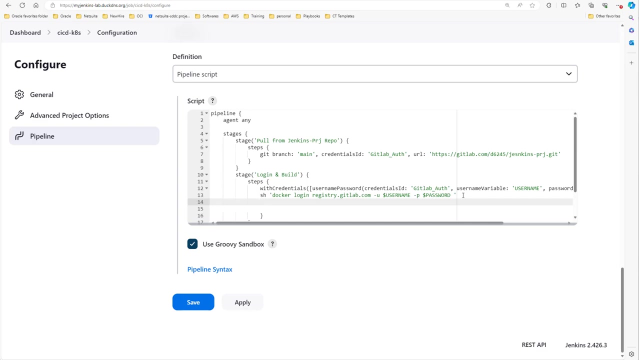 with the following commands. as you see, the first one will build an image and the second one will push the built image to registry. so let's grab the first one back to jenkins. let's go back to gitlab. we are going to say that this large good jenkins could build the video last liedzemit, so take这个. 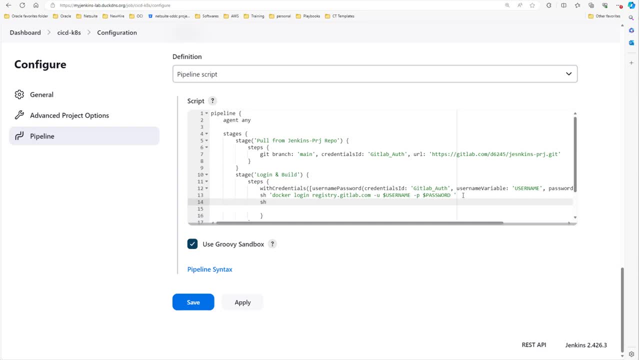 one. we normally start off with Google chrome, so let's go to google��呢, we're going to create a and we're going to create an image. oh, let's take one single image, something like that. you should remember: in youtube, when they pass forward, there's always a lot of buttons we can. 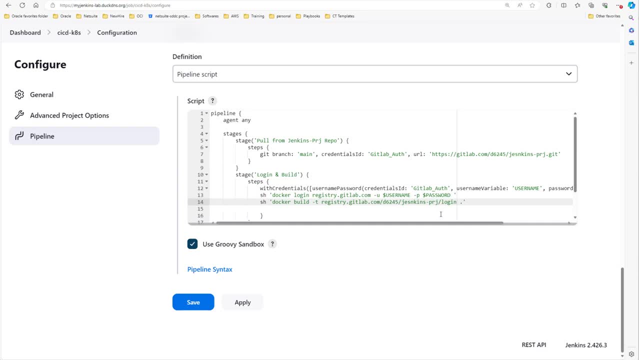 actually hard to enter into bio. it's open, so you didn't have to do this at first, but you can do it. if you have some animations that are already built, like dating, you're going to be able to use some actives in this, while that mode is available inside gitlab soon, but we would love to see the same. 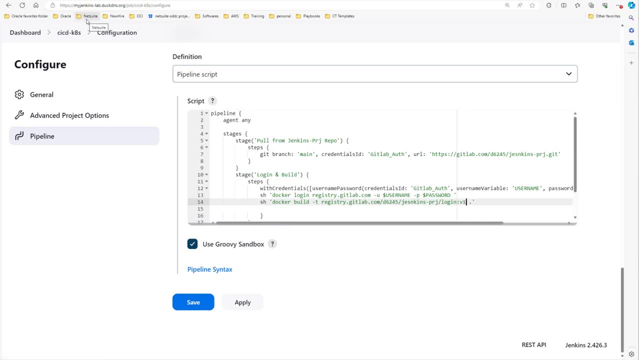 so as to. so that's going to configure and add it here again. we use the sh because we want to run the command open quotation and paste it here. one also, let's grab the other one, copy this one back again to Jenkins and add a new line. 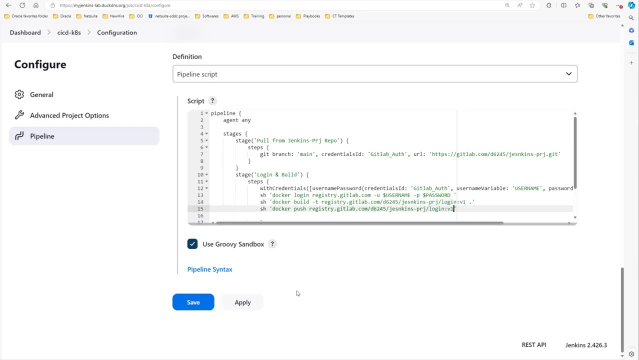 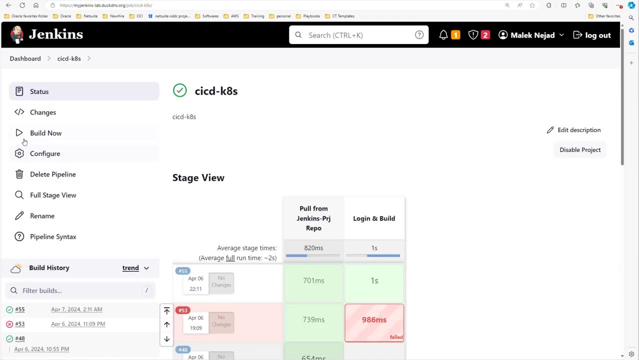 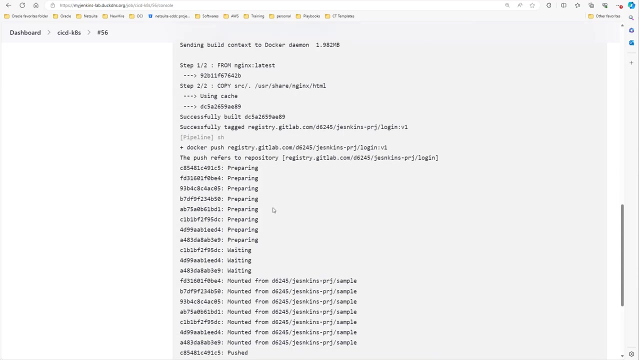 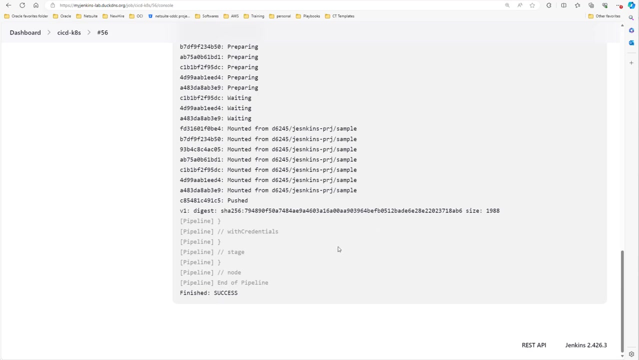 add this one at the end. just, we are doing a test. let's save it and click on build and see the result. let's click on this one and see here: look here it will go and build an image and finally push it to registry and you see the job finished successfully. let's back to 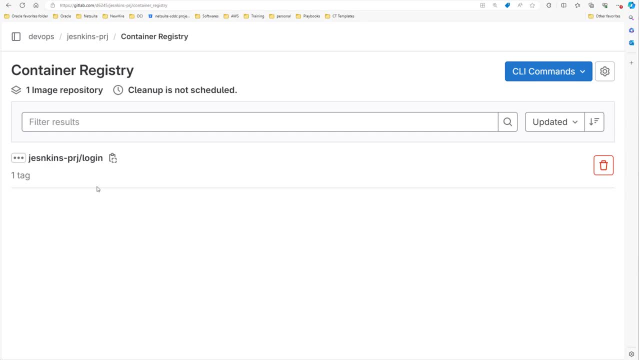 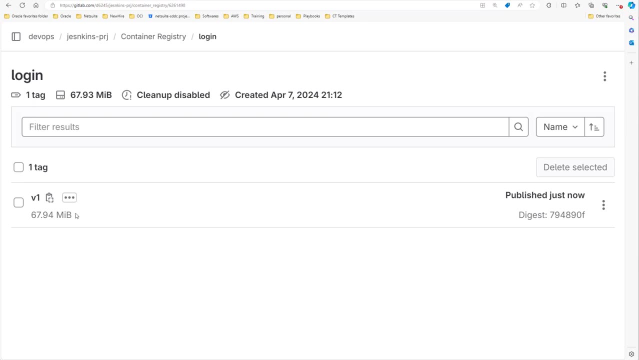 GitLab and refresh page. look here: one tag added here. let's click on this one. and here the version one. as you saw, we could build an image and push it to GitLab registry. let's back to job and see the result. let's back to GitLab and refresh page. look here, one tag added here, let's. 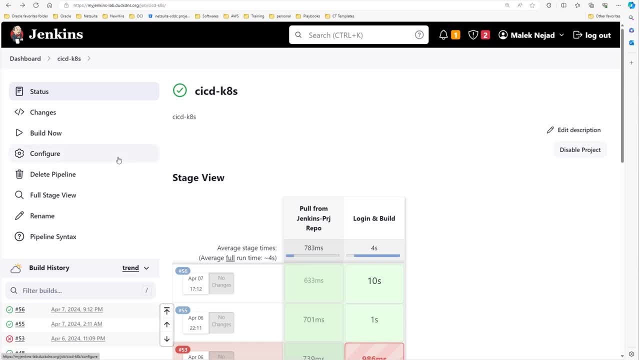 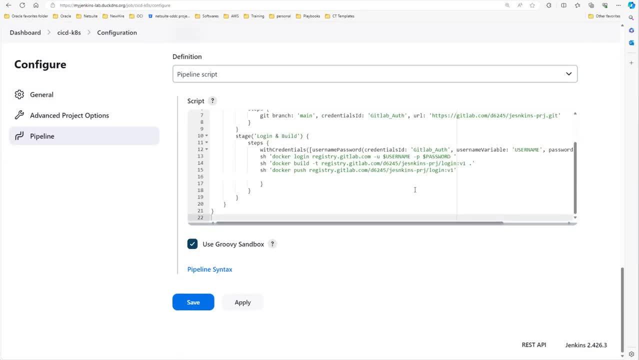 and make a little change on that to be more user friendly. going to configure and going down. this is the job that we are working on that. so you see here, if every time we want to run this one and change this version manually, it's not user friendly, so how we can change it automatically. 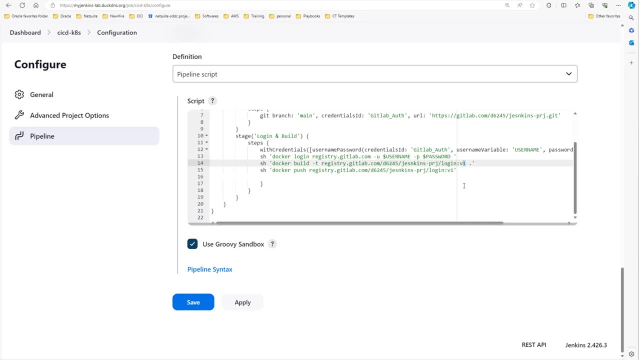 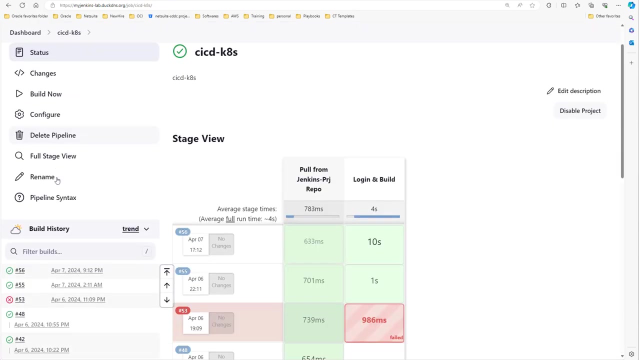 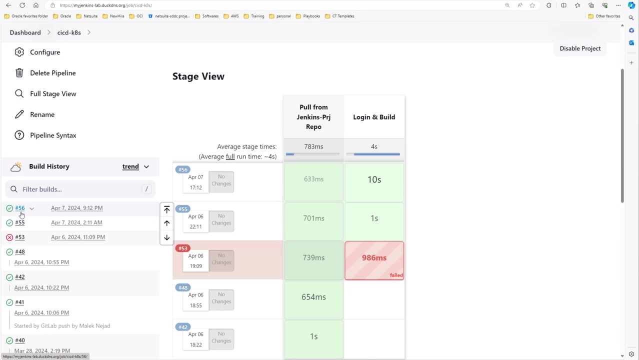 and each time we run build job automatically increase by one, for example, version 2, version 3 and so on. one of the way that we can use it using the build number. let's back here, for example, at the moment we are on build 56, so if i again run it it will increase to 57, so we want to use this. 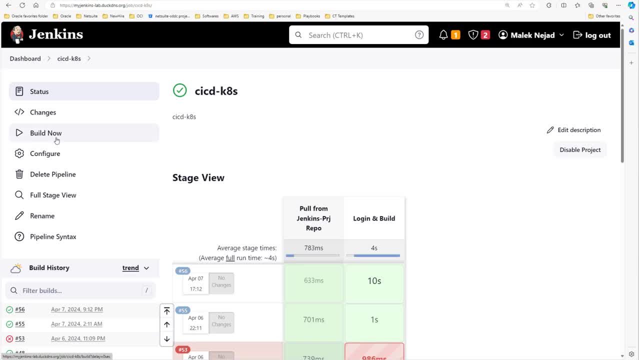 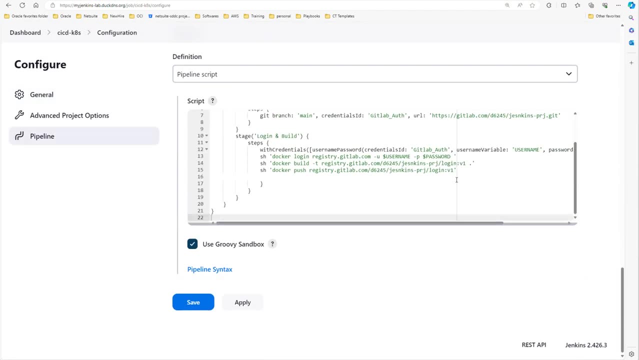 number on build. so let's going here- sorry i made a mistake and run it again, so let's finish it. okay, 57, next time will be 58.. so let's going to configure, going down how we can do that we can define environment variables and use it here. how we can do that. we can type environment open and. 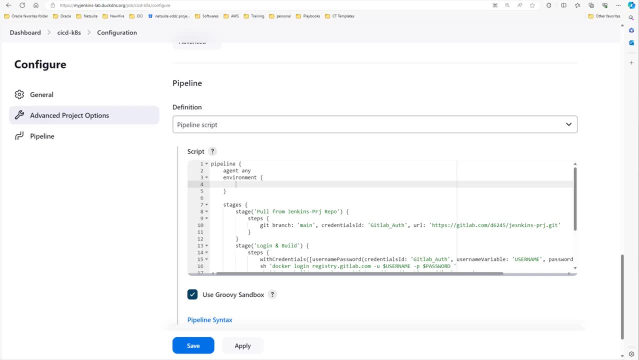 so let's enter here. we can define version like this: one version environment build id. if we install gitlab plugin- that we did at the start of this session- we can retrieve the build id. each time we run our job we can get build id, so it will save it in the build id. so let's go ahead and 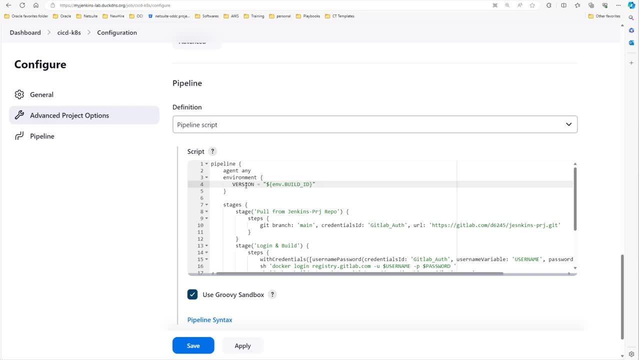 then we can change it to any type of build id, such as json build id, or we can change it to name version, and if we choose to use the name or we can change it to tag everything you want you can define here. also, i can define another variable. 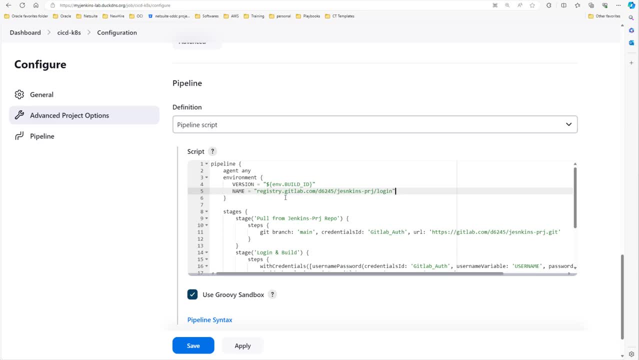 like this: one name or path: registrygitlabcom and my repository, and this is the name of the build image. so let's going down and use these two variables here. so instead of this one, i can remove from here to here and replace like this and the same for: 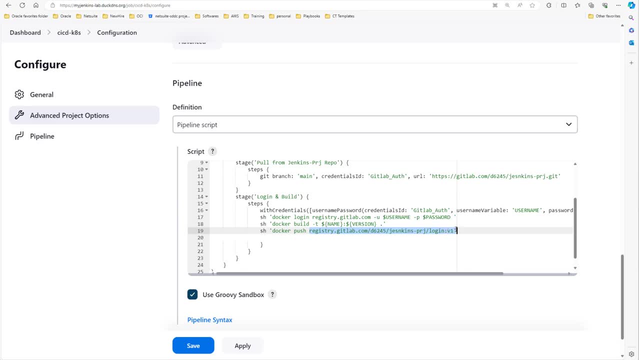 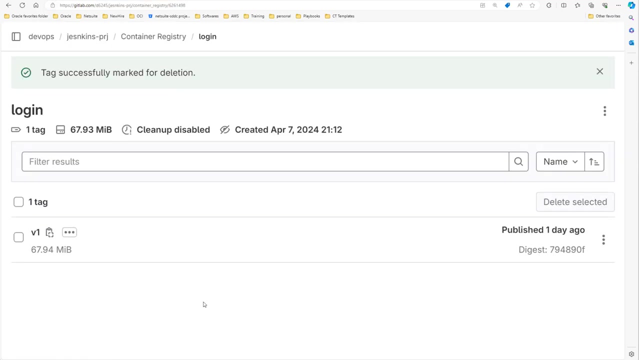 the next line, just replace to this one. it's more user friendly and each time we run the job automatically we'll get the build number as tag. let's save it before click on build. let's go into gitlab and here in image registry. at the moment we have version one. now let's back to 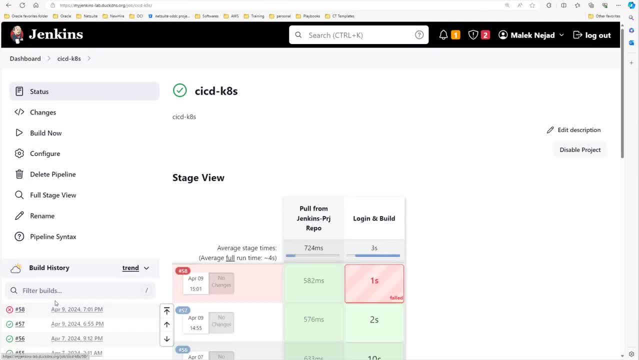 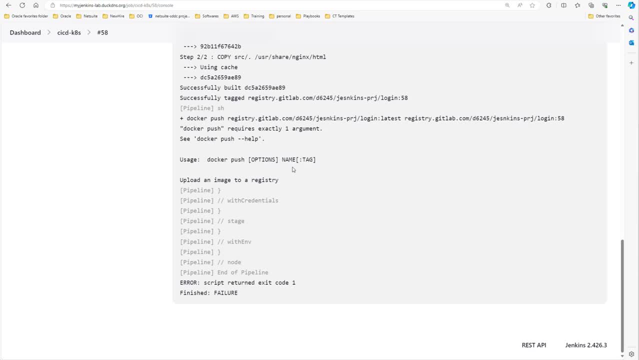 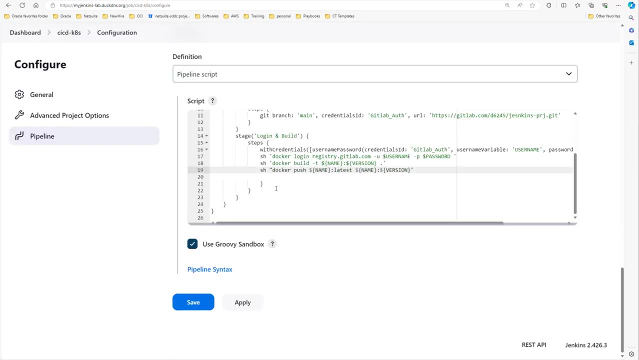 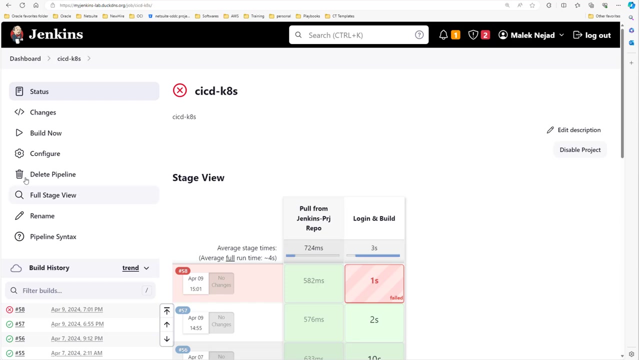 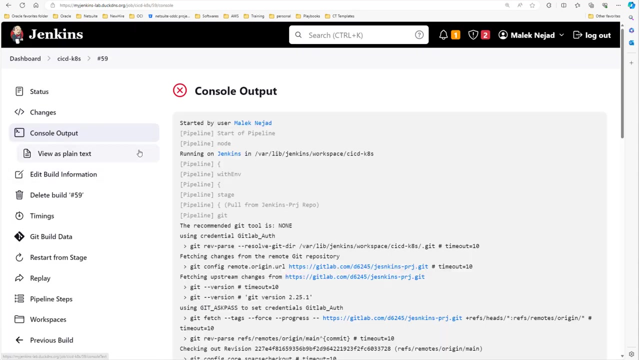 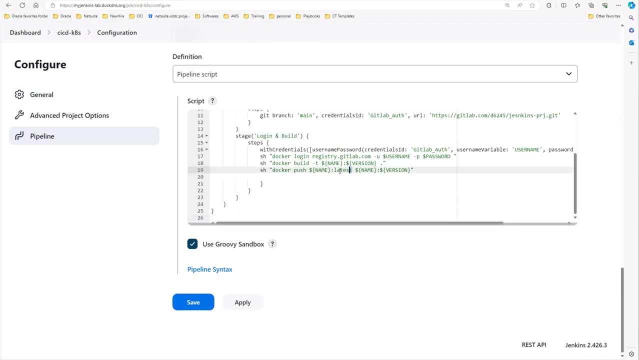 jenkins and click on build. let's see why it is failed. get problem here. let's check it again. back to configure. as my experience, it is better to change to double quotation and the same for this one and run it again. again, we got issue. let's click it here. it seems i made a mistake somewhere. let's configure going down. yes, let's. 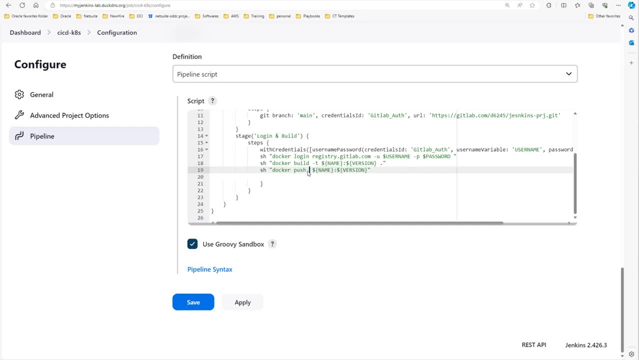 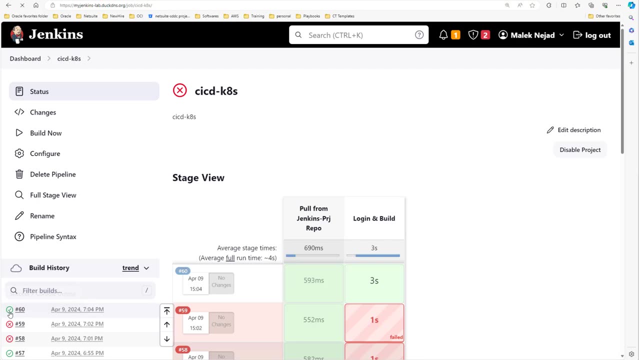 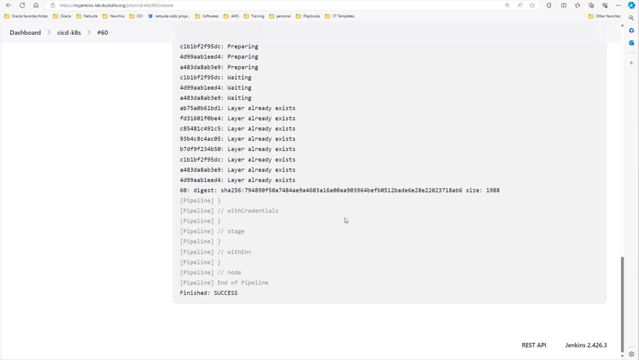 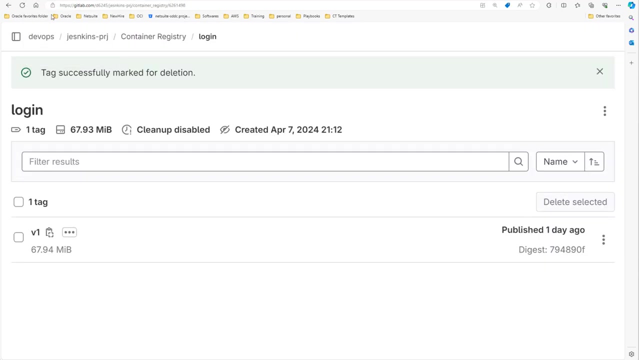 this one. we don't need it, just git, push, okay, let's save it and build it again. this time run successfully. let's going down here, build image and then push it to registry. let's back to registry and see if everything going well. let's refresh this page. look here: this tag 60: 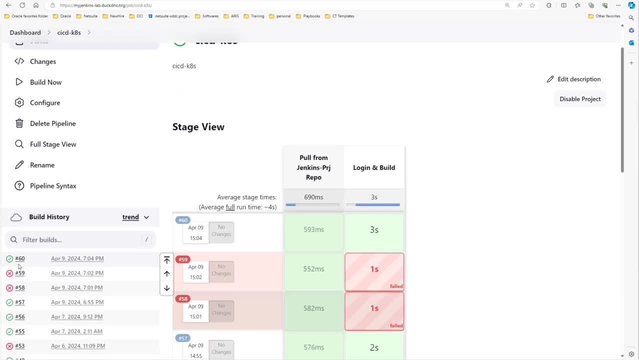 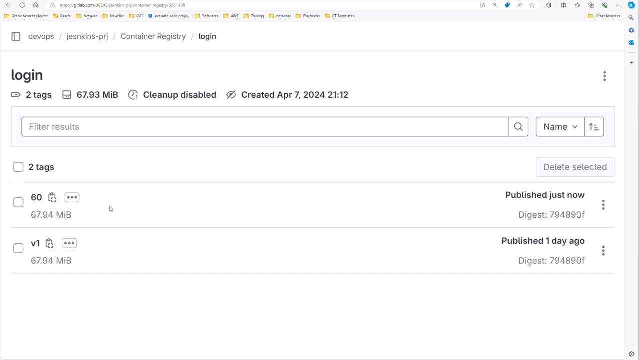 this one 60.. back to here, the successful job 60 push it here. so far, so good. now let's going one step forward and update this tag there in helm chart that we have there. let's going here, if i going down, and click on manifest repo. 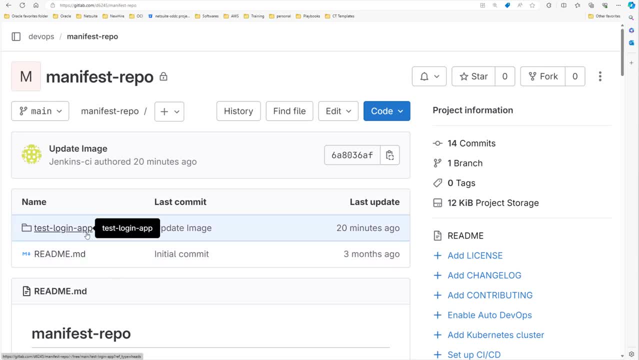 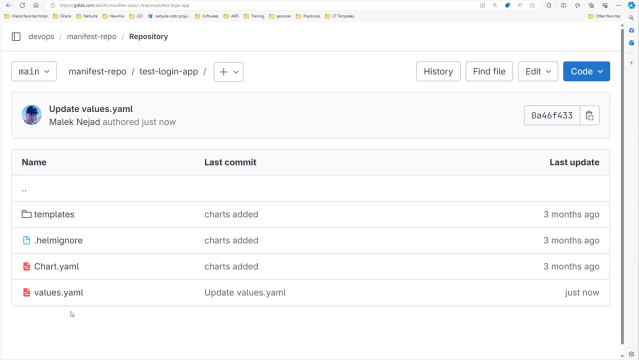 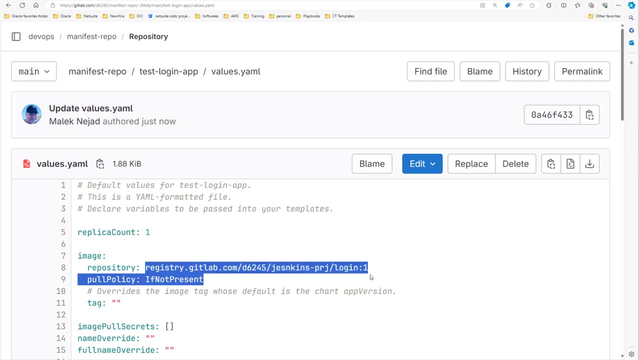 so here this is my helm chart. if i click here here you see all the file related to helm chart. let's click on value and in image repository you will see this one. okay, so we need to update this one to the latest one by jenkins pipeline. so how we can do it. 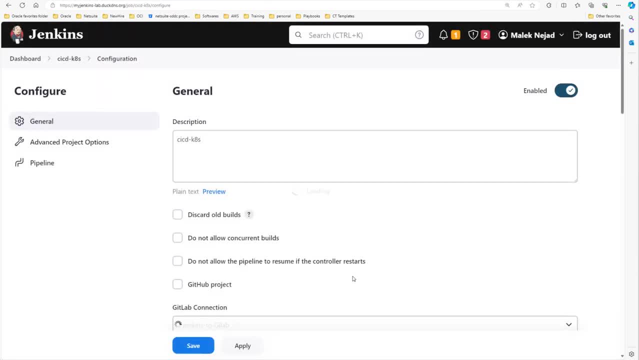 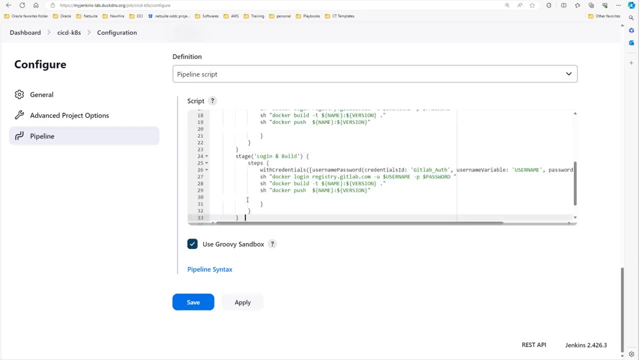 in jenkins. if i back here, we have to add another step, so let's copy this one, paste it here. let's change the name to update tag and let's remove everything that we have here and be ready to update tag. how we can do it? at first we have to pull manifest report. 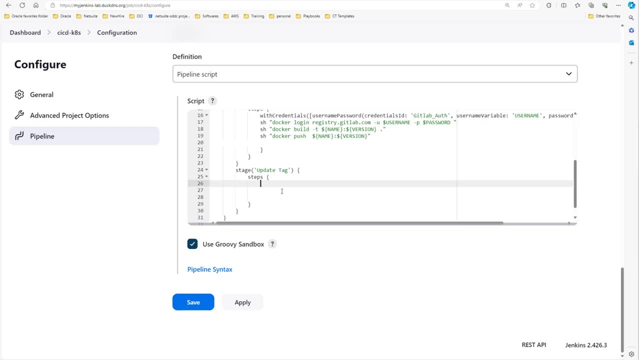 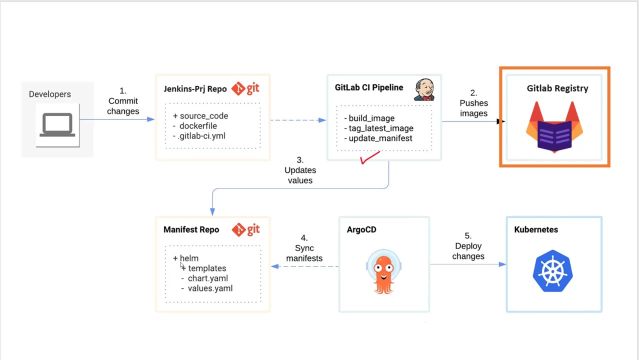 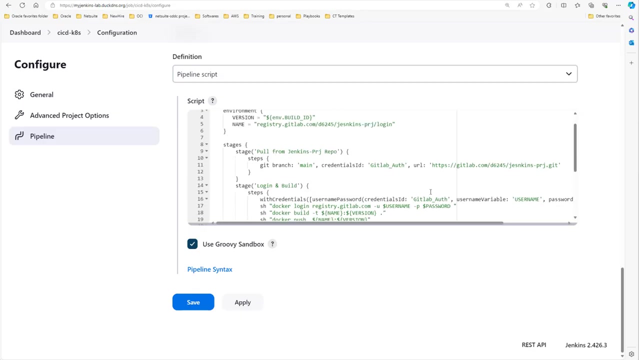 first we have to pull manifest report. first we have to pull manifest report here. here is my jenkins and we have to pull this repo here. as you remember, we did here for jenkins dash prj repo. we are going to do the same for this repository. just paste it here, it will go. 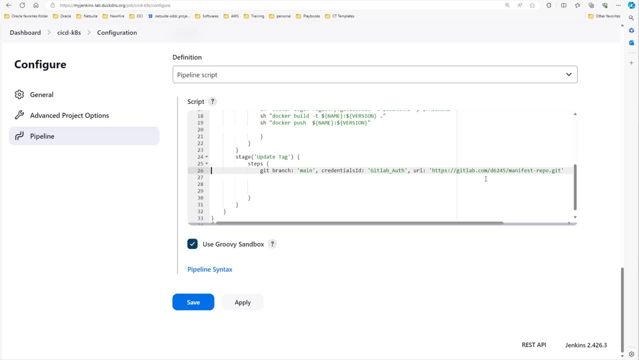 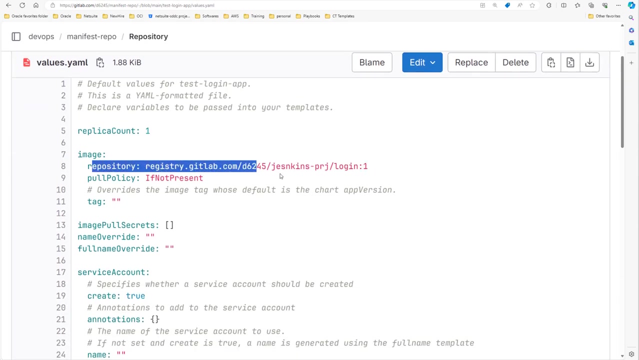 and pull manifest repository here. okay, after pull it, what it should do. okay, let's add a tag here with a starting or updating image tag and how we can do it should go and open this file and find this line and replace it. how we can do it. it's easy with said. 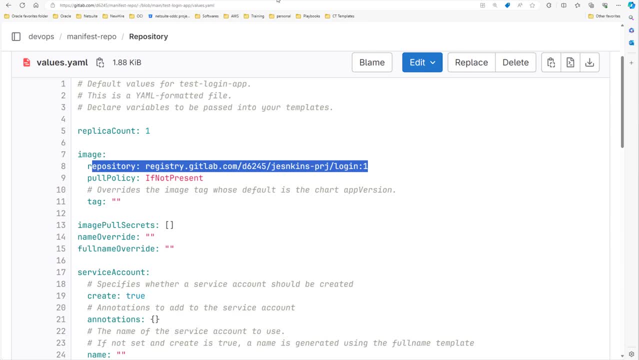 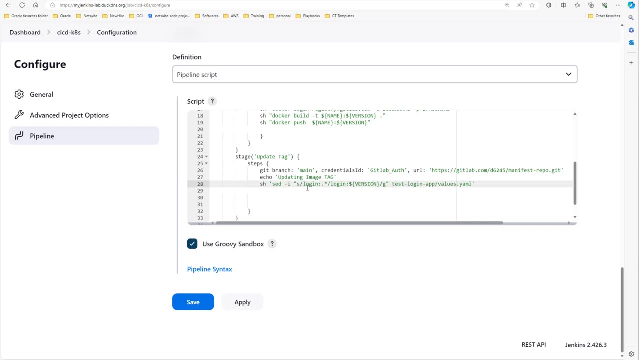 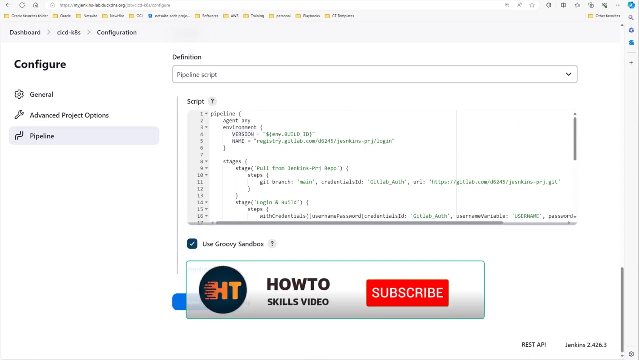 or another command in linux you can do it. so here i'm using this command. said it will go where inside helm chart value dot yaml file and will go and find login with any version and we change it to the new version. new version- what is that? it's a build. 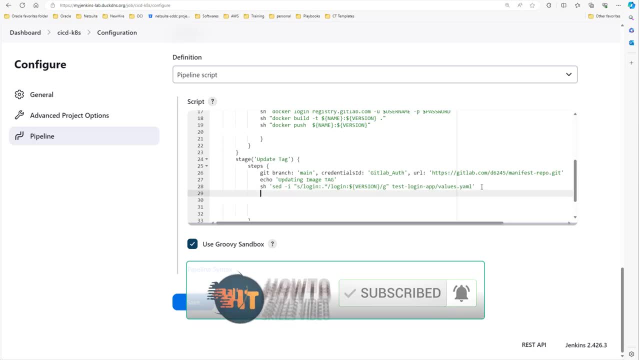 number. good so far, so good. okay, after that, what it has to do it should be push it back there to manifest ripple, and it means update repository. but before that we have to config git for it what it means when you want to push a change to a repository, you have to config. 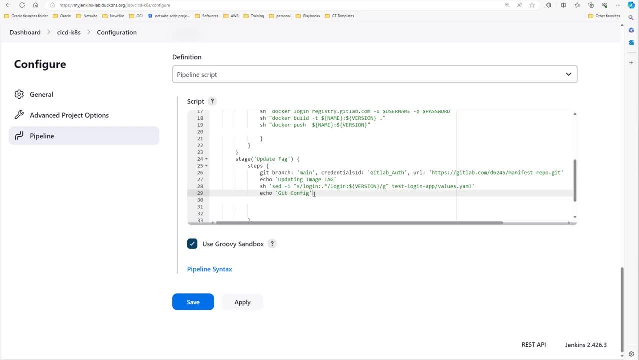 git on your computer. you have to define your email, you have to define, you go to email, you have to go to states and you have to then emmiam5 to ya 당시press or ya in theتمain, you have to define your link and so on to ipn that being state, and your website is going to be the ditch andациnnื่. 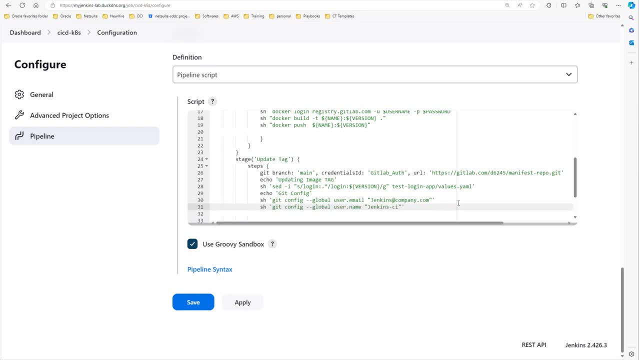 your name, who, who are you who want to do this push? because when we review all the commits, all the changes, we should know who did this one. so we define like this, and then now it's time to to add changes. you can do git, add dot or a specific file, that we change it and then commit. 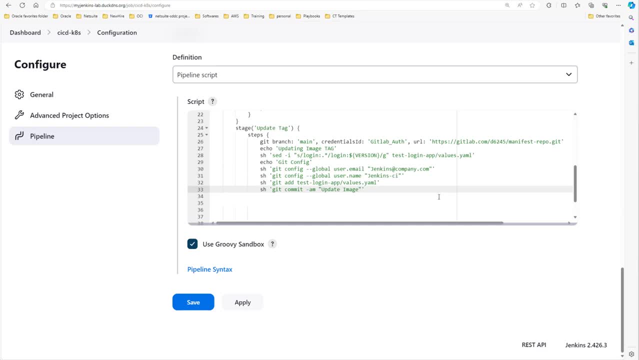 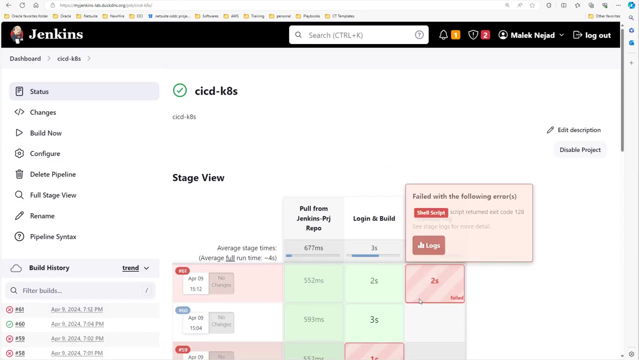 changes, update image tag, for example. and then we have to push it. okay, let's type sh like this: one double quotation or one quotation, no problem, git push. let's save it and run the build 61. look, here we got a failed. let's go in and see. 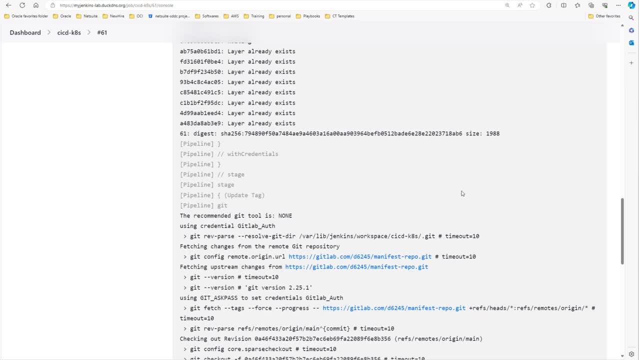 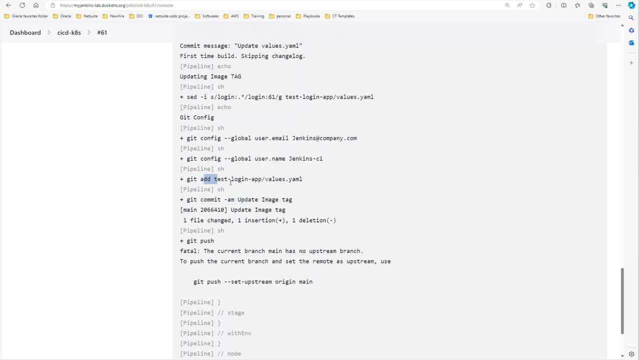 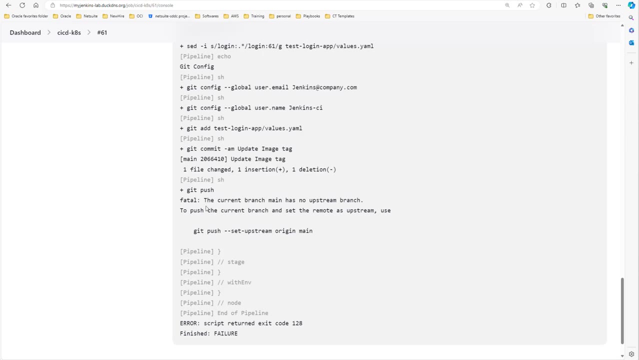 what's the reason? let's going down. okay, build is okay. look here, update, updated. look here also: git add, git commit, git push. okay, we got an issue on git push. as it show it here, the current branch main has no upstream branch you have to use like this one, okay. 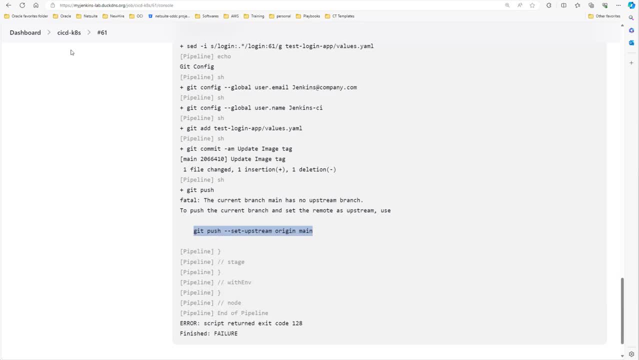 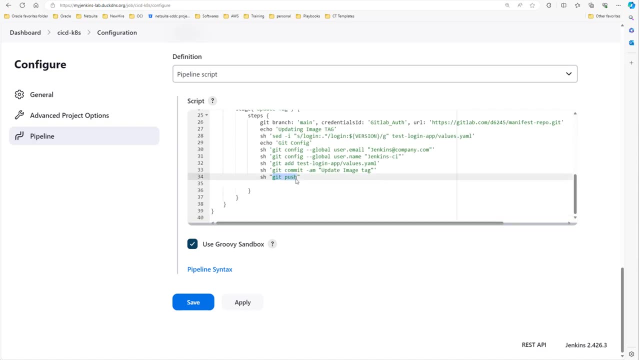 let's copy this one and back to configuration- configure, going down as it is written. we replace it here. let's see if it is work, and i'm sure it will not work. just i want to show you what's the issue: save and build. let's click it here, as i told you, it's. 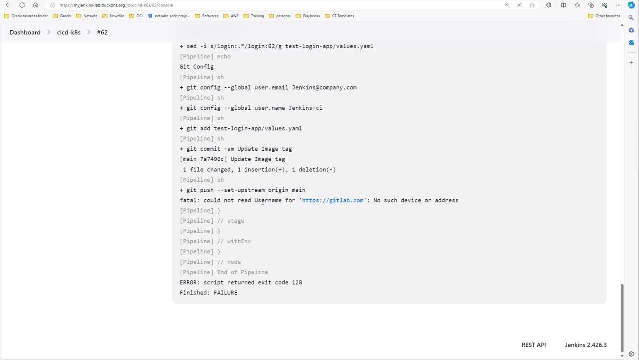 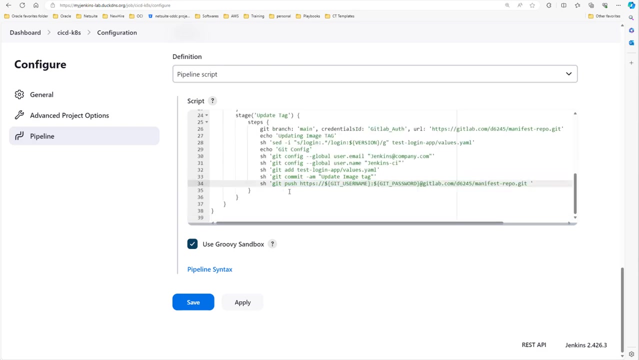 look here could not read username for gitlabcom. here we found out what's the problem: need username. when you want to push to gitlab, you need username and password. so let's go in here in configuration and solve this one. at first it should be like this: git push repository address with username and password. so from where we have to. 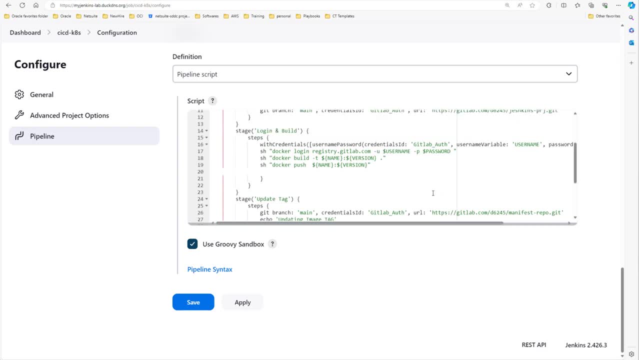 get this username and password. if you remember from the build, we use this one with credentials, so let's copy this one and add it at the first line here. if you see at the end has an acroлоad: http//githubcom. ok, you have to keep the". 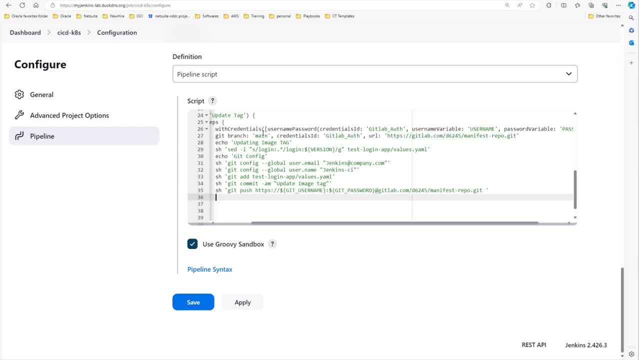 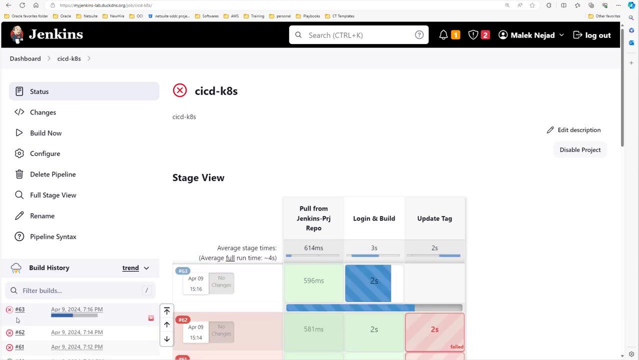 close this upload. so at the end and close the upload. and here you see we have username and password. so it is better to update with this one and for the password. so far, so good. let's save it and build it. let's see if it will go successfully. let's see what's the problem. okay. 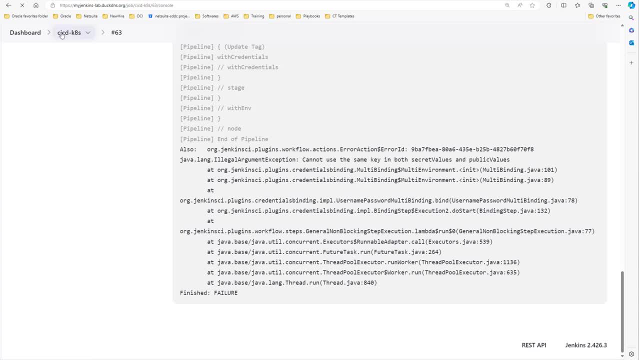 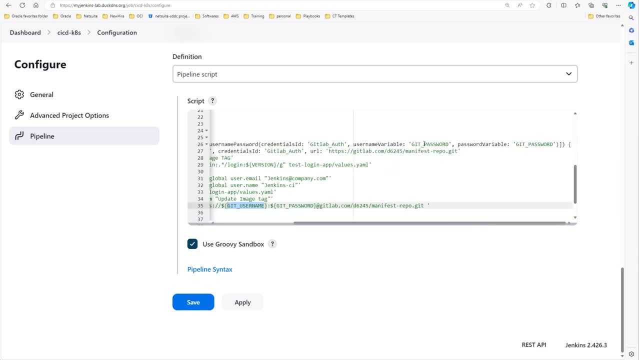 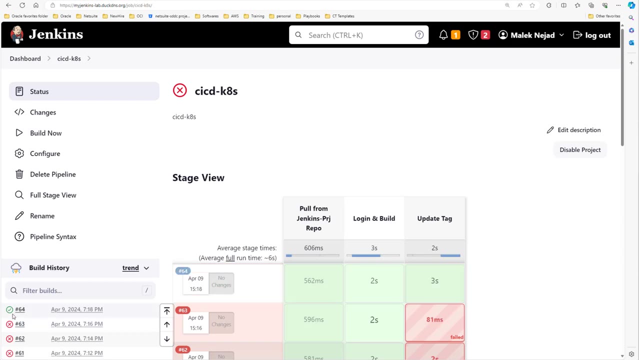 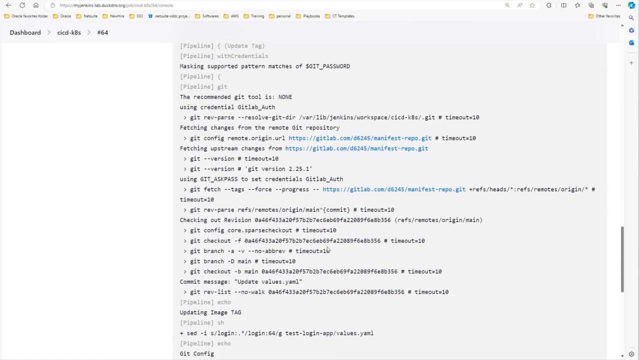 with this error. it means a typo. let's back here: configure with credential username. at first i did a mistake here. i have to update the git username password. okay, let's save it. build good. so i the moment run successfully, click here and going down and see: yes, everything done at. 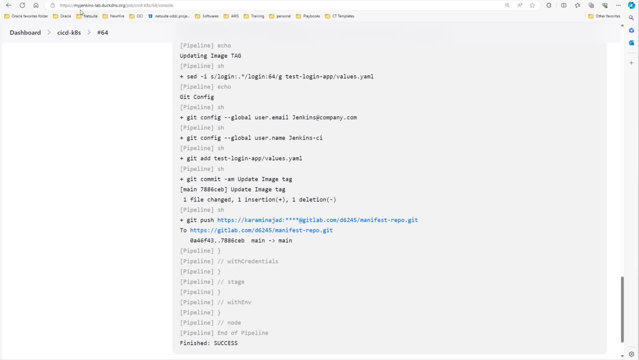 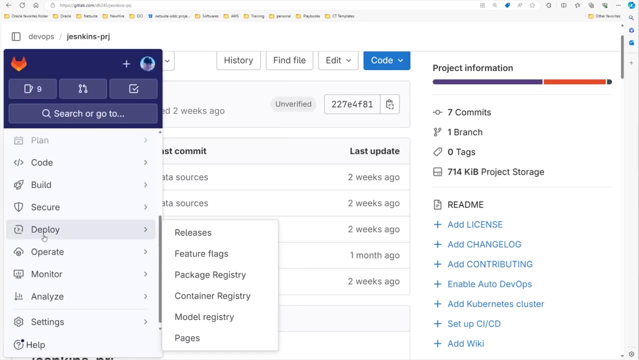 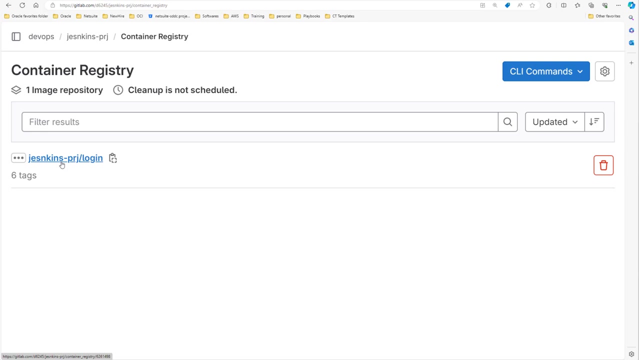 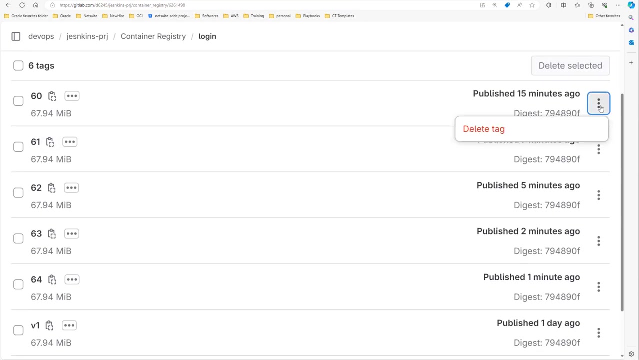 first let's see this one: 64 back to gitlab repository, to jenkins prj from the left side. deploy container registry six tag, because every time we did run a new tag added here the latest one that we got successfully, so we don't need the other one at the moment. let's. 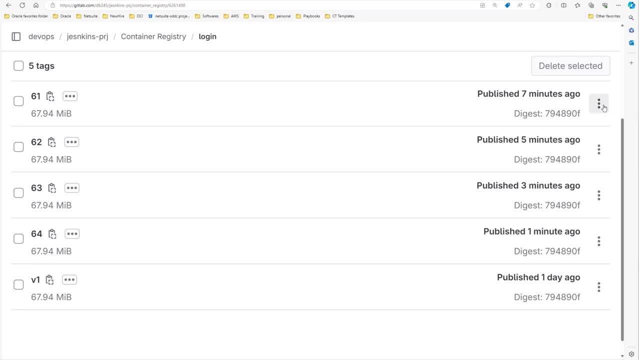 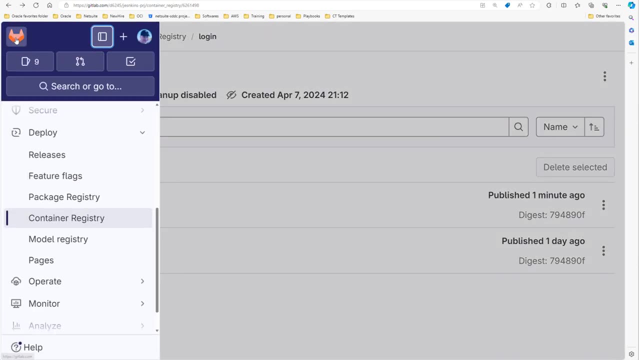 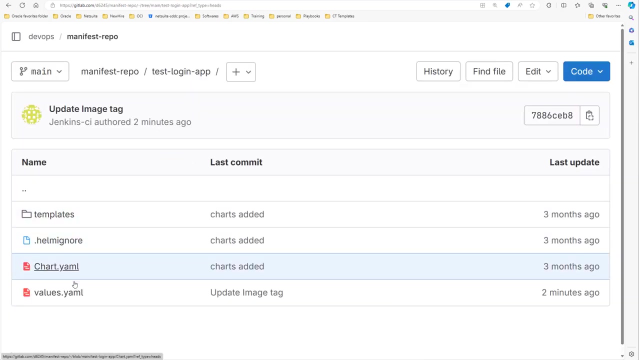 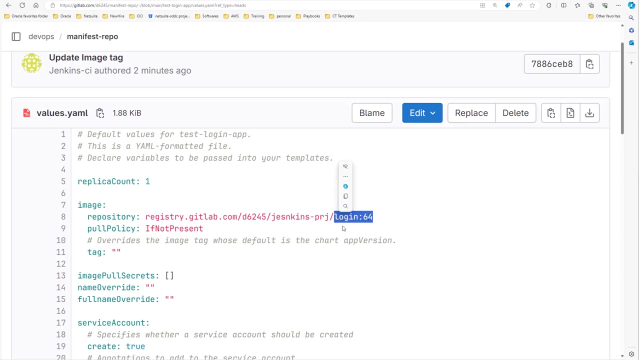 clean this one to prevent any lake of capacity. let's remove this one also and let's back to other repository- manifest repository- and click on helm chart on value and look here the latest tag updated here. so far, so good. just for quick Argo CD installation on Kubernetes. 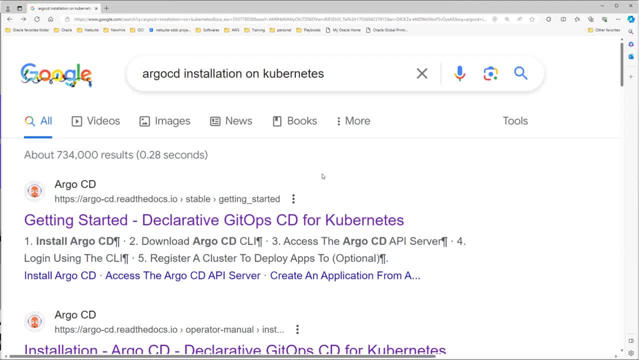 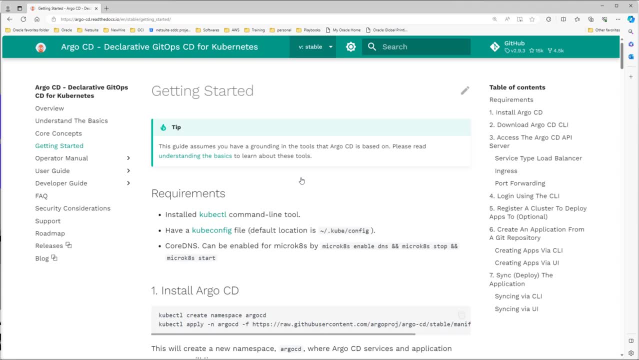 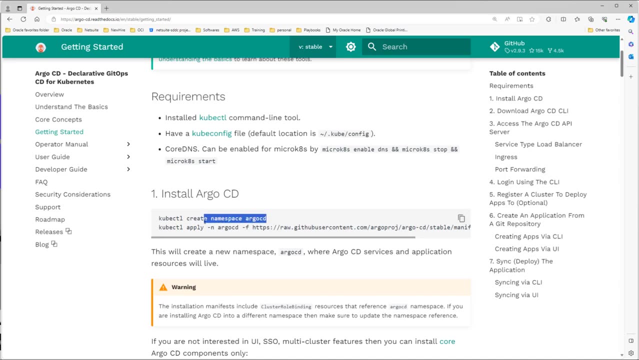 type this title on google and from the result click on the first one. so here is the official website of argo cd and here you will see: install argo cd. just there are two commands. the first one, it will create a name space. it's called install организational senorand. just click on the link. 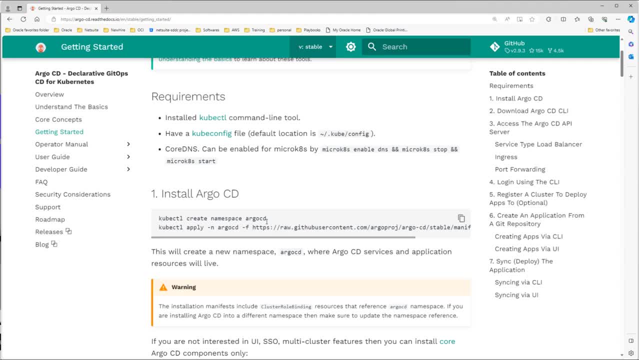 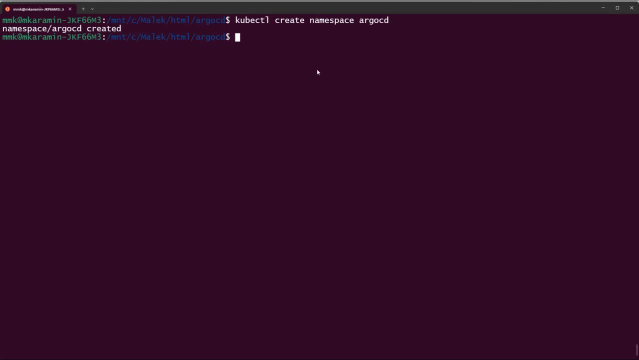 and after the امول object type, the second one- and as you can see it will create a name space- will argo cd, and the second one in this namespace will install argo cd. so let's copy the first one back to terminal and paste it here. okay, argo cd namespace has been created. let's go in and copy. 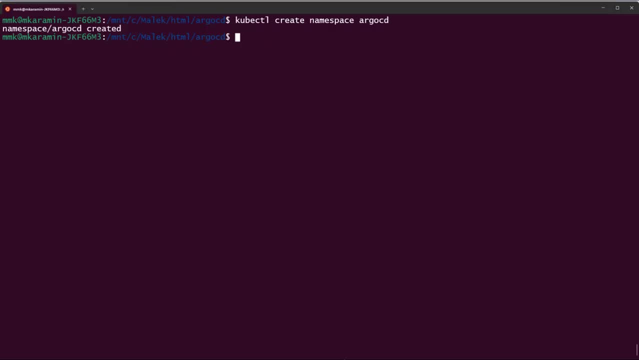 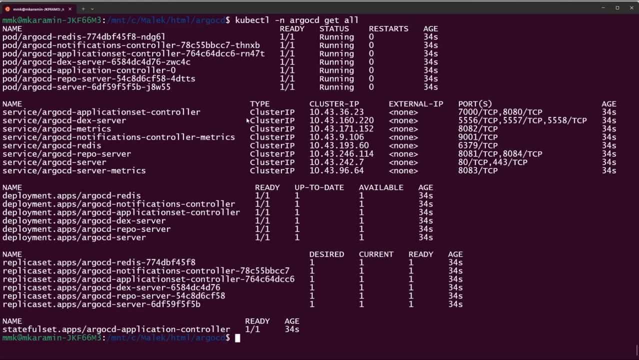 the next command, copy and paste it in terminal. okay, it's done. let's type kubectl dash in argo cd, the namespace, and get all all the object related to argo cd have been installed and in running status. look here, there are some pods related to that. they are: 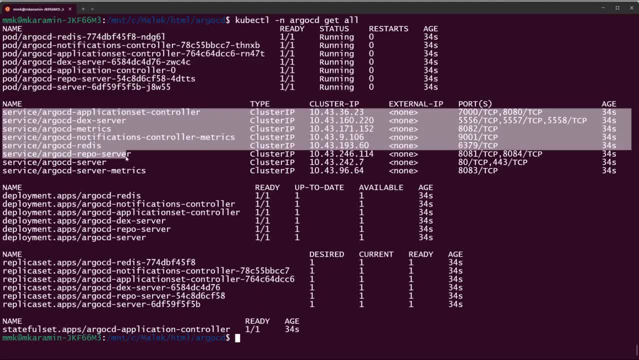 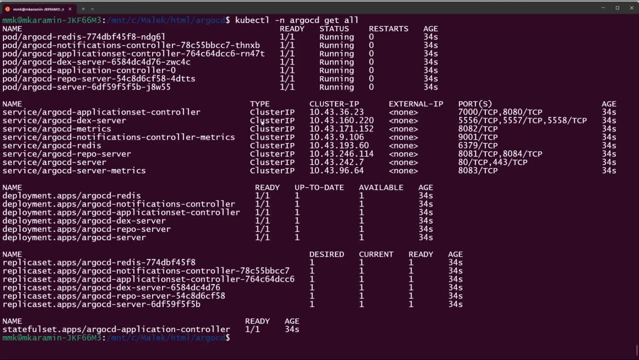 installed and in running status. look here there are some pods related to that. they are installed and in running status. look here there are some pods related to that. they are running status. also, services deployment and replica set as you see all the services exposed as the cluster IP here. so for access to our go CD web UI from: 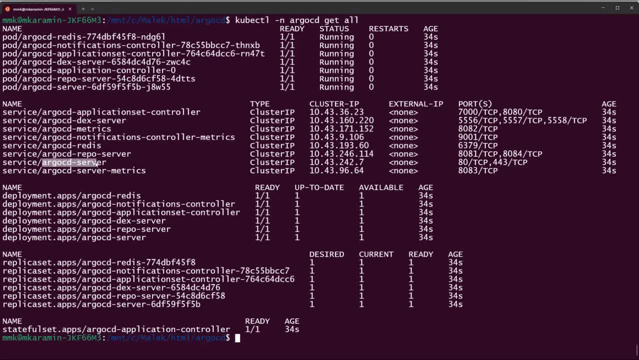 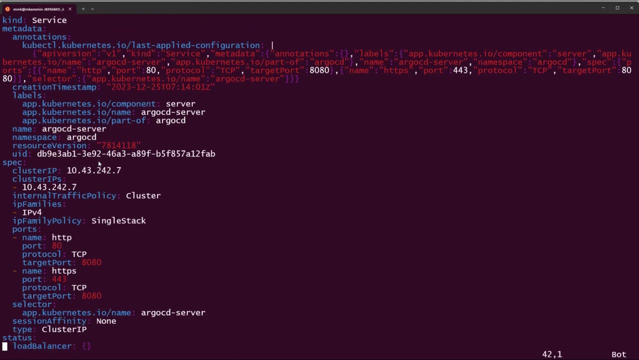 the external we need to expose our go CD server as not port or load balancer. but here I'm going to change this cluster IP to loop port. how do that just type cube CTL dash in our go CD edit service, our go CD server, and going down and change. 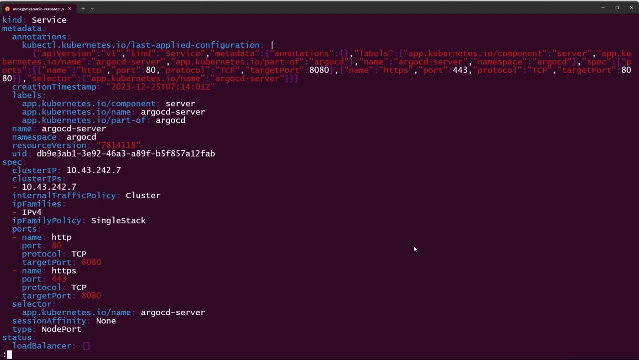 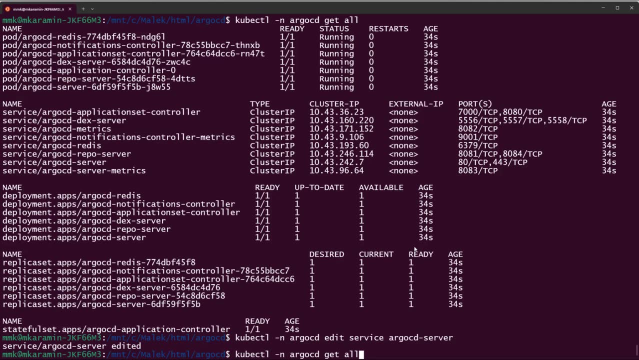 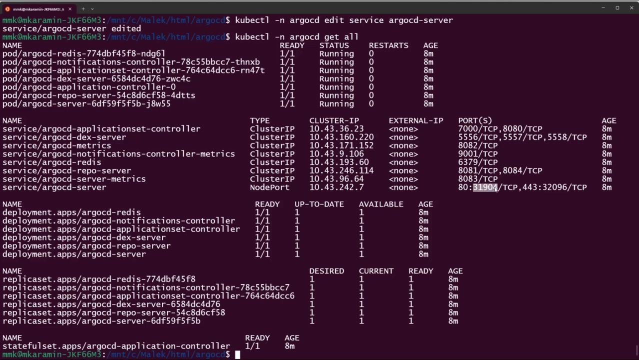 the type to node port. just save it and exit- it's edited. if I run again, cube CTL dash in our go CD, get all you will see it changed. all you will see it changed. all you will see it changed to node port and automatically got this port so we can access it from outside of kubernetes cluster. 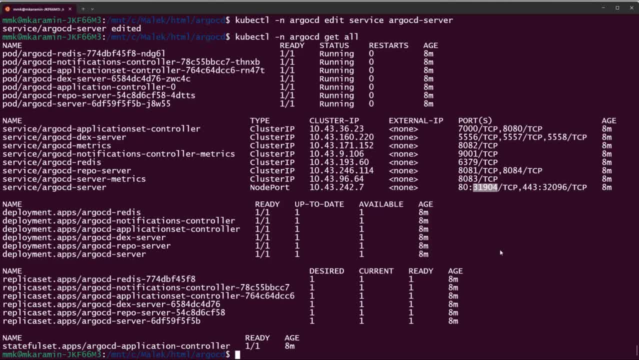 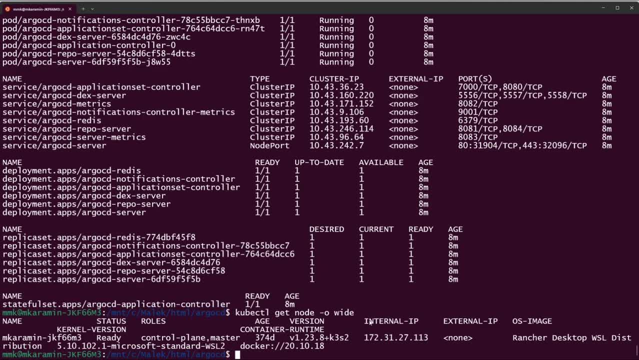 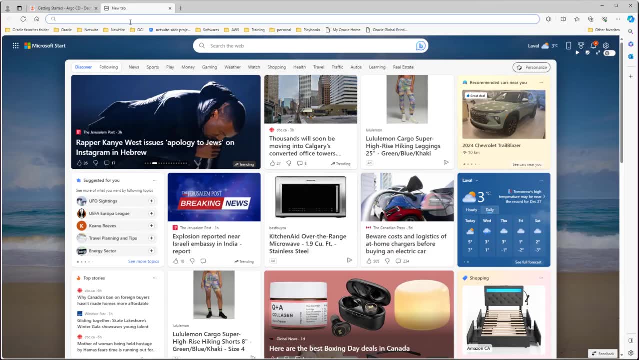 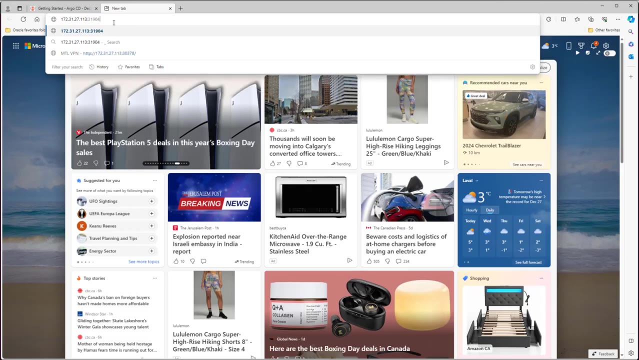 okay, let's find the ip address of kubernetes, node tube ctl. get node dash all wide and this is the ip address of the node. let's grab this ip going to browser, paste it here. let's get the port. take this port and back to browser and paste it here. look here, advance continue and here is the argo cd. 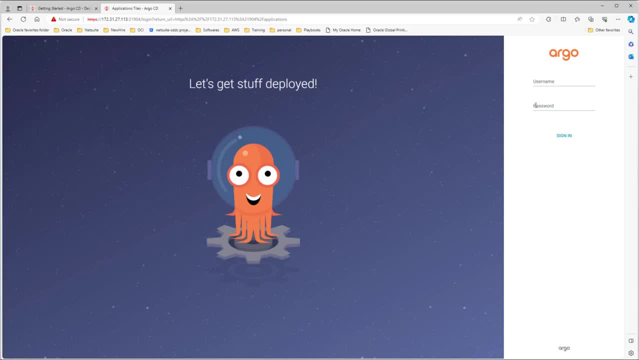 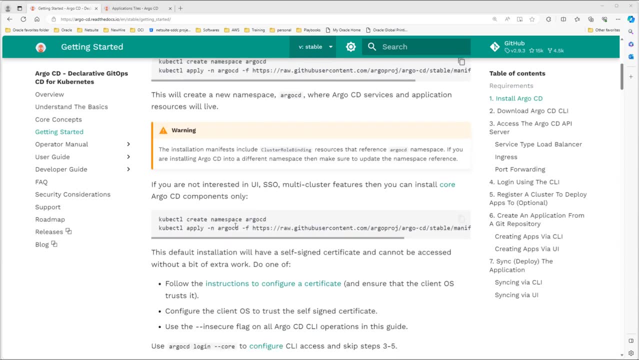 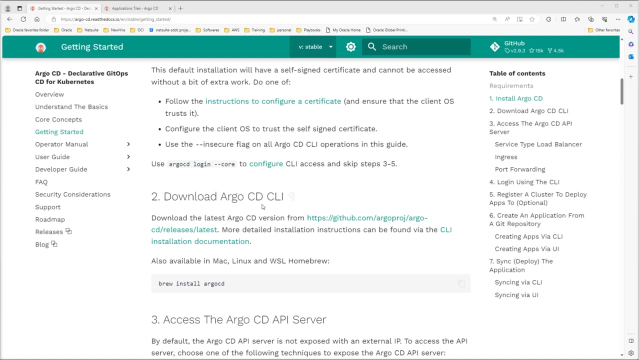 web ui for credential. let's back to argo cd official website and here, after install that, let's going down and you will see download argo cd cli. so we need to install argo cd cli. then we can retrieve the admin password to connect argo cd web ui as it is mentioned here. 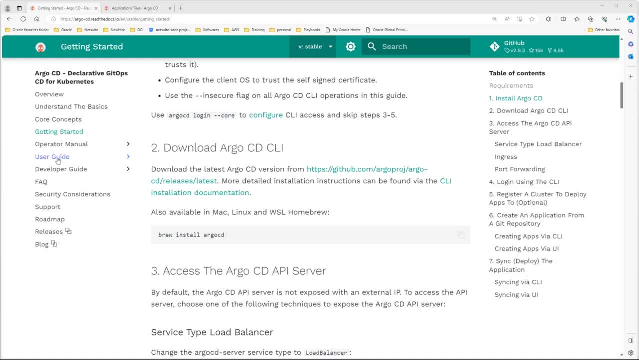 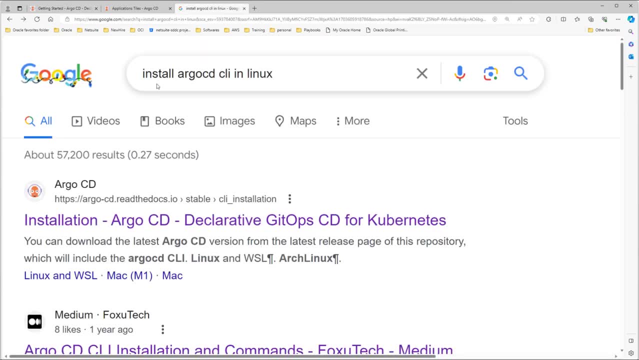 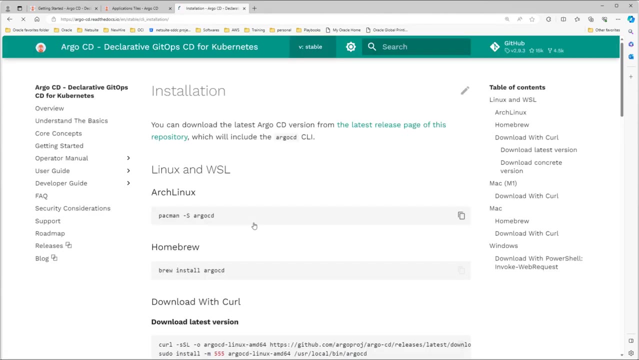 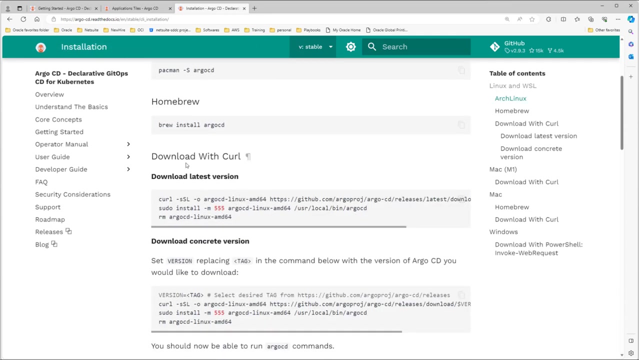 also available in different operating system. how to do that, here there is a documentation about it. but if going to google and quickly type install argo cd cli in linux and from the result click on the first one, here you see the installation on different operating system. let's go in here and using download with curl, so copy this one back to. 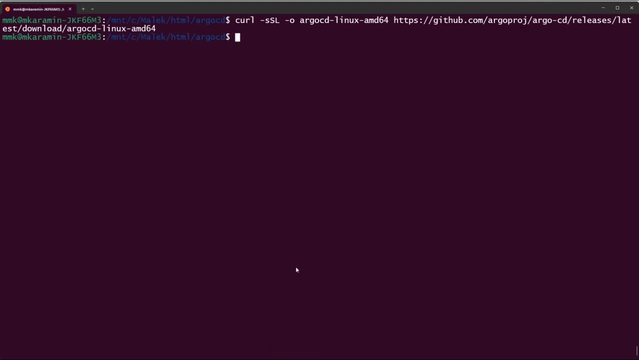 terminal. okay, it's done. ls here you see, it is downloaded. so let's let's back to argo cd website and copy the second command back here, paste it here installed and let's grab the last one and move the downloaded file. okay, good, let's back to official document. this one is downloaded and 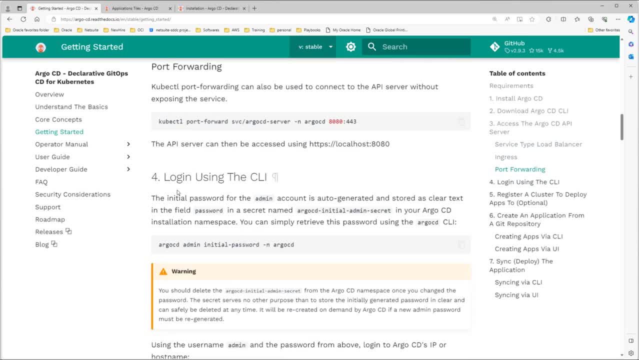 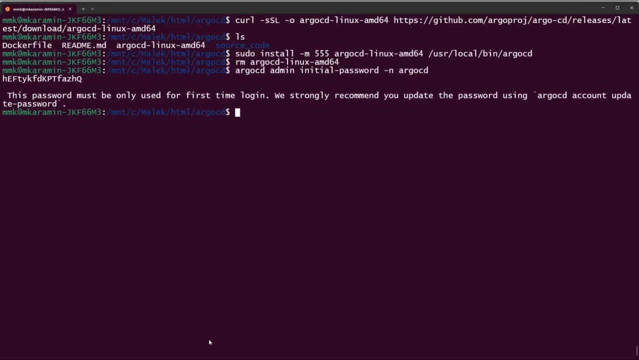 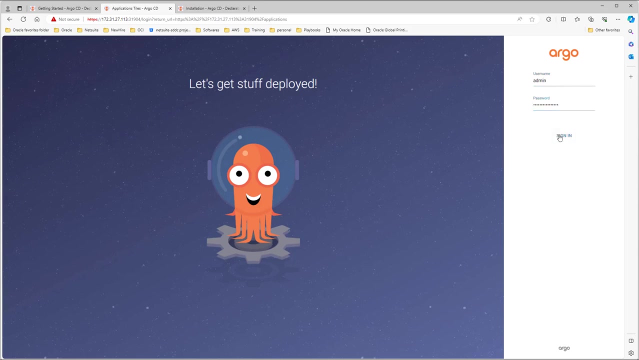 installed. just let's going down and here you see login using the cli. let's grab this command to get the initial password for the admin account. here is the password for the admin account. just copy this one back to argo cd web ui, type admin and password and sign in. here you are. this is argo cd web ui. it has been installed. 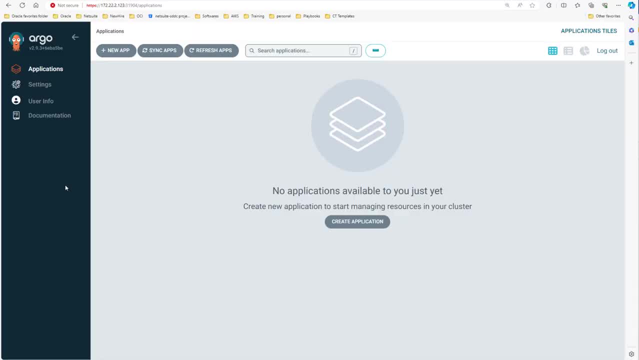 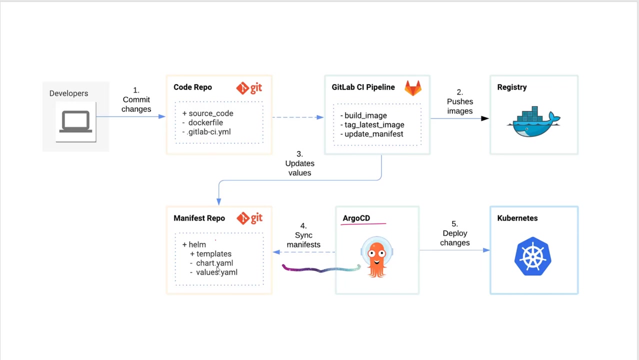 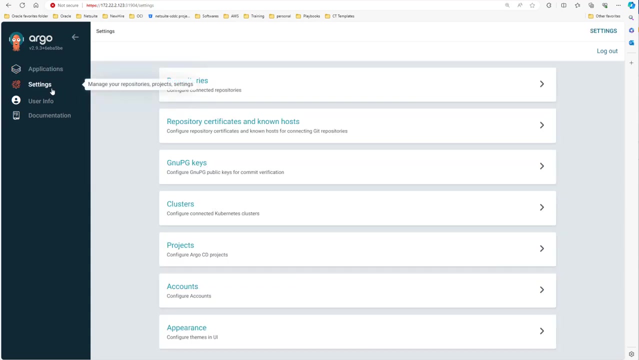 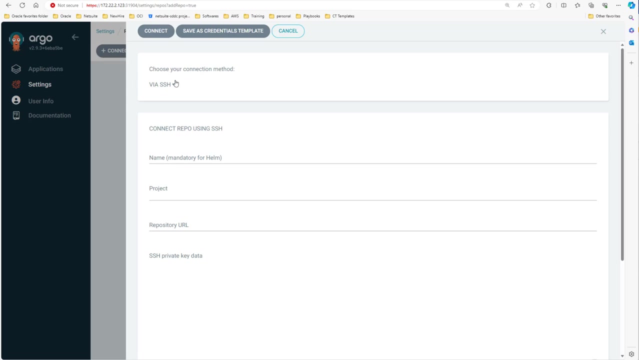 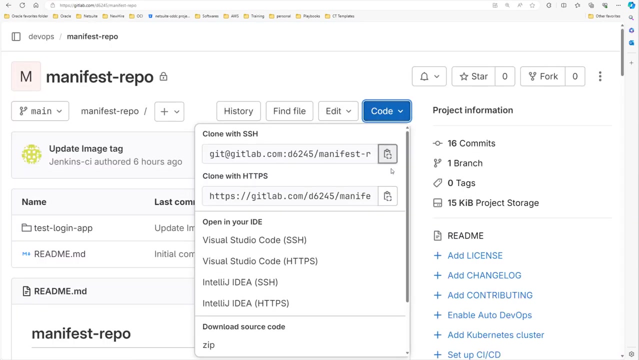 and ready to use in project. okay, now let's connect argo cd to manifest repo. make connection between argo cd and manifest repo- the left side going to setting click on repositories- and connect repository via https type git project default repository url. let's copy it from the gitlab manifest repo code. 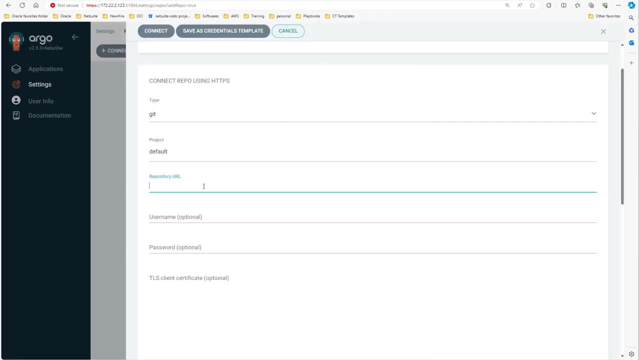 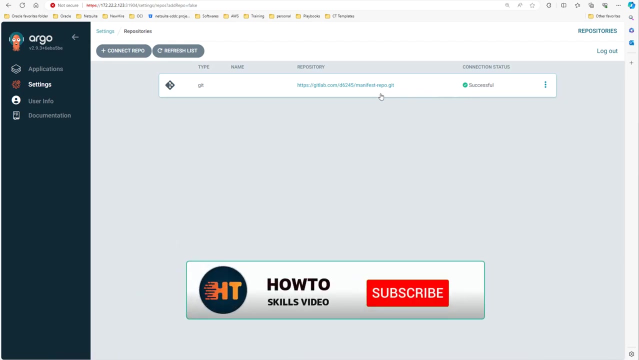 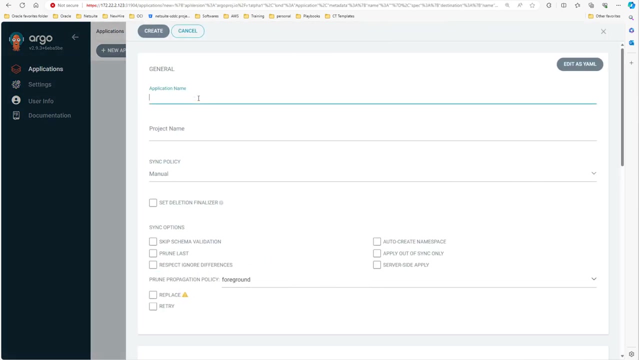 grab it back to argo cd, paste it here. username: because this repository is private, we need to enter username and password and connect successfully connected to manifest repository. now let's back to application: new application. give it a name. it should be in lower case, for example, login page. project name: default. 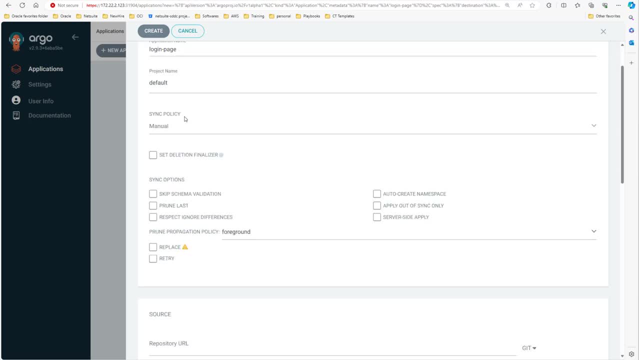 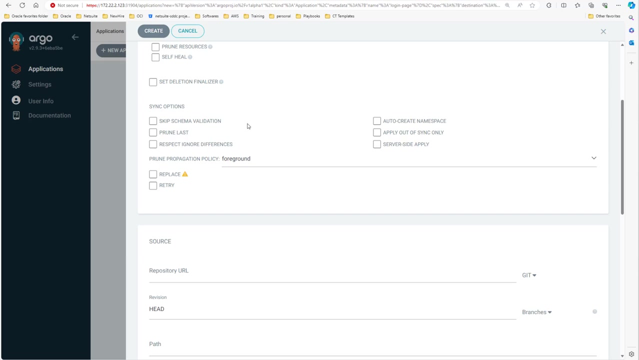 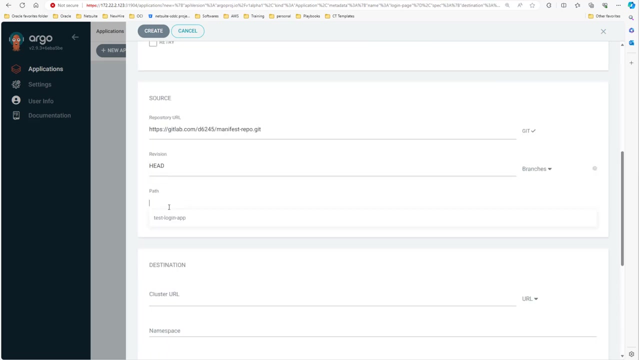 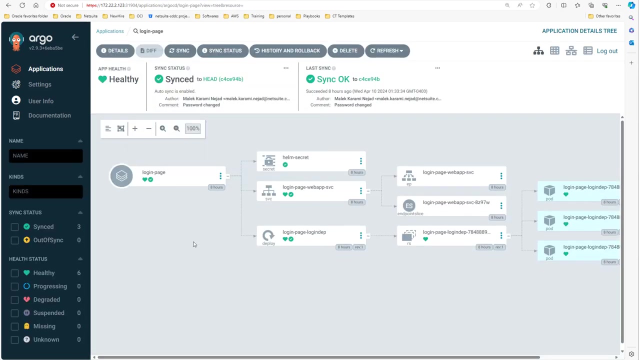 as we selected in repository for sync policy. change it to automatic so every change happened in repository. automatically will deploy on kubernetes cluster. so, going down for the repository url, select this one: revision head and path. show you the helm chart folder. so select this one. and going down, cluster una fault and carry it. let's click on this box and 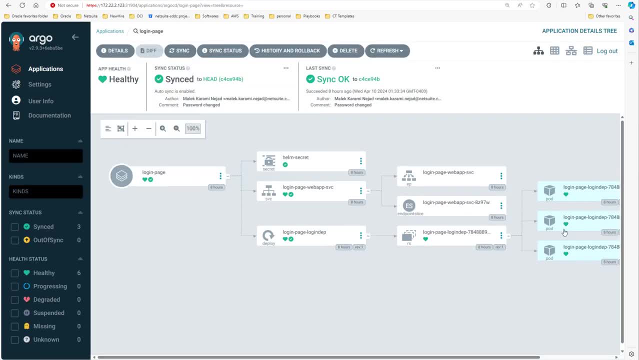 you see application deployed on kubernetes cluster in or helm chart. we have a secret. we have a speakingValue我们有主要广告我们有证明 hatch. we have a secret service and a deployment. look here deployment: successfully and healthy deployed three pod on kubernetes cluster. let's go into terminal and verify that. here is my terminal: cube ctl. 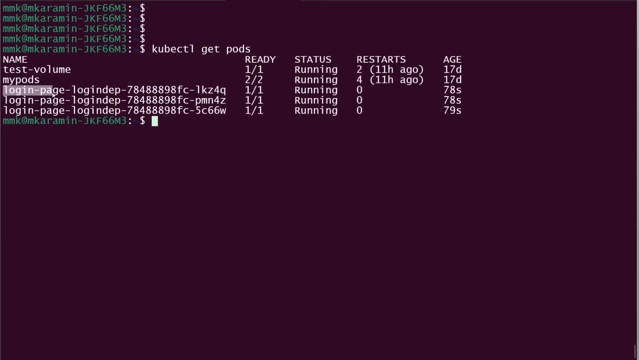 get pods. look here, three pods with the name login page. if you remember, in argo cd we use this name for our application. let's cube ctl get, as we see, login page web application. look to the service. it is not port and this is the port that we can reach. it on browser type: cube ctl get notes, dash. 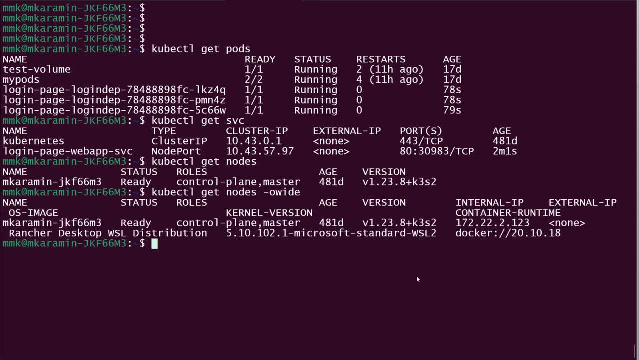 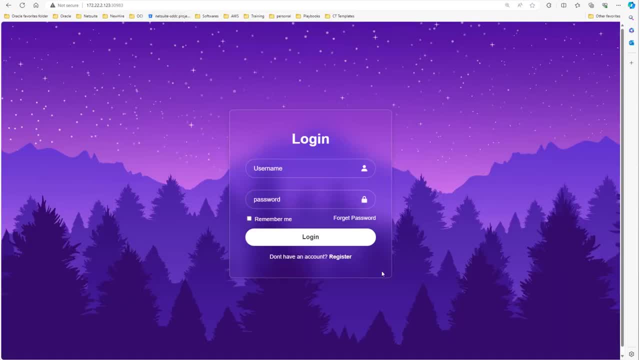 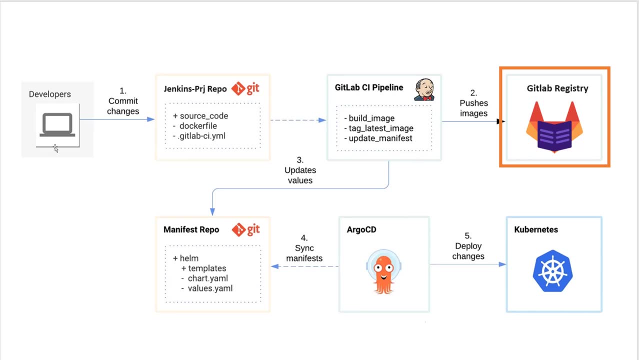 or wide. take this ip back to browser and port this port. look here, this is the login page. now let's do another test. at first we do a change on source code and push it to jenkins prj repository. then it will trigger jenkins pipeline by webhook. will. 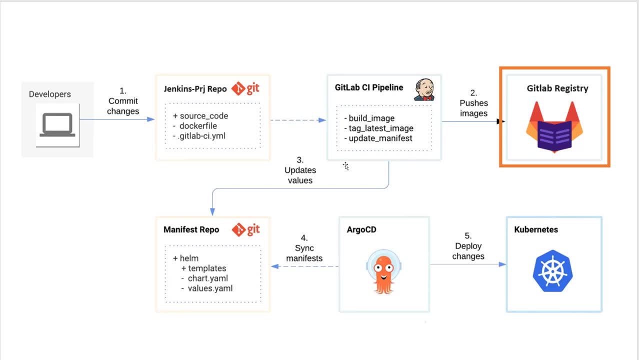 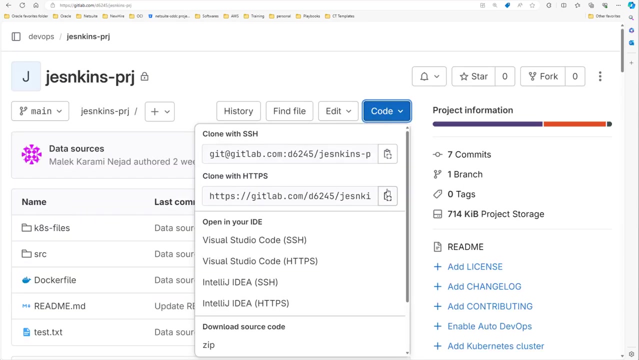 build an image, push it to gitlab repository. then we'll update tag on manifest repo and will sync argo cd and argo cd will update application on kubernetes cluster. let's do a test at first. let's going to jenkins prj. take the link back to terminal. 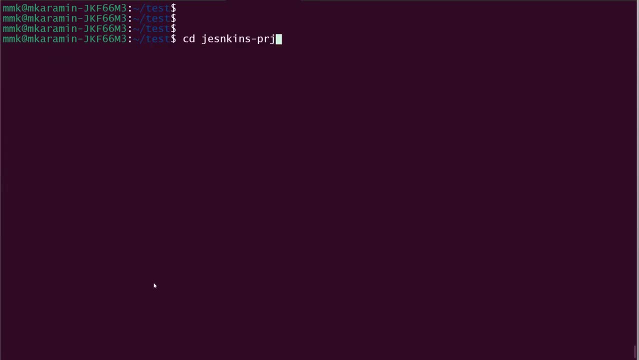 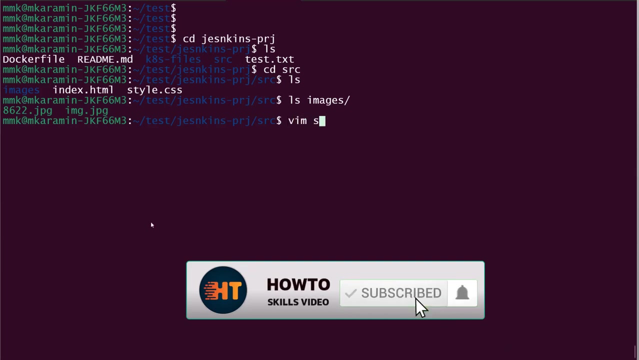 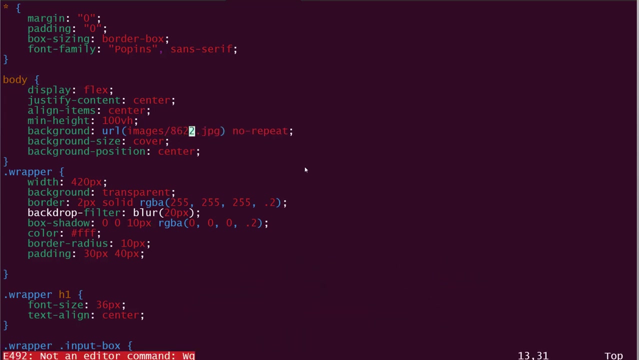 git clone this one cd jenkins and ls going to src. and let's ls image. have these two image. let's copy this name and vim style. at the moment we are using this one. let's replace with new name. save it. git status. git add. git commit. add a message. 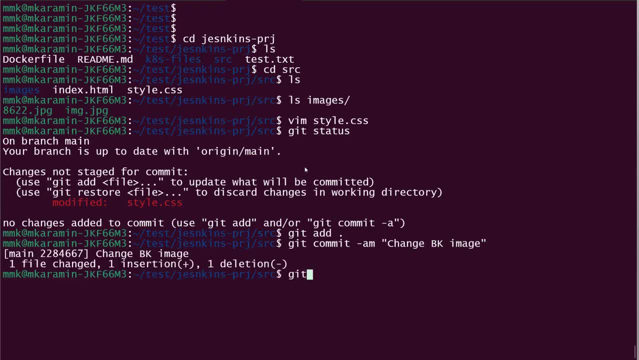 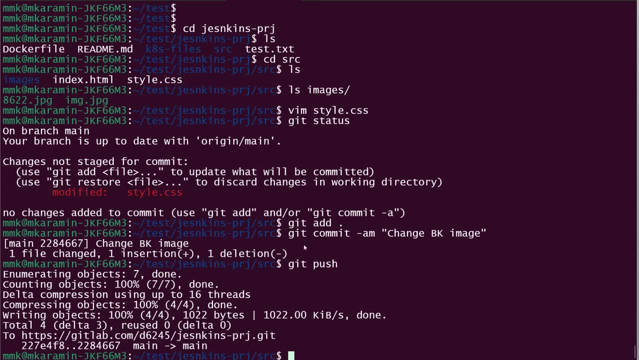 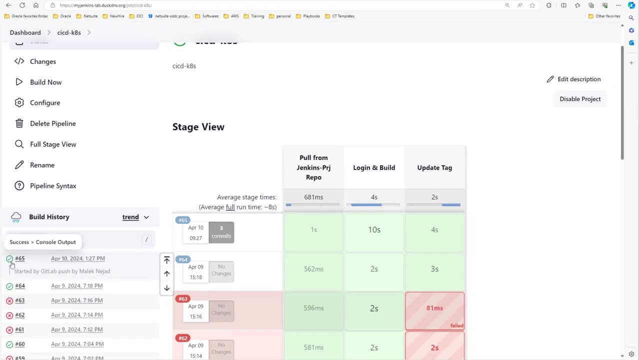 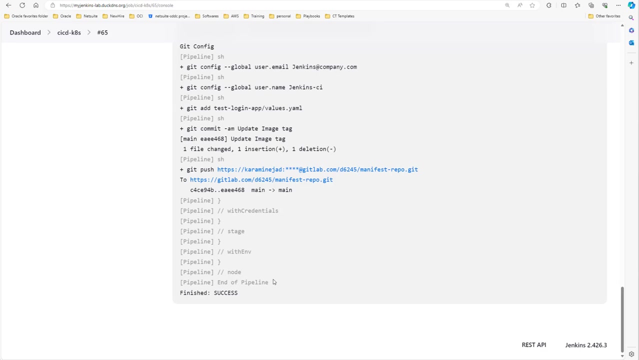 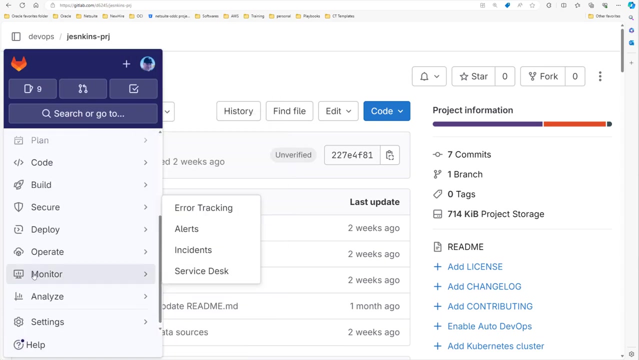 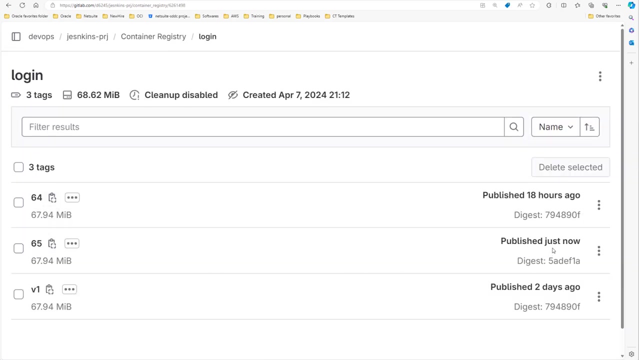 change background image and git push. so we push the change to jenkins dash prj repository. let's back to jenkins. this one- look here. 65- started by gitlab push. everything done successfully, let's going to gitlab and from the left side, going to deploy container registry. click here. look here. 65 just some seconds ago. 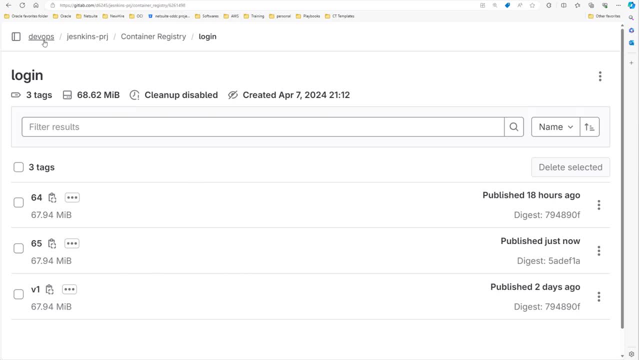 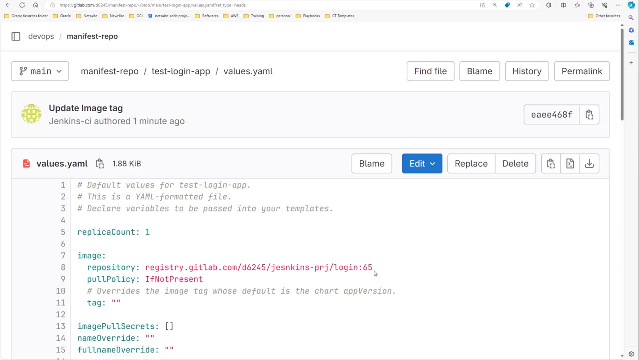 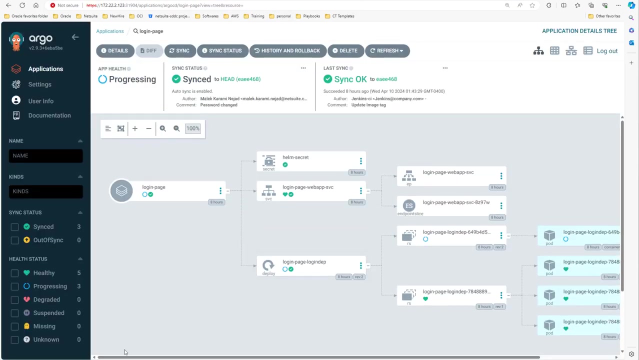 it's updated to 65.. now let's go into another repository, manifest repo. click on helm chart value. look here, it updated to 65. and let's back to argo cd. look here in argo cd, revision 2.. before it was revision 1, with the old background image. 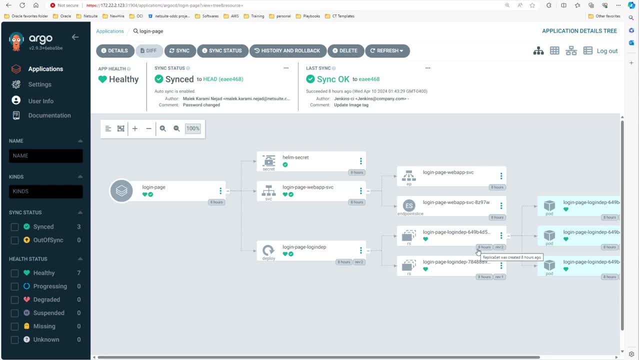 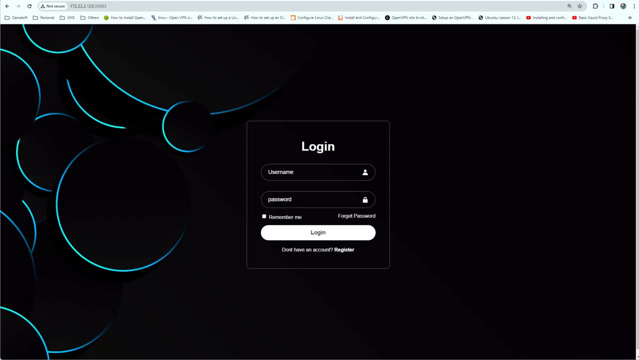 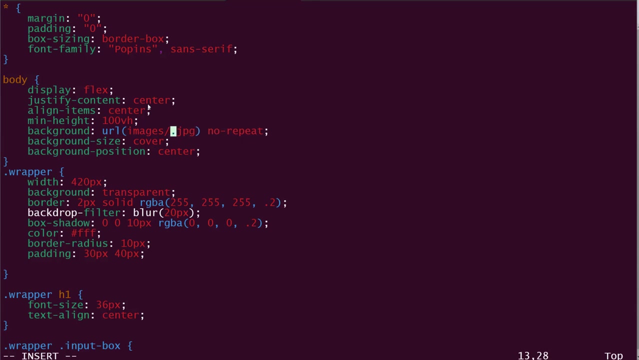 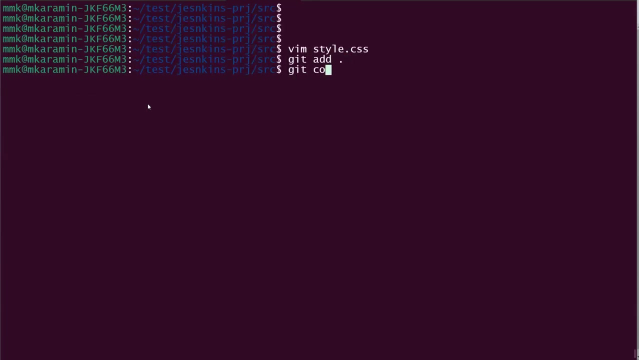 now everything updated and new revision created by helm and the parts updated with the new one. if i go here and refresh, and here the login page with new background, let's revert changes. img was the old name. let's save it. git add, git, commit, dash am river back. revert background and git. 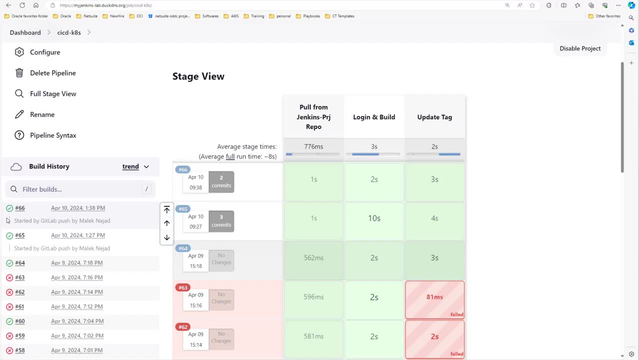 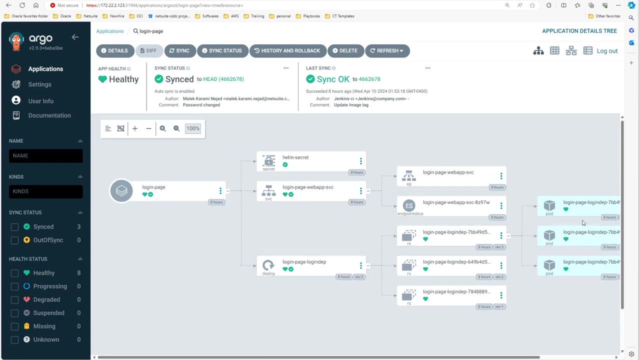 push. let's quickly back to argo cd. look here in jenkins 66 was created, so updated tag on manifest repo: look here. revision 3 is creating and the old parts deleted. new parts are: детейdallee, alexisaBI, child engineerus-team paul.